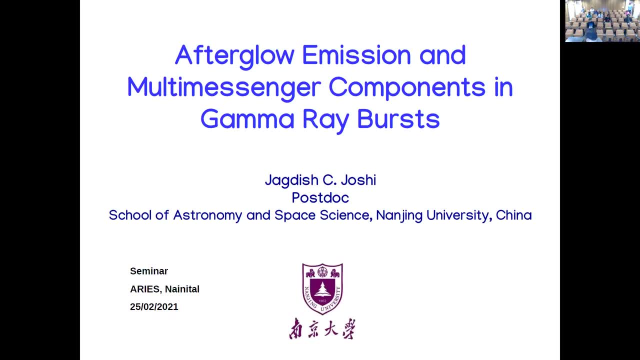 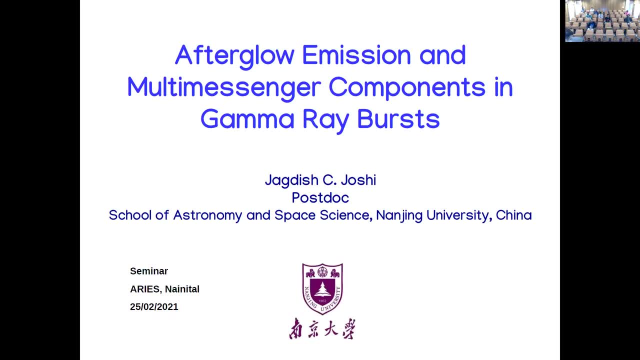 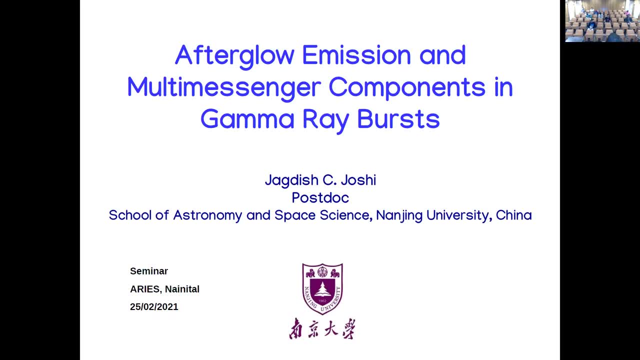 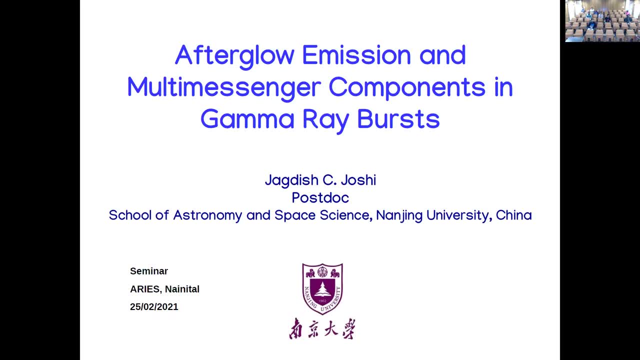 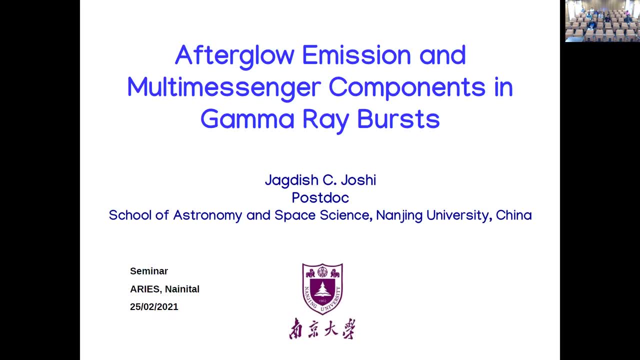 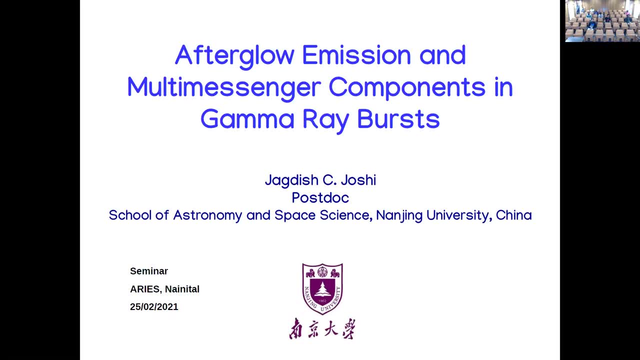 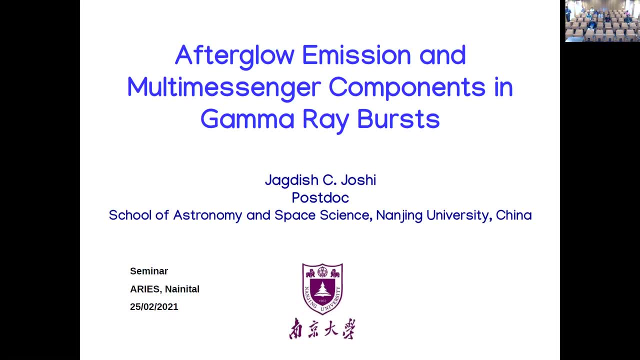 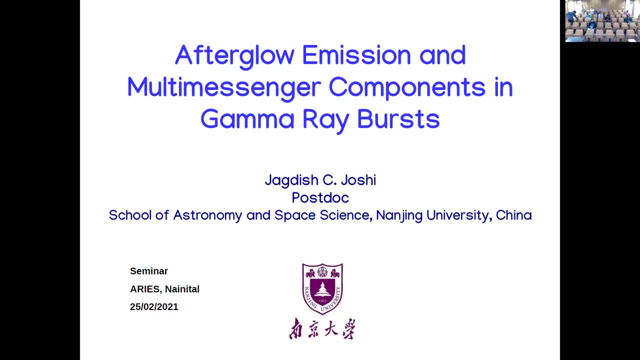 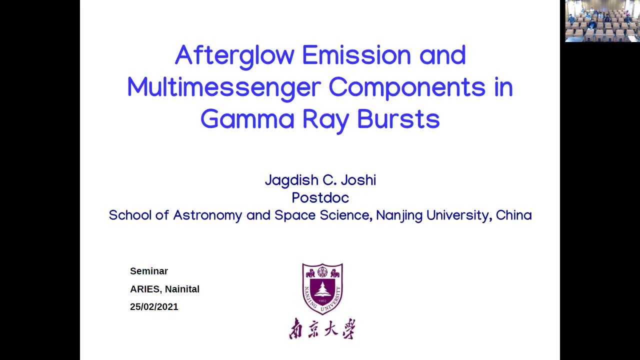 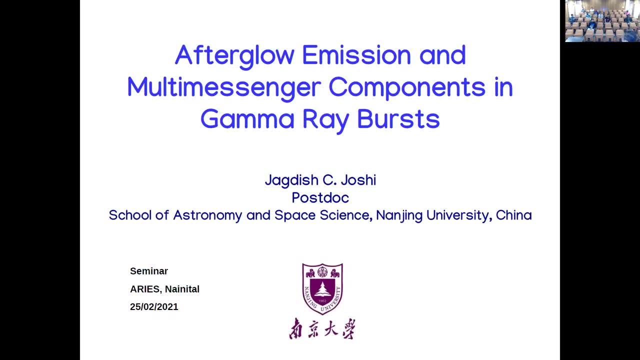 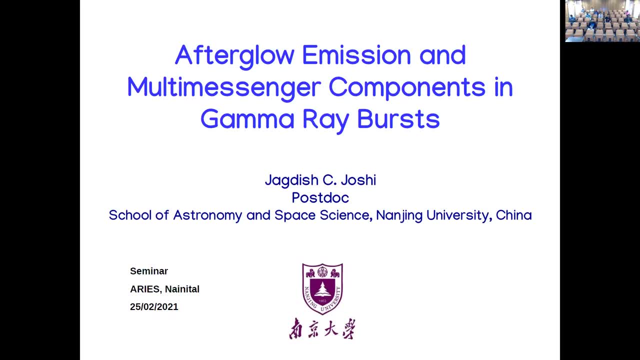 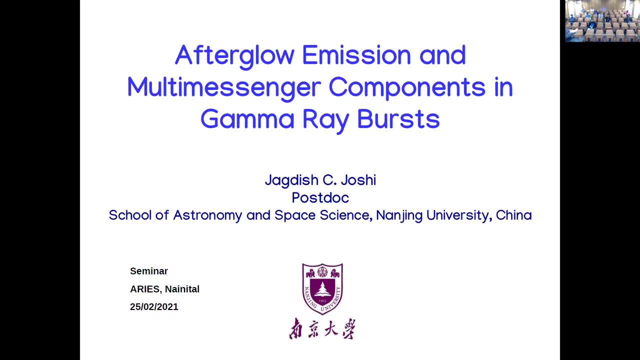 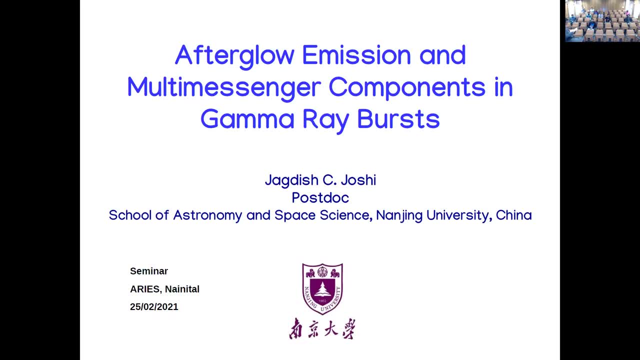 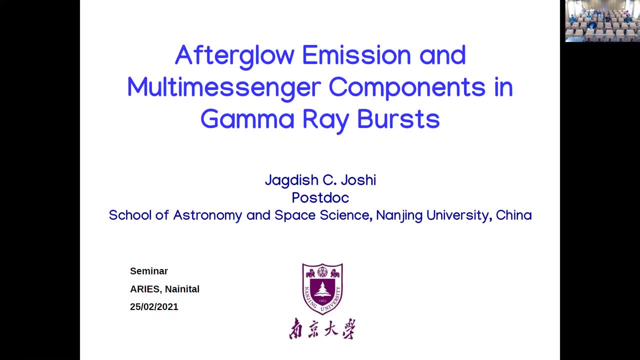 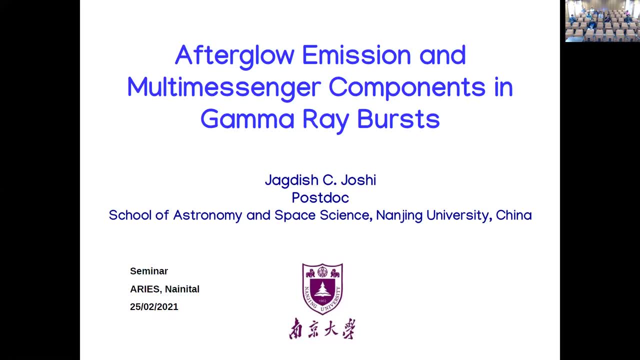 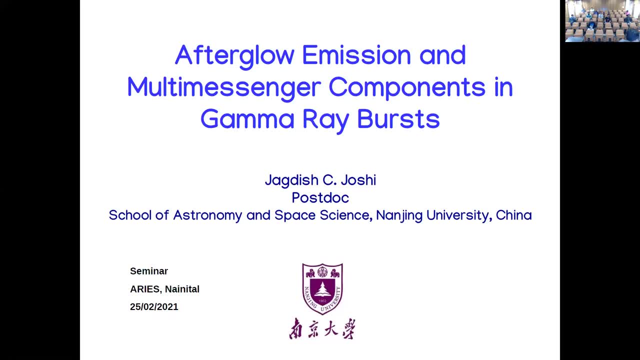 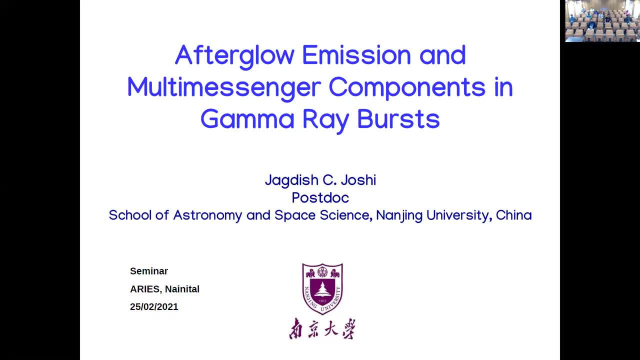 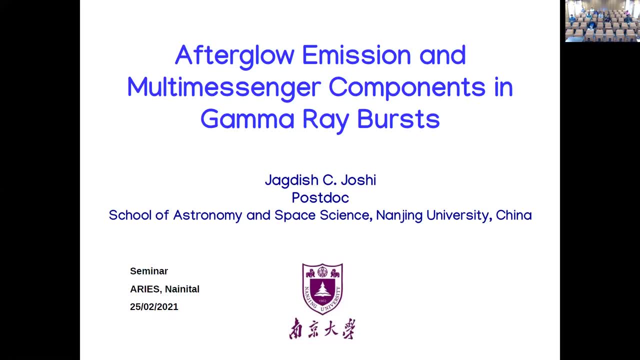 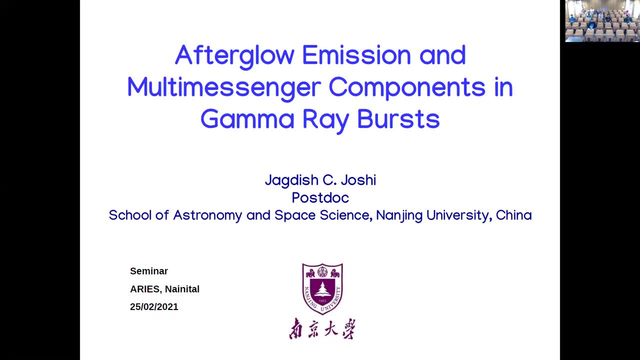 So good afternoon everybody and participants available here as well as online. So good afternoon everybody and participants available here as well as online. So good afternoon everybody, and participants available here as well as online. let us discuss what we can do jointly. and he visited, and i would say very nice gentle and person. 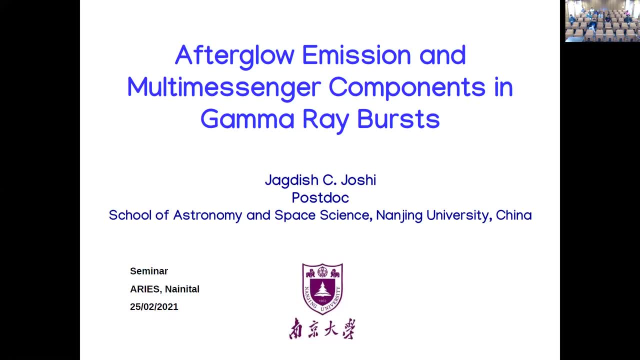 and looking for a girl to get married. so in grbs, i believe his experience has really helped him to understand grbs to a very large extent, i would say, and he has submitted a very nice paper in mnrs. it has been reviewed and soon it is in public. so you will see that how he has really done with all the way from synchrotron to 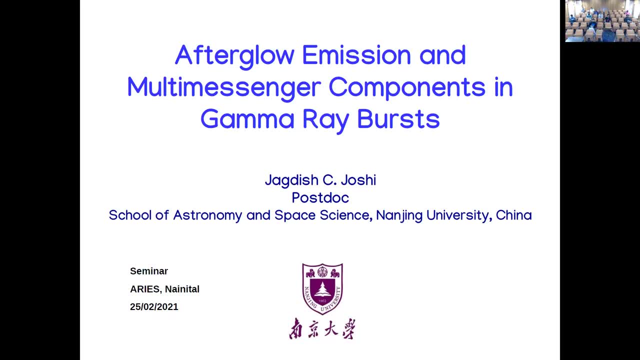 synchrotron self-competent and how he has really done with it thanks to this talk offline after one year? definitely. so i will talk about after doing mission in the memory burst and this topic has become interesting in last one or two years after the discovery of uh. 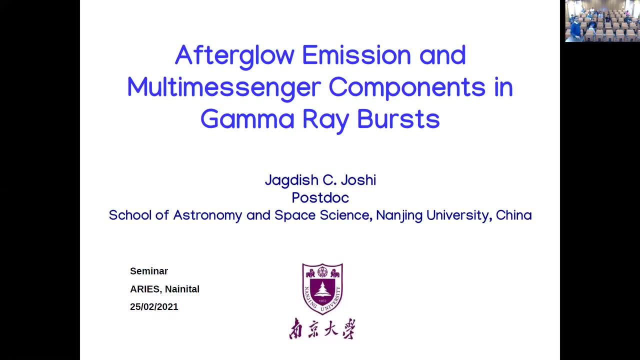 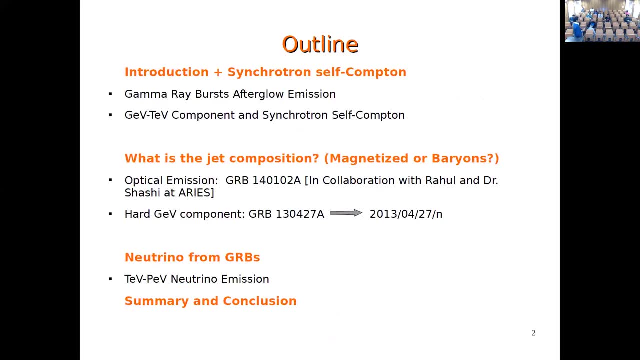 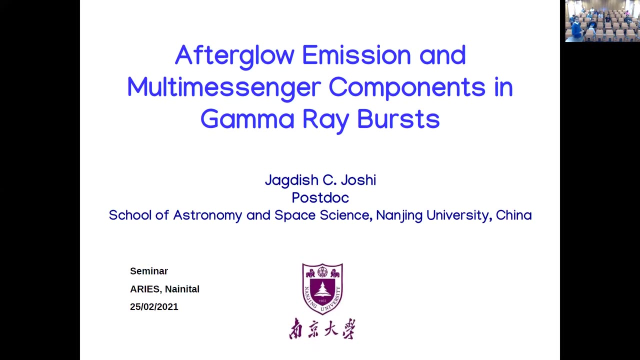 after the discovery of GVTEB component in Gamma Reburst. It was predicted in theory, like 20 years back, by Massaroos and Sari and Essene papers, and recently it has been discovered by the ground based telescopes. Other than that part of the talk, I will discuss about reverse shock component. 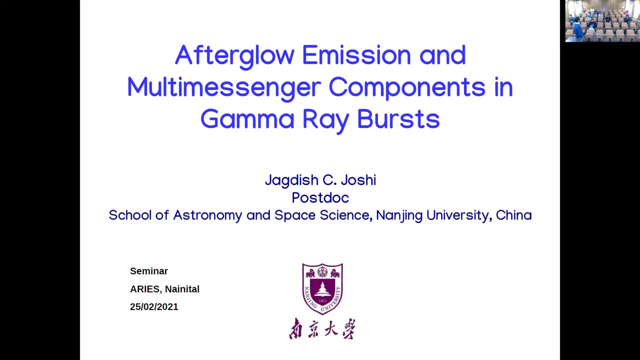 how it can be useful to understand the jet composition and in some cases, particularly the jet composition, some component in GRB can be useful to study the jet composition and the last part of the talk will be about the neutrino. and then if we can understand, 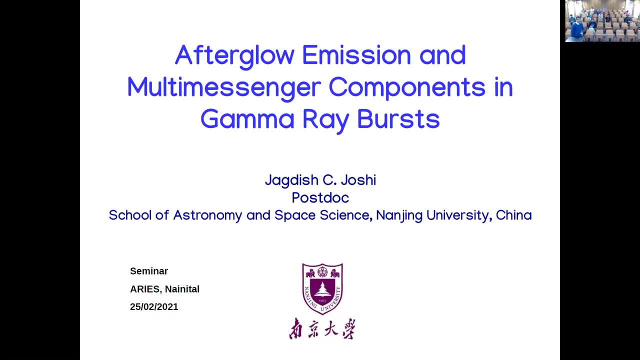 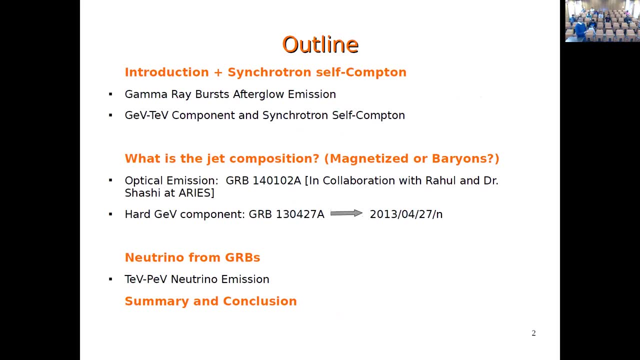 something about GRB and supernova connections. Okay, so the outline of the talk is like. I will describe a little bit about synchrotron self-compton, which is now observationally confirmed in GRB. It's very well known in the Aegean and Glacier community. but 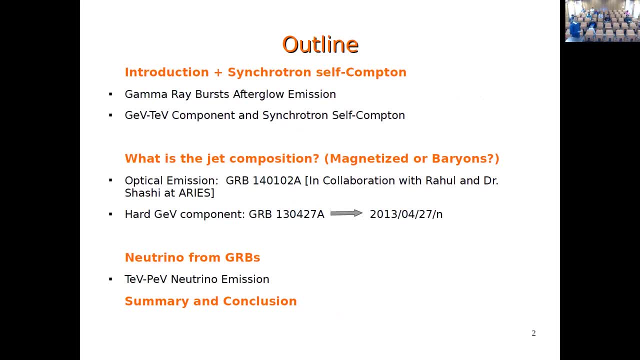 now at least we have one or two examples where this component has been observed. The second part of the talk will describe- I will discuss about the jet composition- how the optical emission in GRBs can be useful in some cases to study the magnetized properties of the jet and some of the component, if they are. 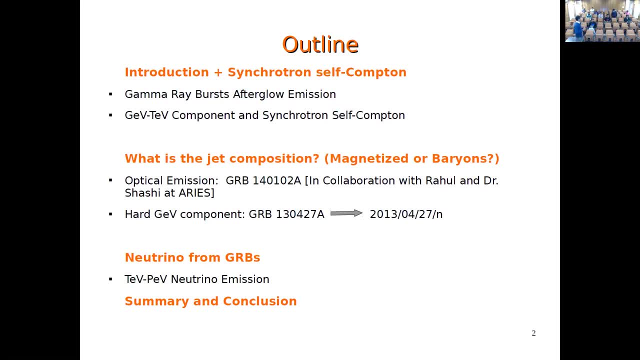 seen in GRB, They can be useful for the study of baryons. The last part of the talk: if I get sufficient time, I will discuss about the GRB jets and how, if in some cases, particular parameter space, they can be useful for detection in the neutrino sector. Still we don't have 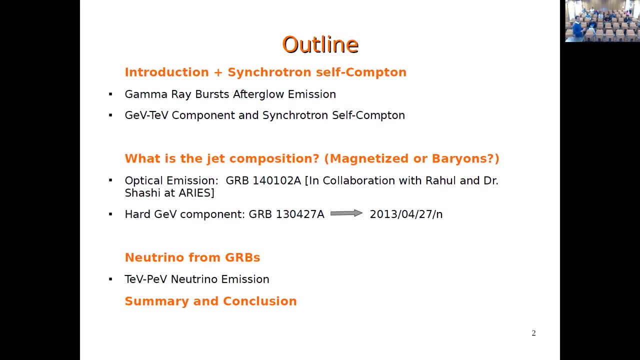 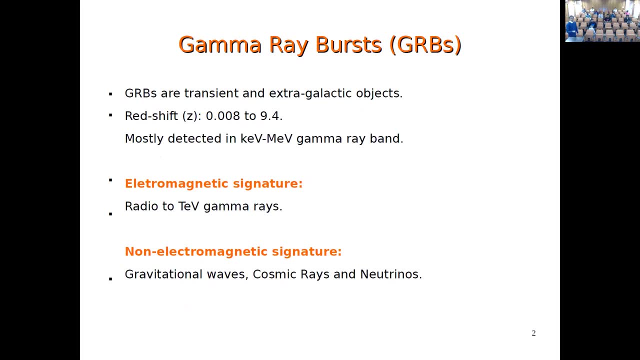 neutrino from GRBs. so but still there is a good hope that these objects can be discovered later. So we know about GRBs This we know. they are transient objects and they are extragalactic well known in KEB and MEB band and their signature is like electromagnetic, in particular in afterglows. 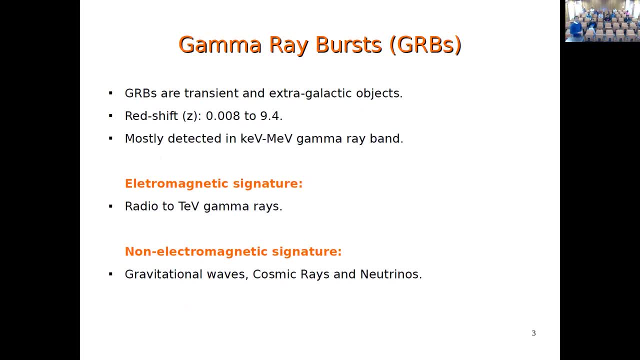 now they have been observed in TV coverage. The second part of the talk is like about, in particular, GRBs. we know they are produced by very extreme events, like the merger event or collapse of the stars, and these processes basically can lead to signature of gravitational 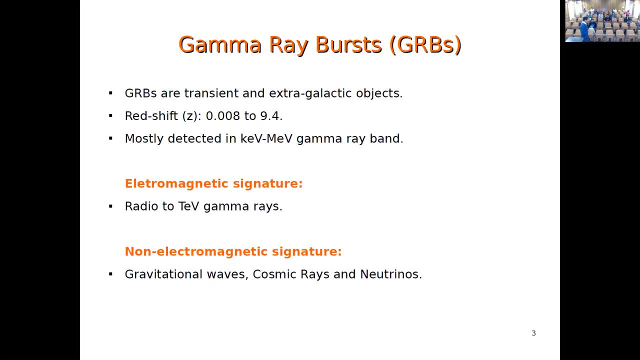 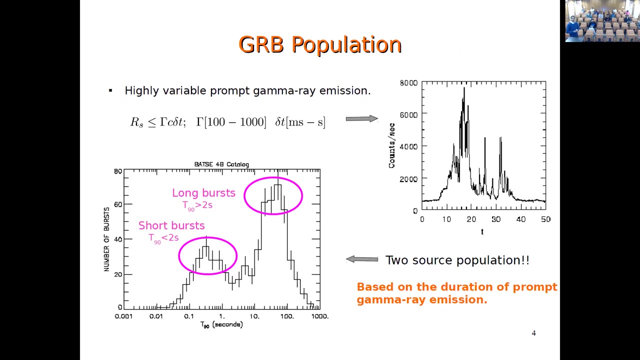 waves and in particular low luminosity GRBs. Maybe I will not talk much about them, but they are interesting sources for cosmic rays and as well as neutrinos. About the population, we know they have two populations, like in the prompt emission. what we observe Suppose the detectors start detecting the prompt emission from each other. 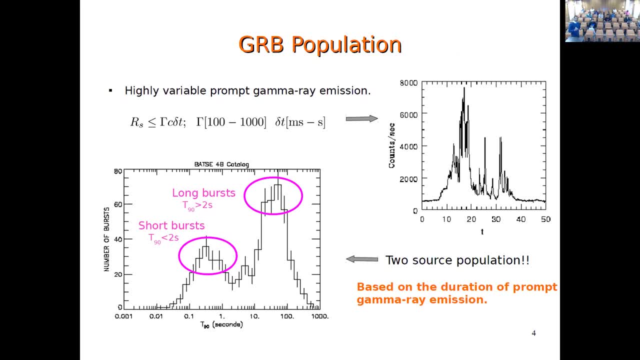 the first one is the GRB, and then there are many pulses, suppose in the bus it will take. the counting can take like more than two seconds or 90% counting. that kind of bus call non-burst. the second type are short. when the pulse duration is of 90%, counting happens. 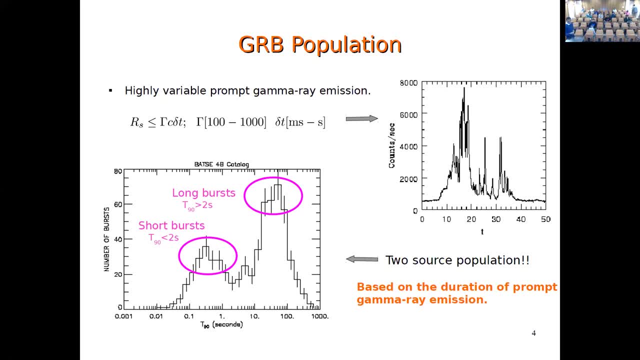 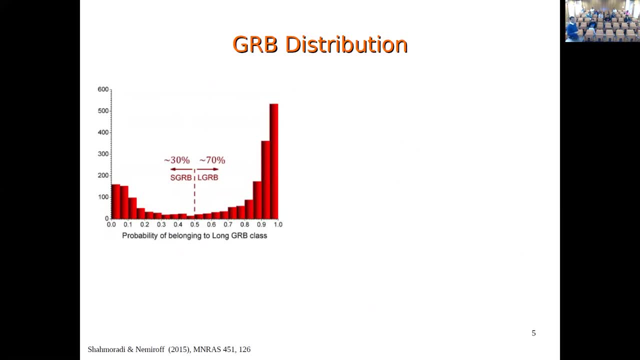 population. further bias towards long GRBs and we know 70% of GRBs can be long and fraction like 30% can be short. About their distribution: definitely, the rate is very high, one per day. So if you project on the projection map they basically looks isotropic Here. 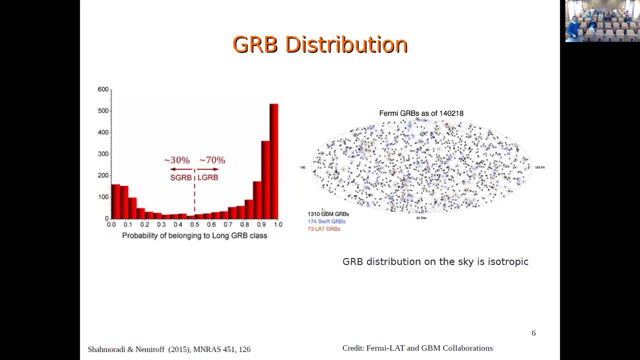 you can see, like the GBM has in this plot like 1000 GRB, which is basically the KAV-MAV band. In the left you have 100 GRB. So that is basically the GEB component. So the GEB component is not very. 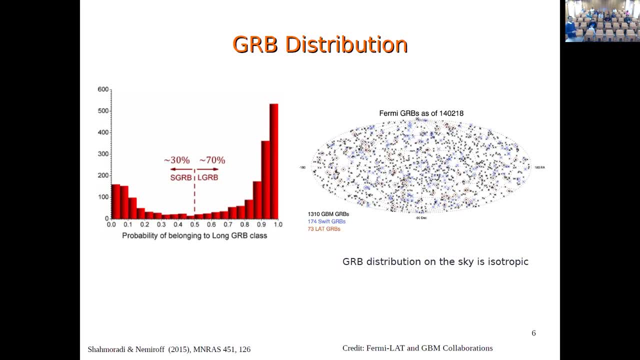 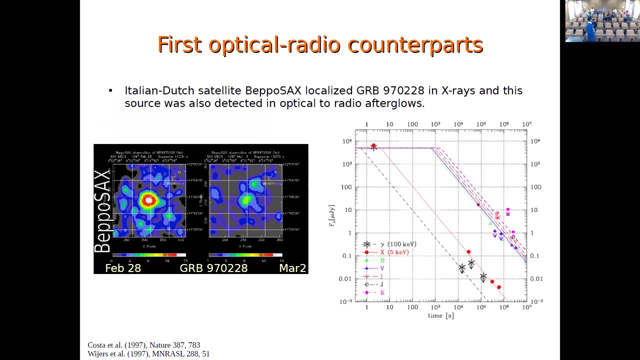 universal like. fraction of like 1 by 10 of GBM-GRBs have GEB photons. Short question: What is the difference between them, apart from the time? Long and short? So the next few slides will describe it. So in the previous slide. So there are quite significant. I mean I do not know. 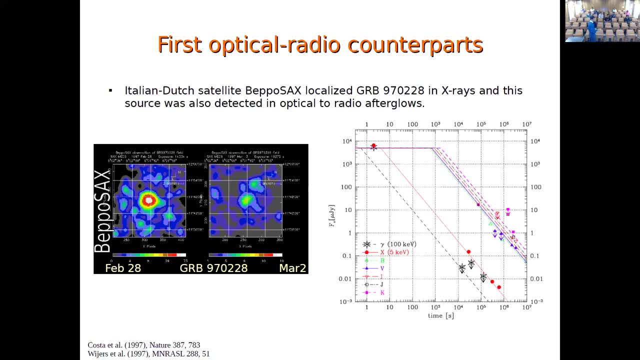 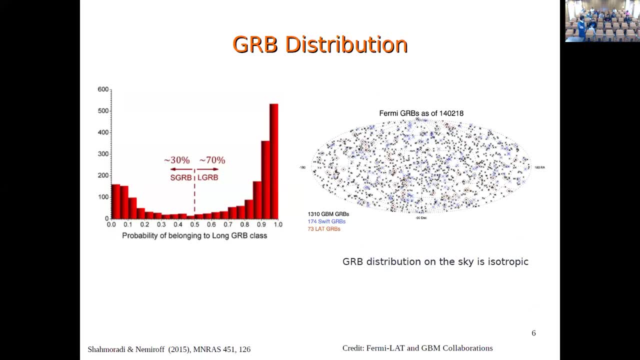 There are GRB detected along our galactic plane by Swift. Are these nearby? So this plot you are talking about? Yeah, yeah, exactly. So this is like, definitely like an isotropic distribution, but if you see Swift, basically this: 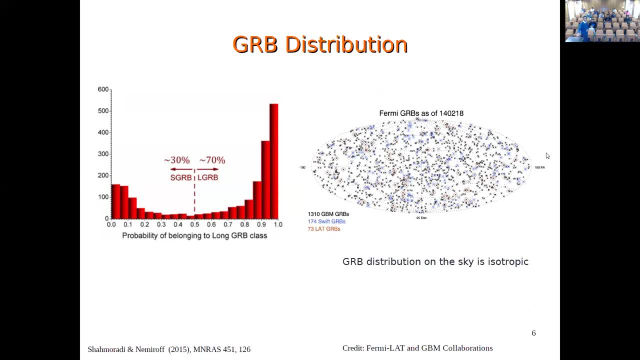 Yeah, exactly, There are quite a quite a number of along the galactic plane. Definitely we know they are not from the galaxy. They can be, like you know, looking like if you see the plane exactly. definitely they do not associate there, but they can be in the hello. 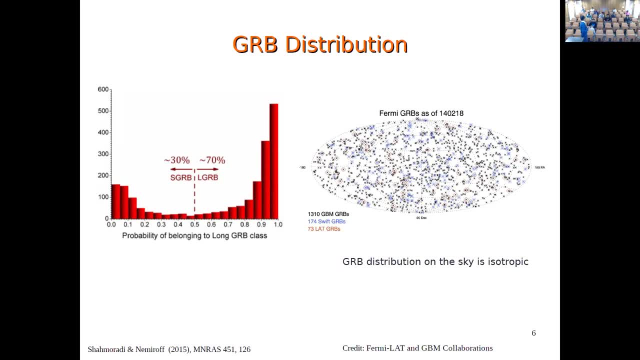 light, but not associated with the galaxy in the background somewhere? No, because the density is too high, I believe. I do not know. One should not expect to observe them, at least in Swift, if I believe. I mean no, the Swift is the. 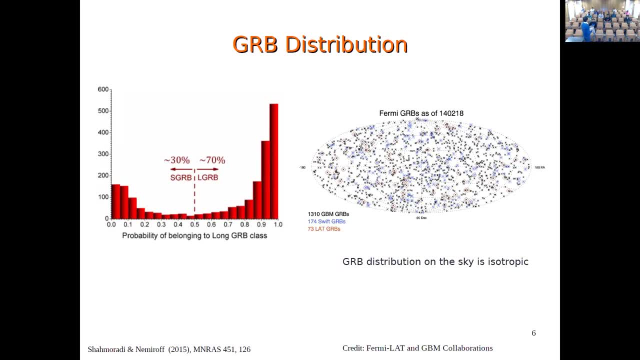 the XR. basically Swift has the XRT band and the GRB are generally observed by the Swift because it has bat which detects the No bat is not. And then it is a Kv, And then Hundreds of Kv. 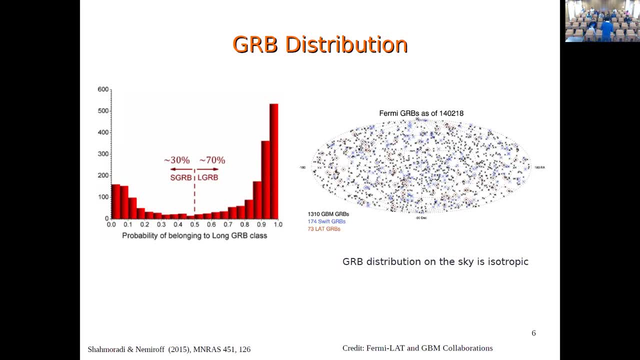 Yeah, then the XRT, which is like 0.3 to 10 Kv, and average GRB is basically: Yeah, that is 15 to 15. 15. Yeah, okay. So average GRB: you will see a light curve in XRT. 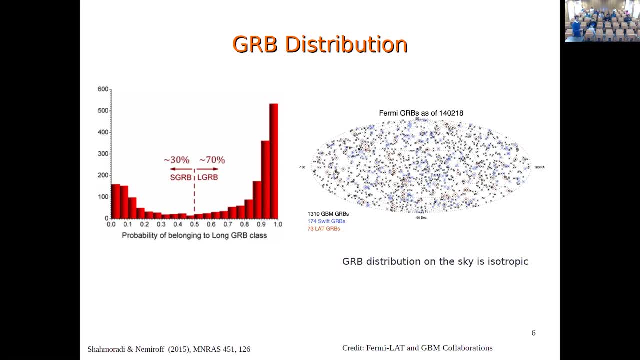 It is 15 to 15?? Yeah, exactly. So that is why, because I was expecting that once your number density goes to like 10, power 2420, maybe it would be like 100 KV, but it is not like that. So in the case of XRT, that is the same. 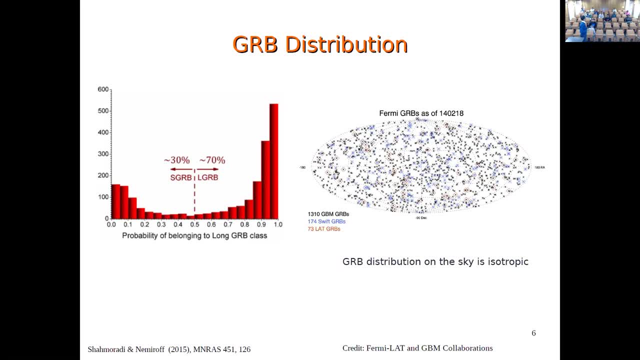 24, 23, which people usually call compound thick area, but that's what it says is actually. you don't have any summer to 10 kev, okay. so if the grb is happening, grow, i mean along the line of the side of this galactic plane, okay. and given that our is a seaford galaxy and the whole mass, 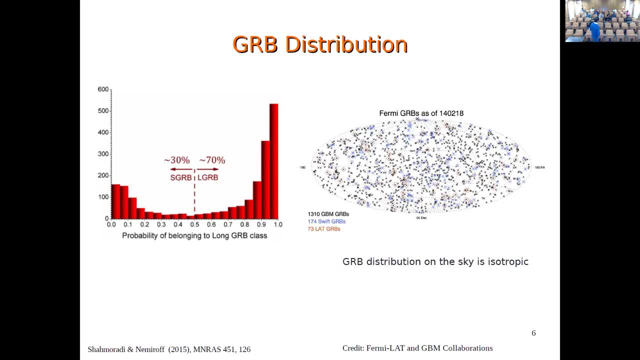 is like in this spiral. i don't know, but i was expecting that one should not see there, okay, so i'm not sure. like maybe, probably, maybe on the other day, i don't know, but even so. so one point here: like this: swift is like the satellite. can you, can you figure out this? 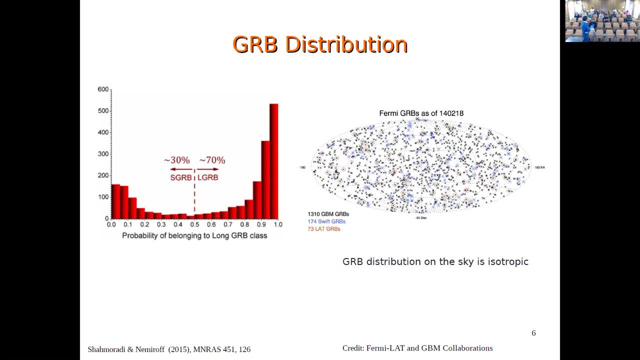 no, no, no. yes, it's like the same for eight kilo parsec distance that we are. uh, few kilometers is that. i mean hundreds are thousands, even thousands of kilometers is nothing for that. so so maybe we can discuss later. but every grb has xrt a light curve. i will show you. yeah, that. 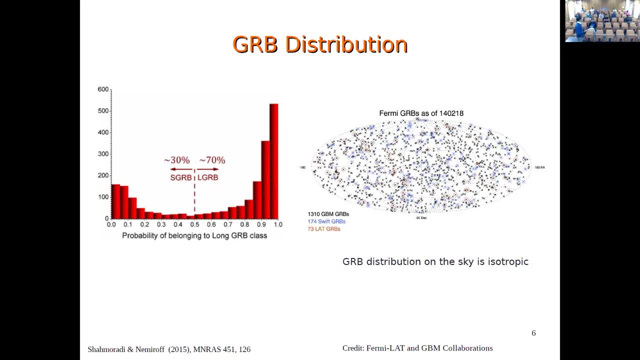 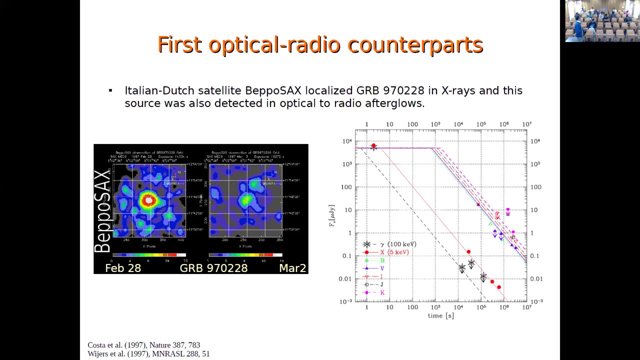 is that i know that every the whole field is driven by this, and maybe it was actually constructed for the same. yeah, okay, but actually this could also be the projection of what you are seeing, of that, such as having more than numbered entities. no, no, so that's what i just said, maybe, so i was. i was, at least in my opinion. i was not expecting 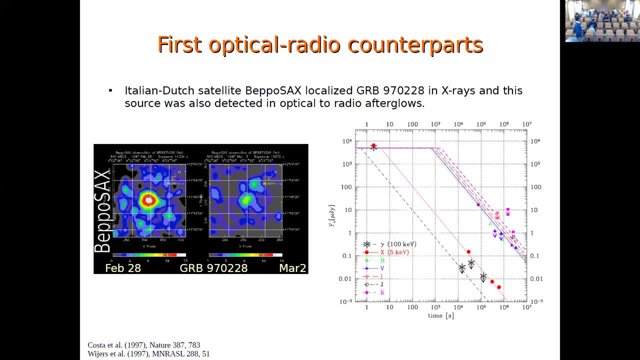 that we should see at least in swift xrt along the galactic plane. beyond that, that is okay. it may be beyond that, but not a problem. but uh, i've even seen that, but not in xrt. but that was i. i still don't know, so okay. 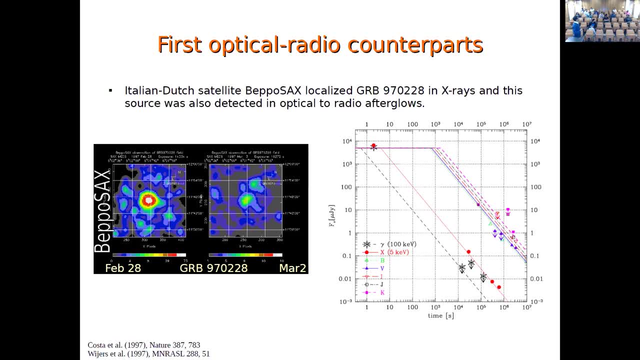 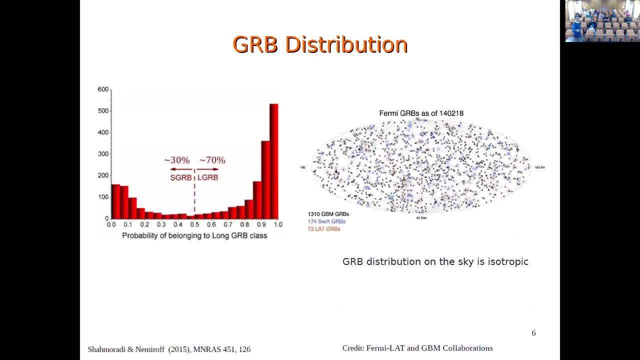 this is the switch. this is the switch. this figure is only for high energy. it doesn't have anything, i don't know. he has written three like bat and that and gbm and that, so all in the case. ah, okay, so i, okay, i the first one. i read that it is just the swift and second, i read it probably. 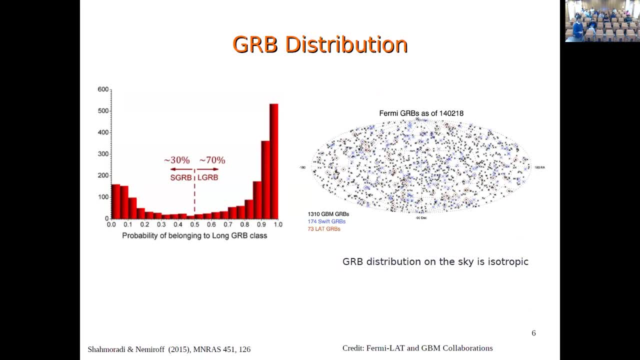 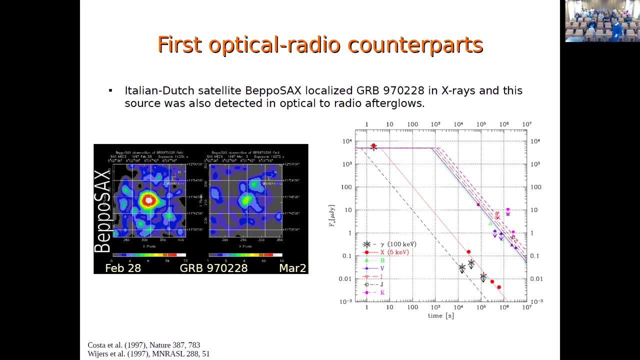 exactly, xrd. okay, now it is clear. yeah, that's right, thanks. yeah, then it is fine, okay, so, so, yeah, so the the whole uh point of this talk is about upper glow emission and this plot uh shows like the discovery, the first upper globe, which was in the in 1997. uh, the name of particular grb, which uh goes like this, is the year 1997. 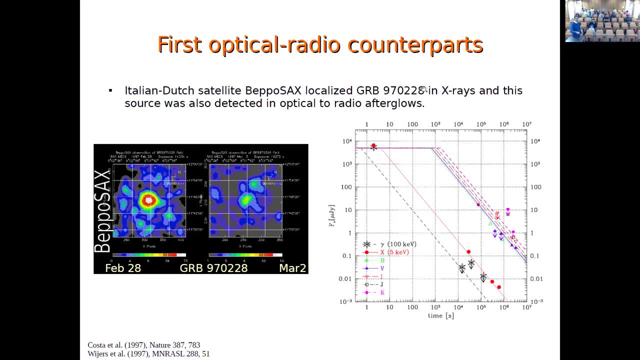 then comes the month and then comes the date. uh, here, uh, first the bepo sex, which was, which was an italian satellite, discovered the x-ray, and then, uh, after the localization, the optical telescopes found that, uh, it has optical afterglow. so this was basically the confirmation of the prediction of the afterglow models. 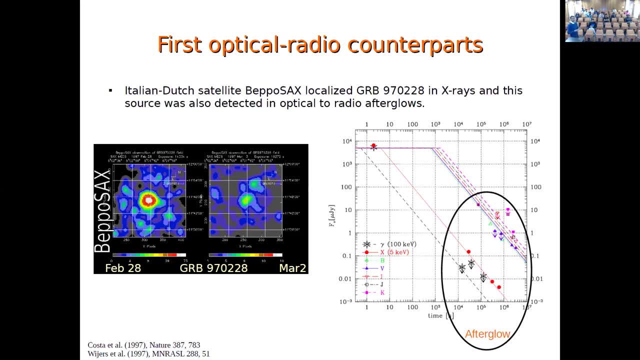 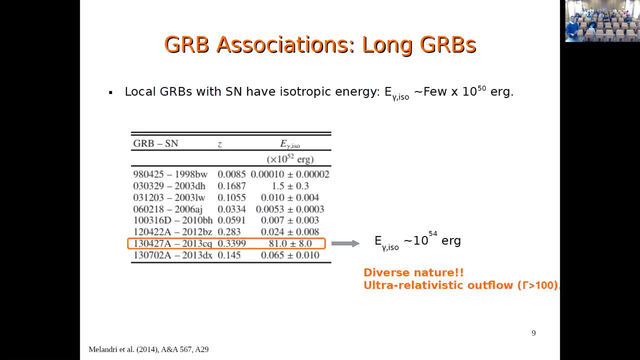 where it was. uh predicted that uh, grb, which are the burst emissions, would have signatures in the in the late times. so now the point comes about: uh, what, uh, what will ask about the association? so we know that grb, uh, in particular the long ones, they are associated with, uh supernovae and uh in the local uh redshift. 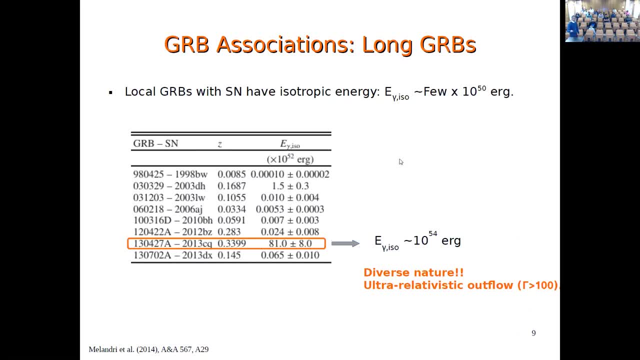 like less than 0.3. the energy goes around a few times and it goes 50 yards, but there are like excess absence. uh, for example, 130427a having redshift 0.3. uh have energetics like a cosmological grb. so similarly, uh, recently 190114c, which is like a tv grb, again having a very local redshift. 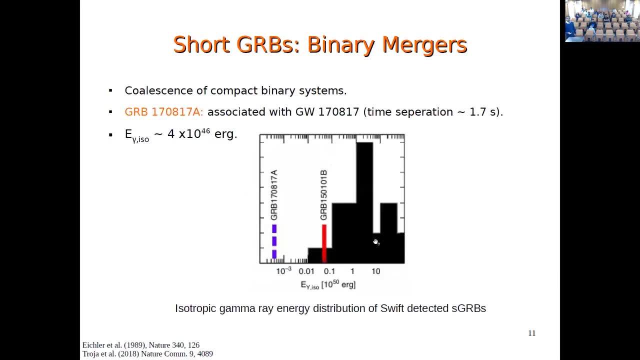 have very, very high energetics. so so, more or less for long grb, it is well stabilized that they are associated with supernovae. recently, in 2017, this short grb, which was very, very low in the luminosity, basically the extreme lower end, uh, in the limits in the energy distribution. for short grb, most of 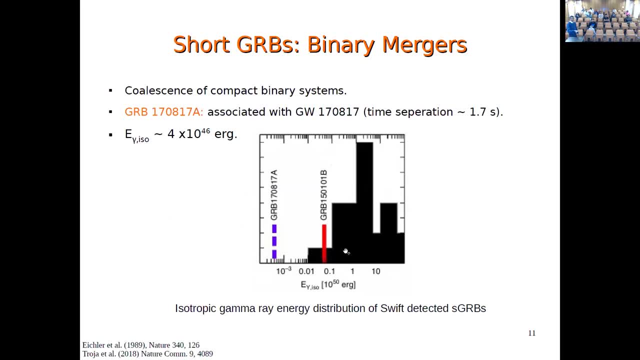 the short grb you can see have energy, something here, isotropic energy. but this grb was the limit. this grb was the limit of the light weight, of the everyday light absorption in this case. so, for example, this long grb would be 10 000 times lower, less luminous. 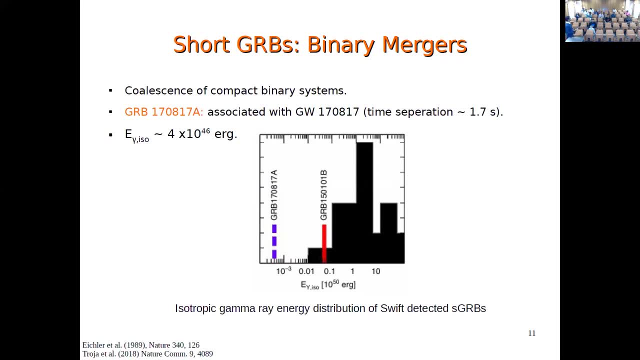 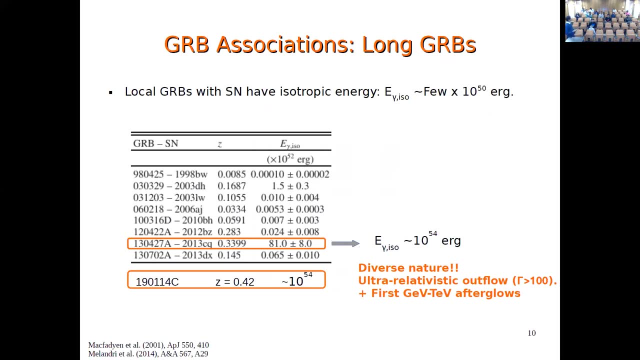 so this uh long grb and supernova connection is from the afterglow study, or yeah, definitely. now you see a grb, then you localize it and then you see the optical afterglow, do spectroscopy and that's how you figure out this. so, uh, for 130427a you, we didn't get any uh tv emission. 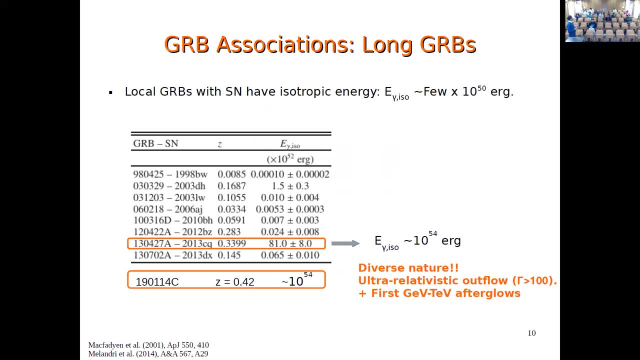 but i will discuss that. yeah, few slides about that. so, uh, for 130427a you, we didn't get any uh tv emission, but i will discuss that. yeah, a few slides about that. so, uh, here the energetics is too high and means the isotropic energy is too high and the rate 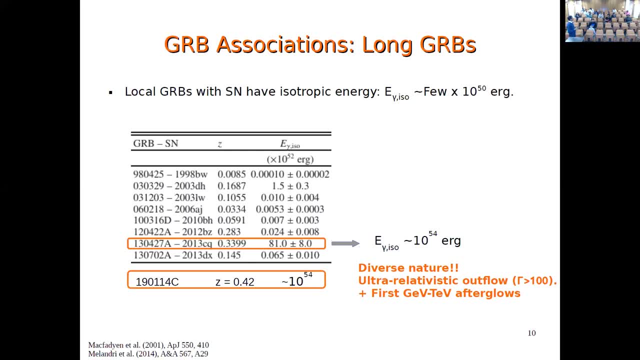 shift is also comparable. that means lesser than the 1914c. i have a slight comparing these two sources, because the dv is not coming from the prompt. this is the gamma iso. the tv is coming in the afterglow case, yeah, but the point is like i will show one slide, even if you see the 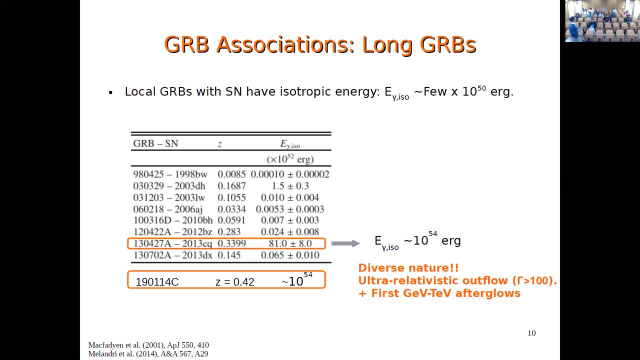 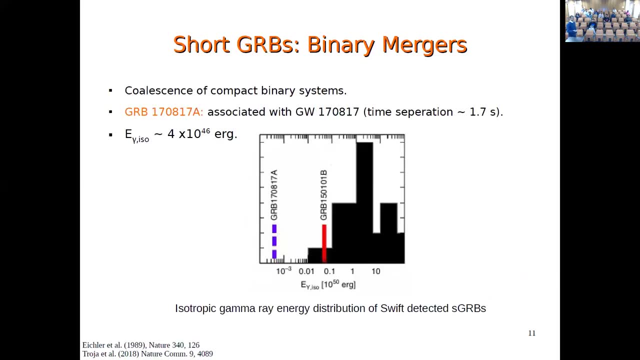 afterglow x-ray meter is very similar level for these two and we don't understand, like, exactly why there is no tv information. yes, and the source. so at that time these cherenko telescopes were there. yeah, definitely. it's like 10 years now. magic one was already there. yeah, maybe very fast. 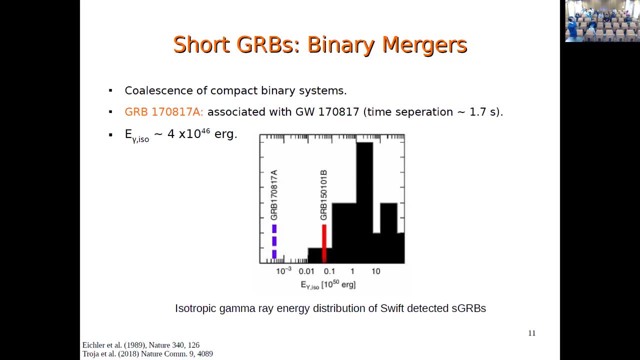 i guess, as it started. yeah, so that's what's there. magic is already quite backwards, so, uh, yeah, so this is the first uh scenario. at least it. it proved that at least in two cases of uh short grb the prognators are uh uh, merger of. 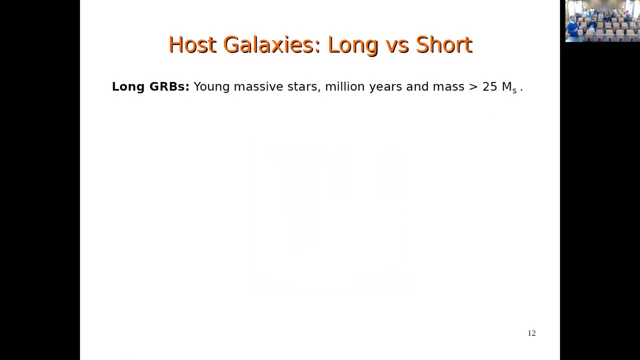 two newton stars. so now about the host galaxy: uh, long grbs. they are produced by massive stars. uh, because, uh, the whole point is like: uh, the explosion has to support something, energy, which is 10. we are more than 10, we are 53, 54 arg in some cases. so, um, and the association is with type. 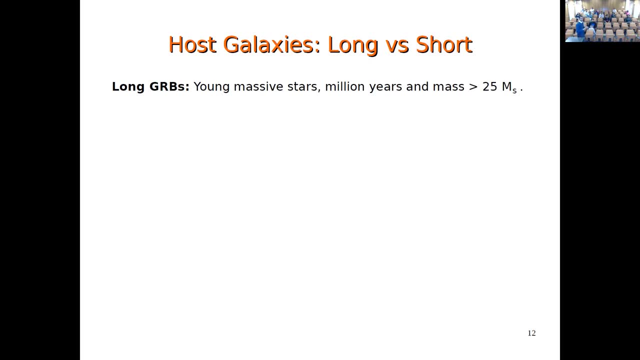 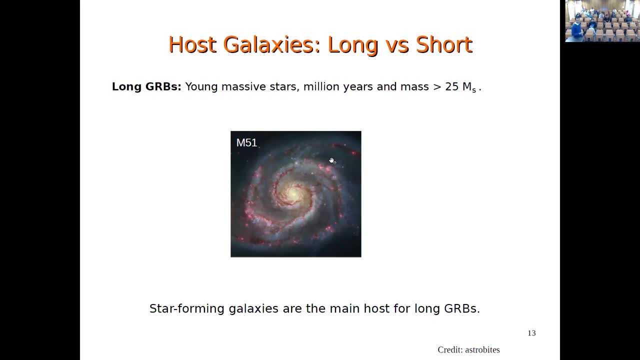 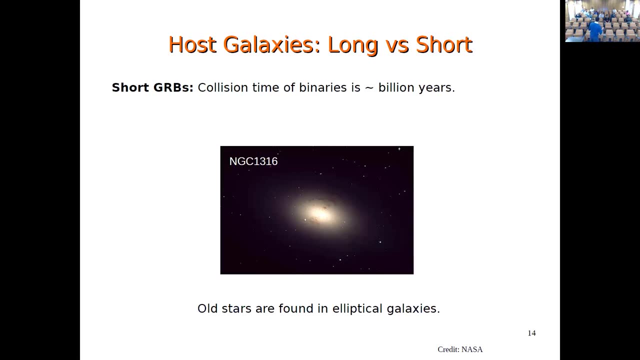 year-eve. so this kind of system can be associated with star forming galaxies and there have been a few cases where uh this has been associated uh about uh search grbs, uh. so what happens in songday armies? say you have these, uh, you have these, uh, uh uh. flying stars, neutron star in the. 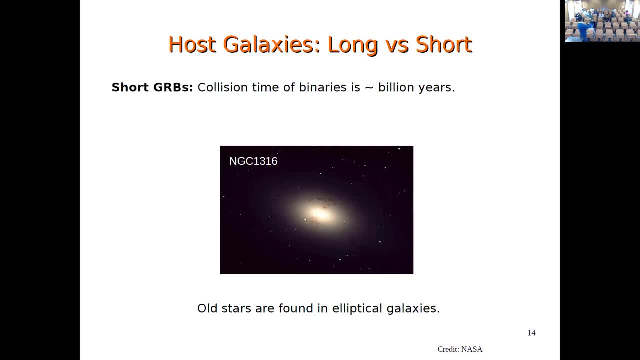 star and stuff, and they are very far and they have to come close to each other and then they have to merge and this process takes billions of years of age and for that to happen, the galaxy has to be very, very old. and you can see like elliptical galaxies are one of. 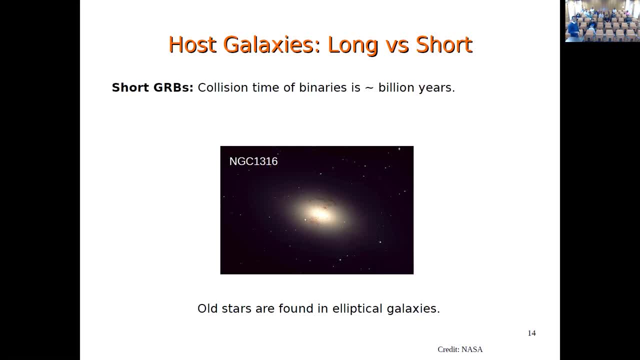 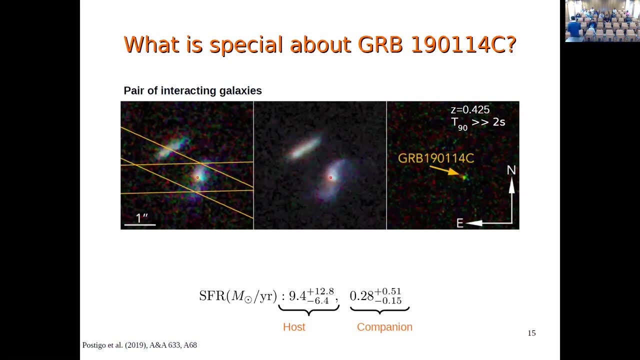 those where one can see the short GIB association. So about today's talk, where I will focus about 1901-14C. there is one paper which says that, okay, this is, this might be interesting. source. only one sample, definitely, but some of the 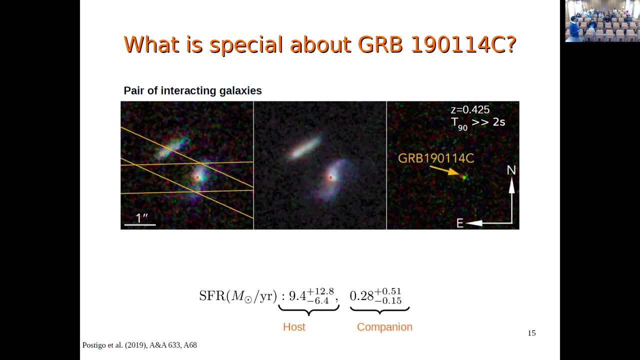 short, GIBs are also associated with the early type host galaxies. So in that case how can you explain that means if you are saying that the neutron submerges is taking place almost in 1 billion years or some billion years? So how can you explain that this can be found in the early type host galaxies also? 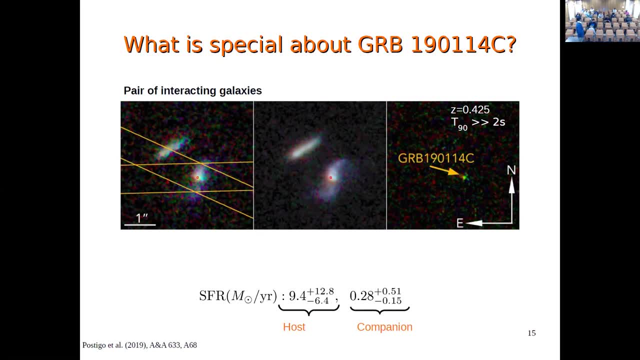 Because it is almost 15% and 85%. I know, 85%, I know, but I don't know how much it is. Yeah, Yeah, 55% is in the early or late type galaxies or the elliptical galaxies. 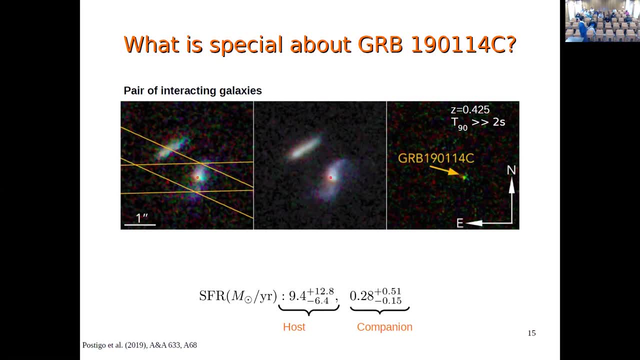 So exact answer. I don't know, but I can say I don't know, I have to check it- but maybe the consonants, maybe the systems- I don't know what it is, Maybe mixed bank also. Really, yeah, I have to answer it later. 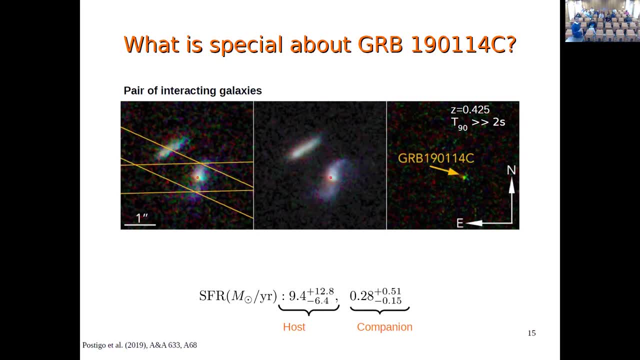 So about this GIB there is? what has been located here is, you can see, this is the location of GIB and it is a pair of of interacting galaxies. Some of the idea in this paper is maybe this interacting galaxy systems makes the environment. 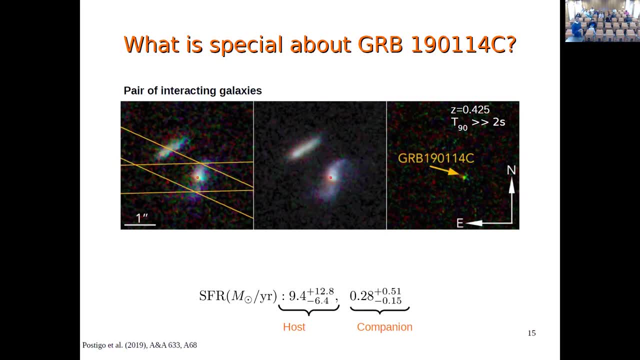 or gas density, something different which leads to GVDB component. It's still not clear, because one has to see a larger sample in future, maybe, and that it can be that it can be more lived upon, But this galaxy happened in the center of this lower of the galaxy, right. 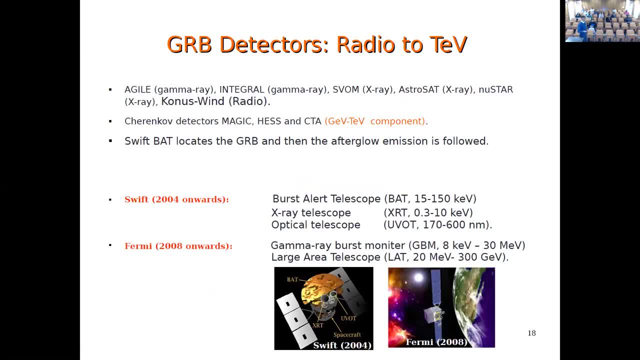 No, I'm sorry, This is GIB. I'm sorry, Yeah, Yeah, So you have these two star forming galaxies. Yes, This is the host having 9.4 solar mass per year star formation rate And this is the companion. 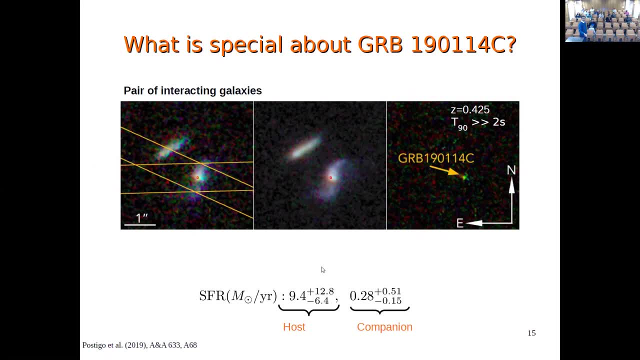 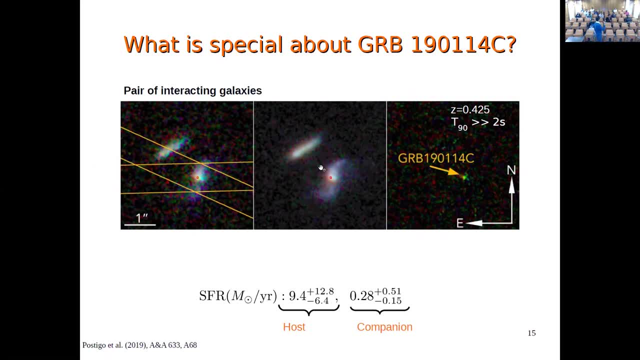 let's see what the LKT is going to be. So projected separation in that one will be like kilo parsecs- Okay, It will be more than kilo parsecs, I don't know. hence kilo parsec and two galaxies that kilo parsec. 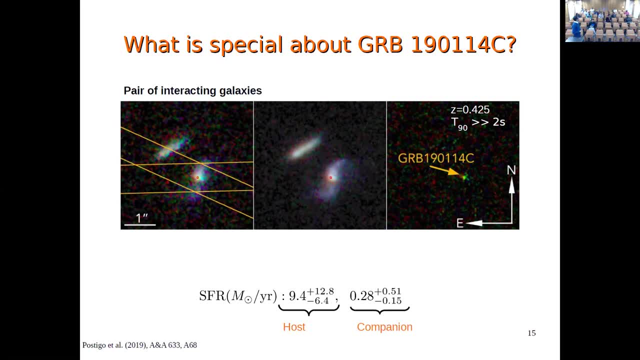 Are? you are saying the separation between these two? Yes, Is it 2 receive into 0 us? it help to do for the Z and the young cell the continuous 밥 novels, But it mean there is a possible. And if you look at the plus equation, give me through the n внимание. 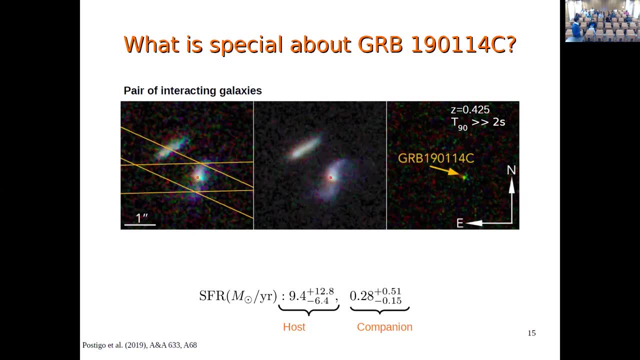 Yes, Yes, That is the property till you compute the 14 articles per day, So could it? some of those are the right answer. So yes, except our proves are typical valid And we don't know what's going to happen. 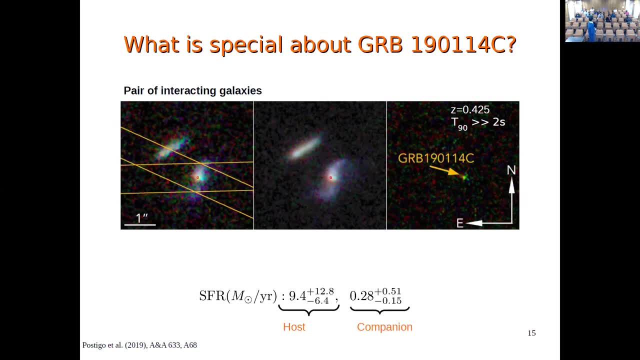 So keeping the information? Yes, It's in intention- is at kilo parsec distance, but So you are saying the separation between these two? Yes, exactly, So kilo parsec in some sense for the GRV, I don't know, it's quite large. 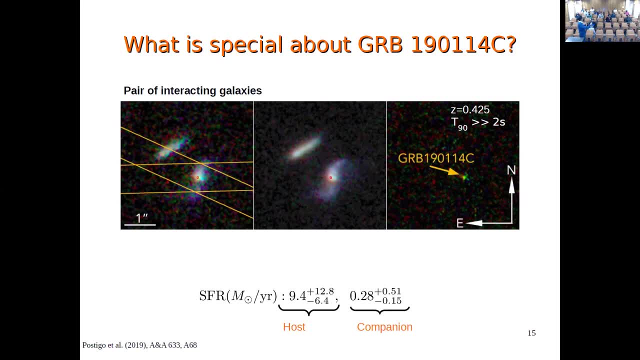 No, these are. these are two star forming galaxies which are interacting. Yes, that's what I'm saying. the separation like if you look at the one or second that you have drawn in the left: Yes, So roughly one hour. second separation right: Yes, And at z is equal. 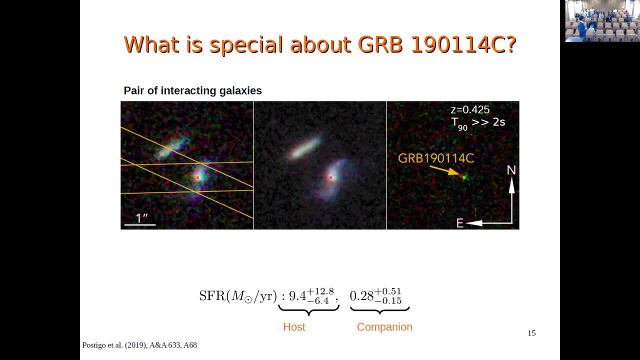 to 0.425, the projection distance, not even the actual distance, and it tells us that at least it would be tens of kilo parsec away. I mean the two separate separation of the two galaxies. So sorry, what is the point, like I didn't know. So you said that a pair of interacting galaxies, so 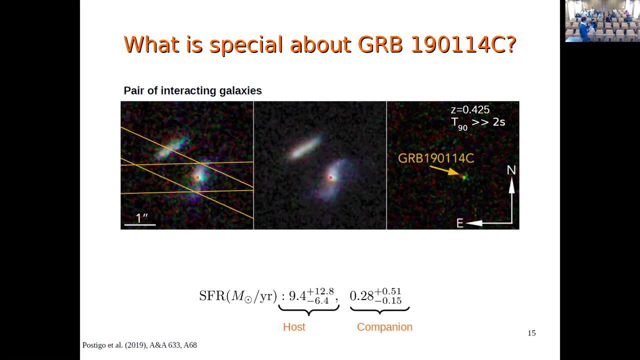 it makes the environment something. so I was trying. So that is the so this that is the point of the paper like because generally GRV they are associated with star forming galaxies and one galaxy in particular, like you know, star forming- well behaved In the. this is the first. 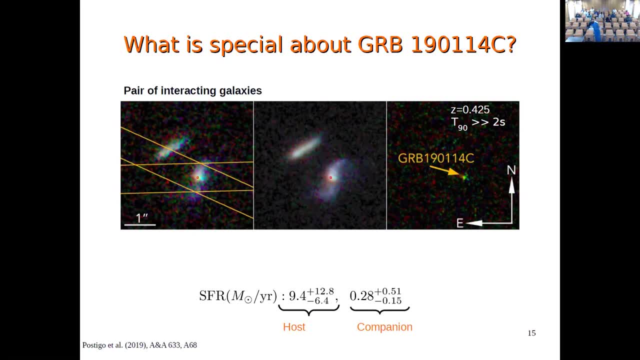 case where we have PV emission- we don't know, still like because this is associated with one high star formation Source and, by coincidence, it happens that you have another galaxy just close by. okay, it doesn't say much, it's just the paper comments that, okay, we have only one source, one sample. maybe this is. 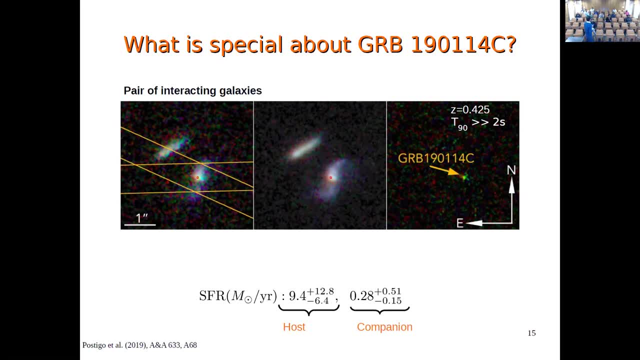 the region. but no, maybe not correct because one has to look for a larger sample, maybe 10 GRV inclusion. then it can be also on speculation. yes, speculation, almost So interesting. why did you always see something new? and that one gbt connection and then something like you know? 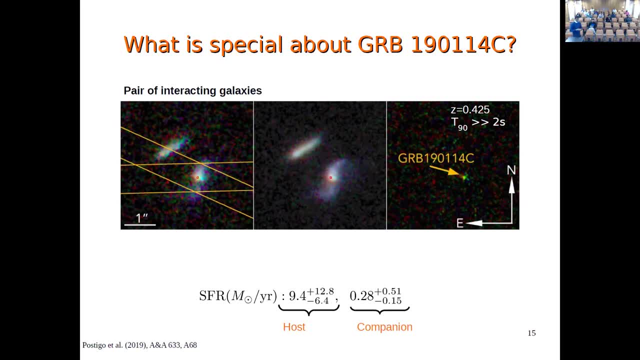 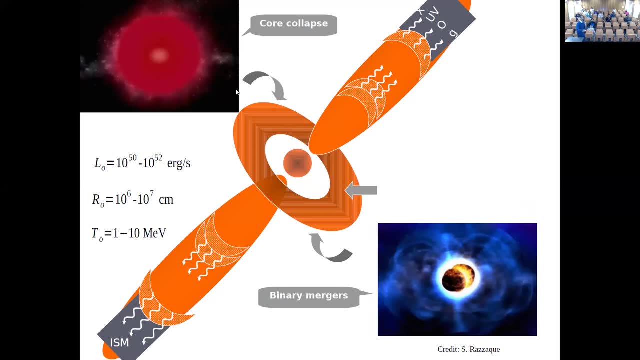 and then- sorry, the interacting galaxy. So so I discovered like: okay, we know about the Prozenegger, we have Kulebsar kind of and we have Merger kind of stuff, and so what happens like, so you have this, the formation of epicentrist and the central black hole. 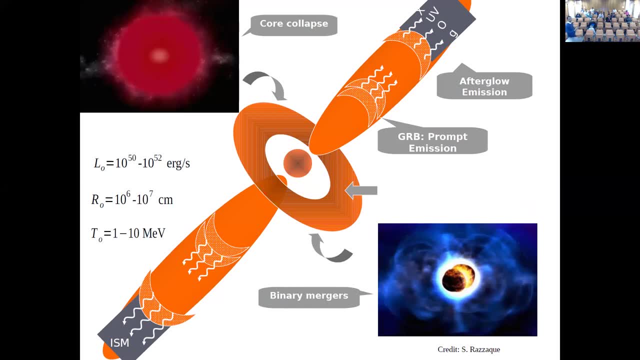 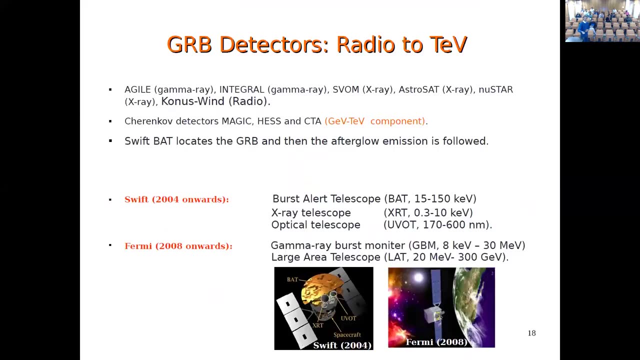 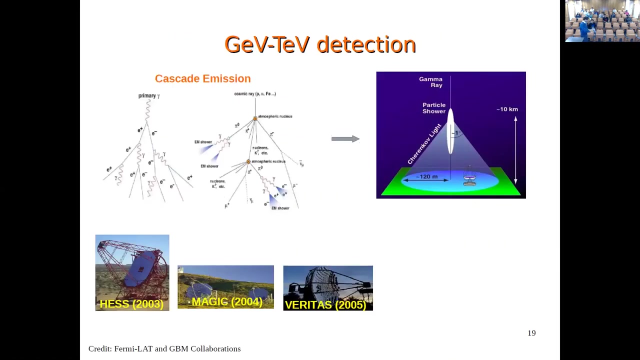 most of the angular momentum of the black hole channel along the along. this is what it's going to do to the other side, the media. Also, we have afires, and you know, and this is what we call the, the point, it, The point it starts changing the, the slide down. 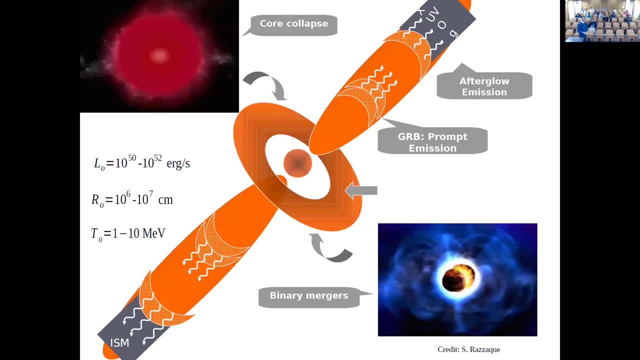 If you press and hold it, then it becomes a point. You just press it and just leave it as it is. no, if you press and hold it, then it becomes a point. okay, so, yeah. so this picture basically tells that, whatever it is like, either long grb and 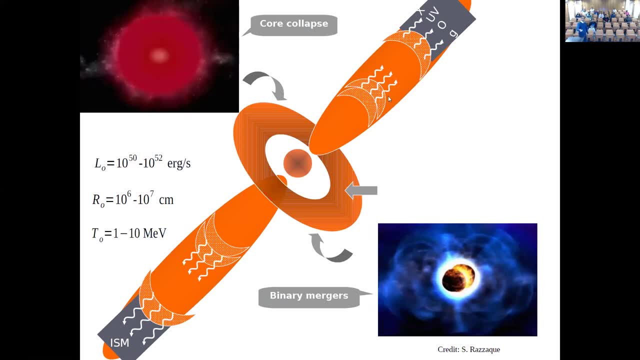 short grb. the end result is you have this: the dissipation of energy here. so this is very close to the black hole and then it can produce prompt emission, early time emission and, coming from the internal shocks, further part of the energy is channelized to the surrounding. 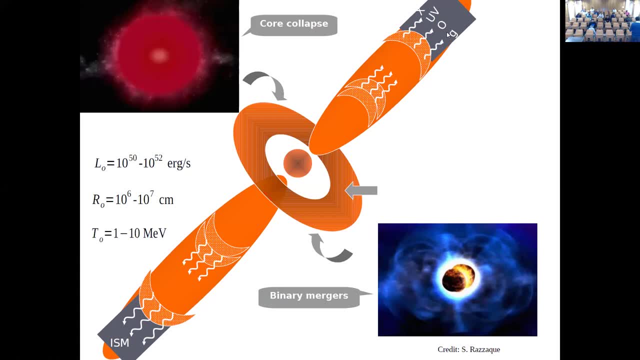 medium, for example in the. in the heavy massive star it is the wind medium, and for the binary these are constant. ncd is a medium. in these two scenarios what can happen in the afterglow is, if we model afterglow emission, we can figure out at least the ambient medium. or 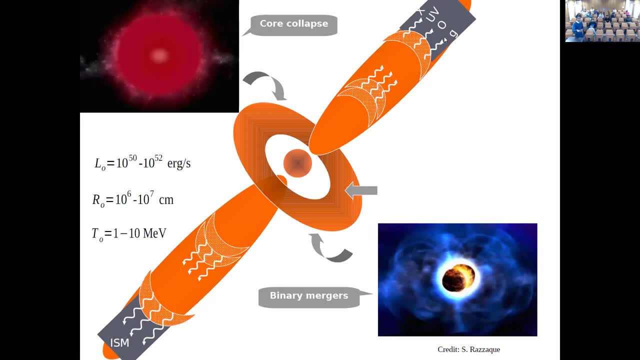 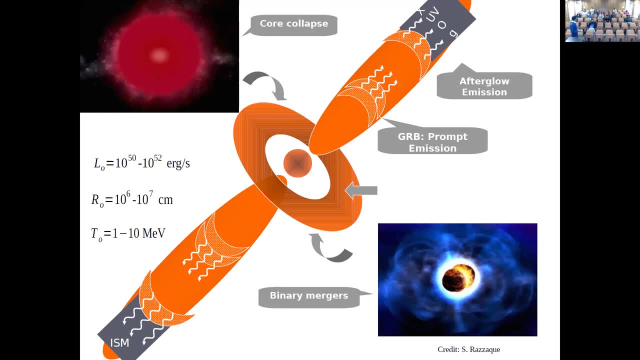 energy radius. why did you say that? of course, single-state museum of wind. uh, so yeah, in the sense like: uh, these massive stars they are, they are that the large enterprise established like Holiday of the, they have a win. so yeah, that's true, but the binary is like, one of the components is like: 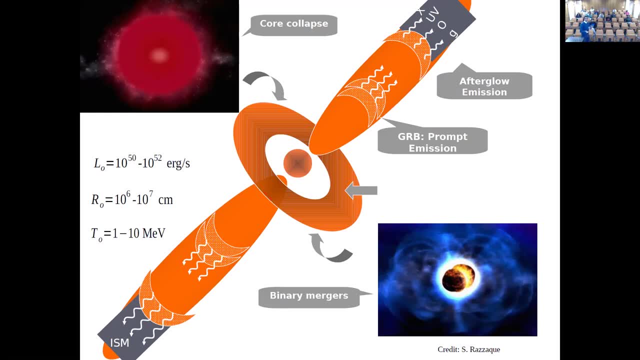 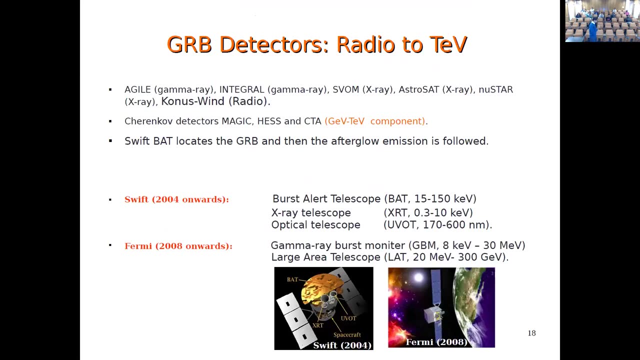 that then they should. so binary is like: mostly you have this Newton sign, you can start or Newton's from black hole and black hole and black demand, roger, yes, okay. so this, this just a picture to show that. okay, how many uh, observatories? yeah, yeah, forty, how many observatories? yes, 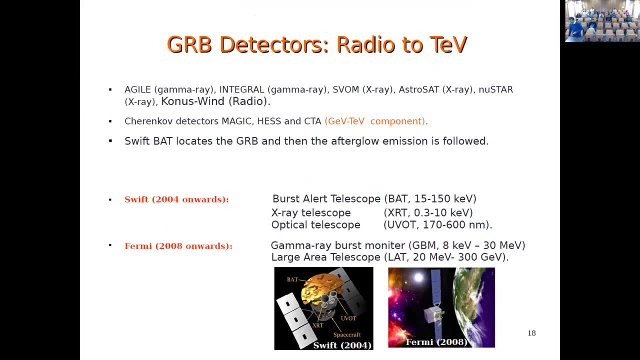 some of our. but you know i used this in companies. but, yeah, it's stable enough that you. you know they generally work to observe the broadband emission And so, with respect to the BAT, BAT is very good to localize the object Once the BAT locates the source. 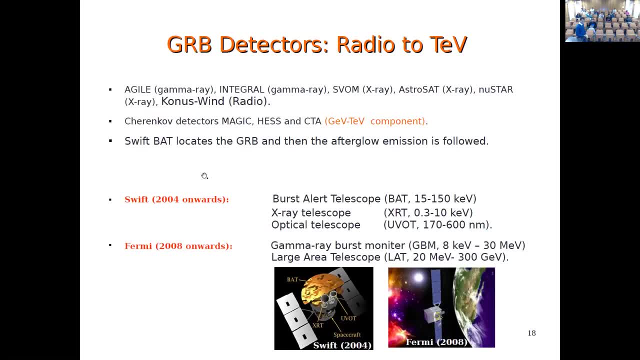 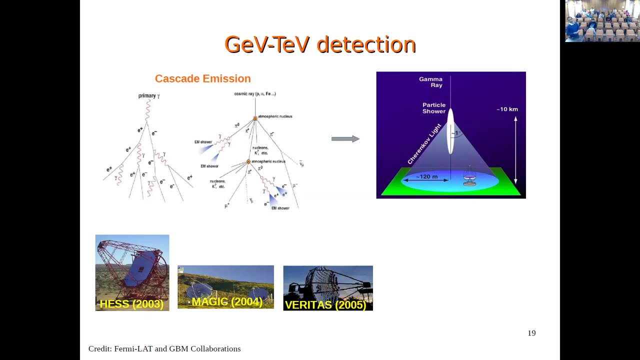 the information is exchanged with the ground-based and other telescopes And then the multi-wavelength observations are done generally in the ground-based as well as the satellite missions. About the GEB-TEB detection like it is like more or less 20 years. 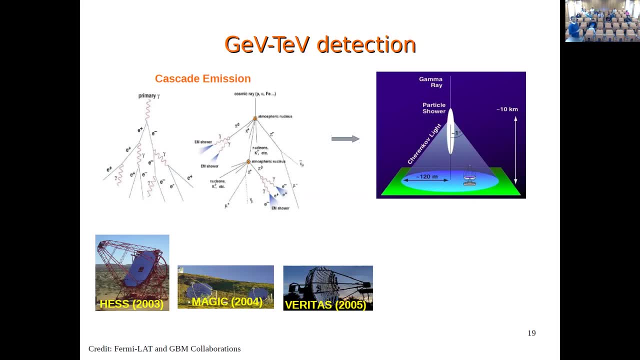 before it was predicted there would be a signal in GEB-TEB. I've never seen, but recently, these ground-based telescopes like HESS was already from 2003,, then MAGIC 2004,, Veritas, all these. 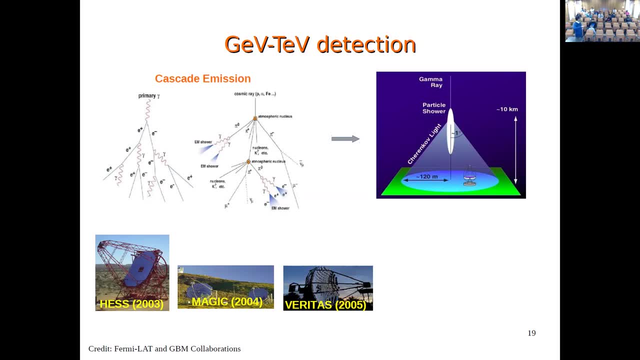 So what happens? like you have a GEB-TEB gamma ray. it hits that atmosphere, nuclei, oxygen and nitrogen- and then you have this cascade: particle production, electron projection. they are heavily relativistic And because of that they produce this blue. 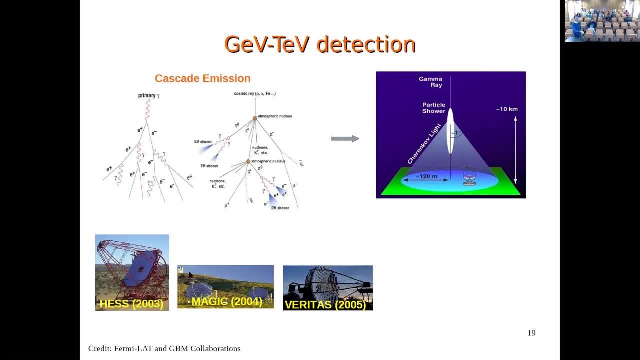 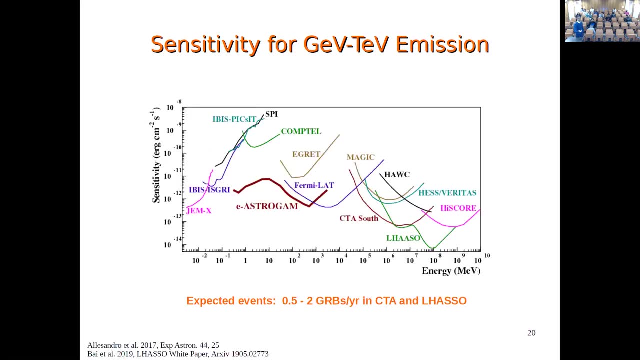 certain gold light which is collected by the mirrors And then reflected back to the collector And based on that, information of the sources is found. So interesting part So CTA was people were building CTA. LASO is the Chinese ground-based telescope. 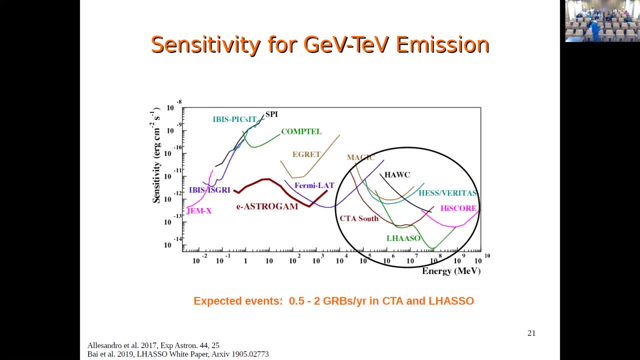 Serengo telescope there, But there was not. there was excitement in the direction of like EGN and Blazer, all the community, but GRB was like, not brief, Like you know. it's like there was like a spooky whether there will be a TEB signal or not. 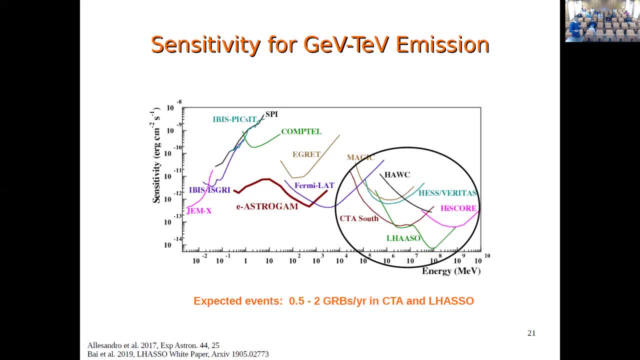 But the direction of these two telescopes, two GRBs, so GRB 19-01-14C- was observed by magic, Having this sensitivity. it gives a lot of hope to CTA having better sensitivity, 10 times better. 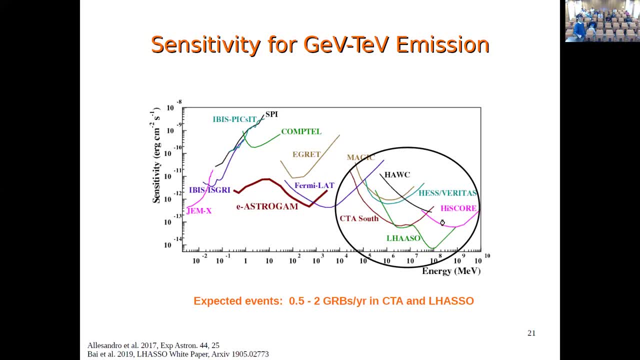 And then LASO, which completely here. So the hope is at least we can see in future like two events per year. okay, That is again. all things should combine. The GRB should be local because it is very, very far. 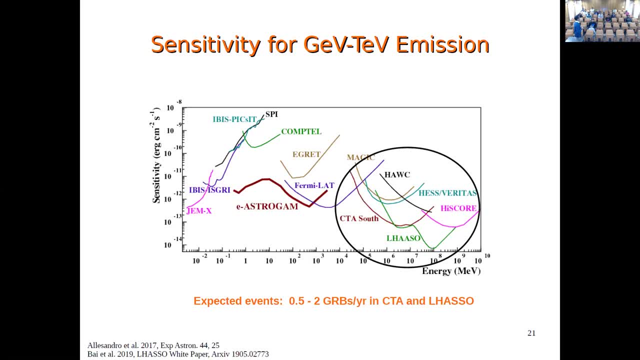 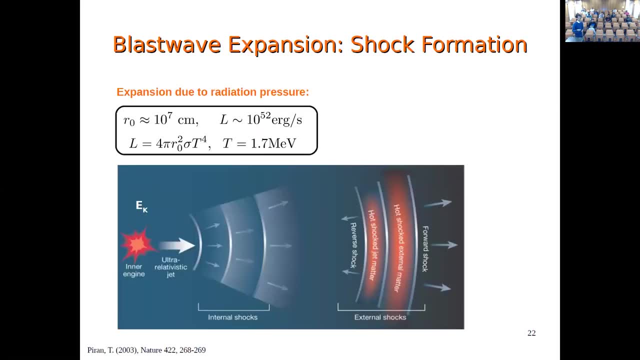 But then the TEB radiation is absorbed by the EGN and stuff. So it depends And I think future five and 10 years would be interesting. So now I will describe the R0 and this stuff. It just became here small R0, that's all. 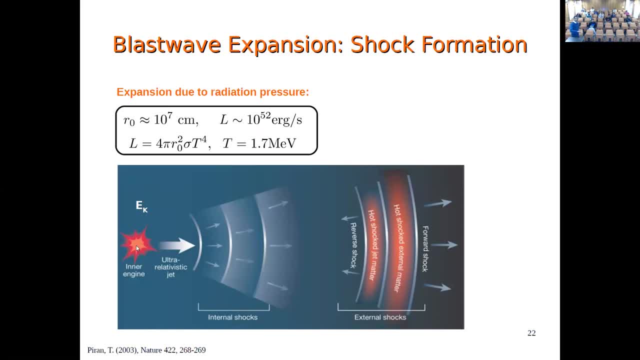 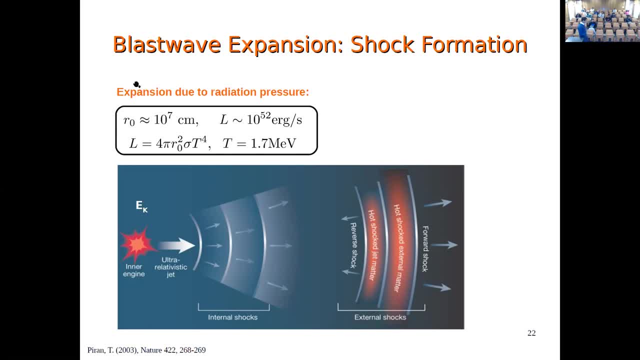 And then if you start calculating the temperature of this volume, a spherical volume, then you will find that the temperature is like around 10 to the power, 11 degree Kelvin. So this is huge temperature and you have a fireball or plasma. 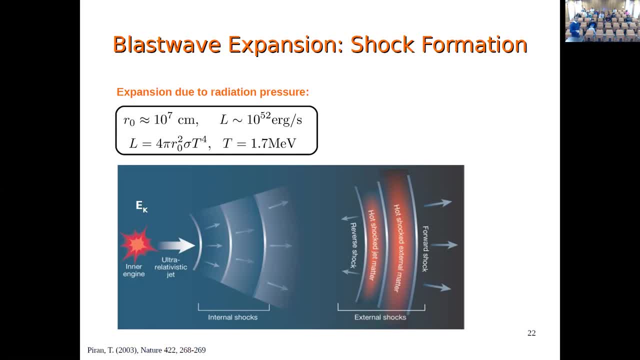 like we all know, magnetized plasma, all these things are possible, But what happens is this thing expands relativistically and that ends up having these jets. So these are the jet, collimated jet Here, these shells emitted by the central engine. 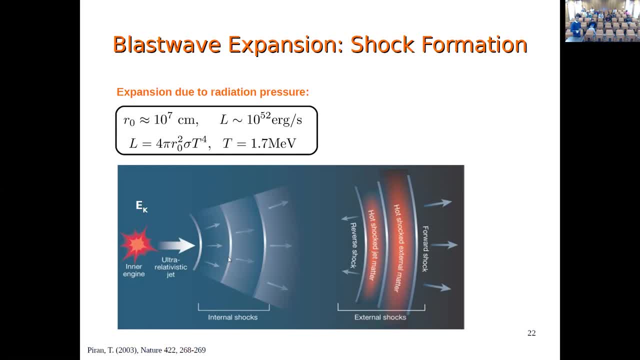 they propagate and if they catch up at some point they produce internal shock. Part of the energy from the central engine is channeled to the surrounding medium. And what happens when the energy channels the surrounding medium? it swaps a lot the mass with time. 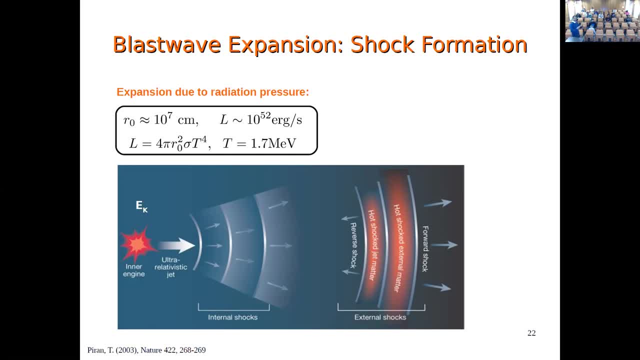 At some point of time what can happen is the channeled energy to the surrounding medium becomes approximately equal to the mass equivalent- sorry, energy equivalent- of sector of mass. In this situation, you basically start seeing the external shocks. So how external shocks form is like. 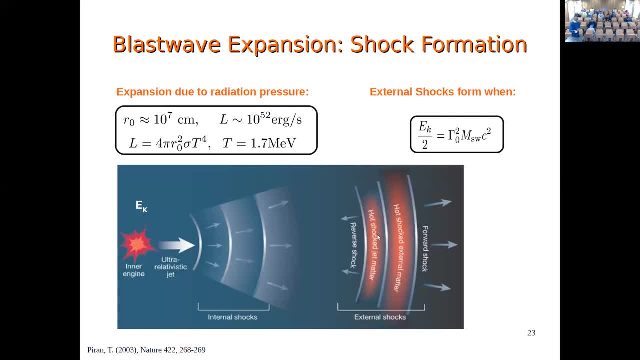 suppose you are in this frame. this is called co-moving frame and this is the galaxy. suppose it has frame And you have a particle here of like a proton. here It is moving relativistically with a Lorentz factor gamma. It will be like Lorentz Boolean. 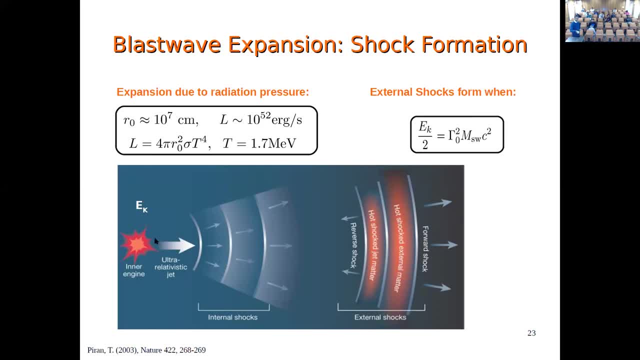 It will be like Lorentz boosted by gamma naught, MPC squared. Now we do calculation here. So again, this and this frame are having a Lorentz factor. gamma gives you a gamma naught square relativistic effect. So the comparison, which is like this, is the swept up mass. 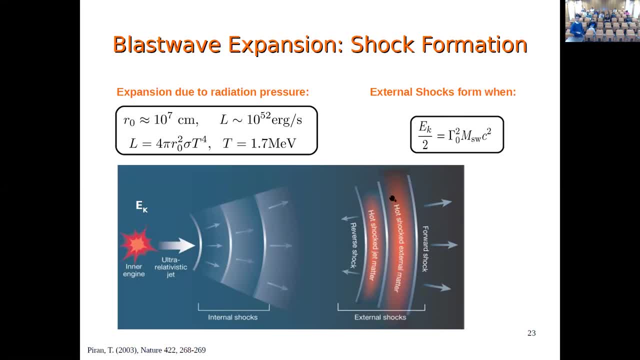 classical. having the relativistic gamma naught square boost gives you the comparison condition for external shocks, The difference when it is gamma naught square. So yeah, So that's what I'm saying. Like you have this frame, This is the frame where you have the particle aspects. 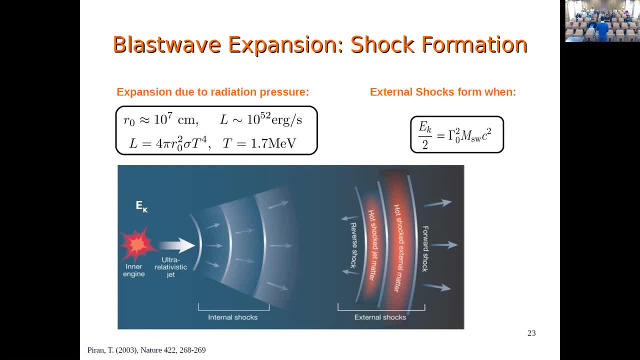 and basically the shock formation. So now, so you have this shock moving forward with a Lorentz factor, So any proton in the ISM will be at rest. If you go to the co-moving frame, you will see the proton is coming to you. 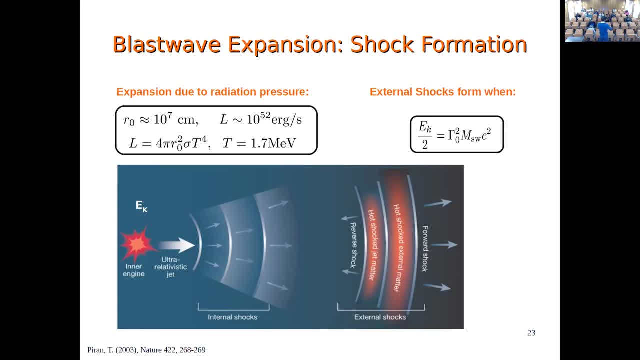 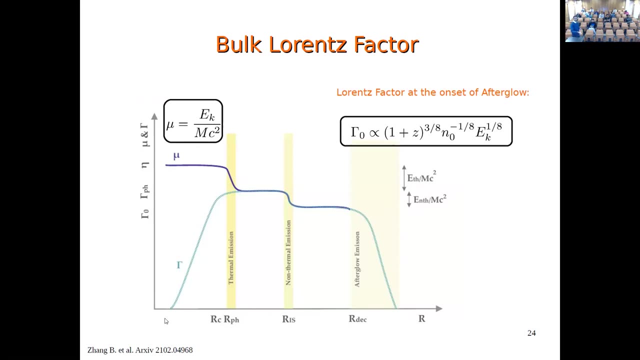 with gamma naught MPC squared. So it will come first to this frame And then again you are doing calculation in this frame, Again, boosted by gamma naught, becomes gamma naught square. OK, So the picture about GRV, the birth and death, starts from here. 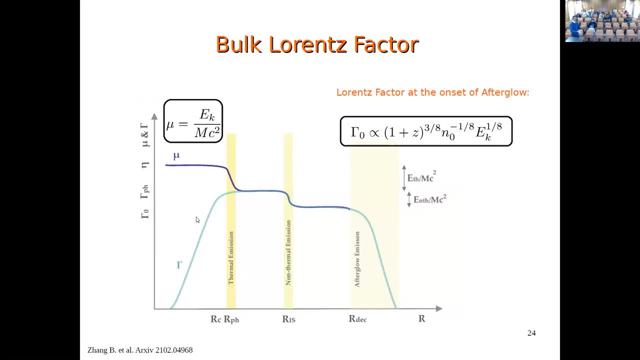 This is the initial trigger And everything like expands relativistically reach to the saturation Lorentz factor. Here you have probably in some cases the thermal emission, And then you have cases where you can see thermal emission into the shock. What is about today's talk? not completely. 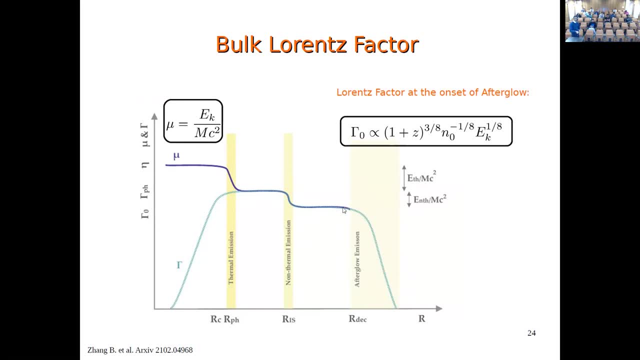 but today's talk focuses here, which is this: starts from here, having a Lorentz factor gamma naught, So this is the onset of the afterglow, OK, And then it evolves and it ends somewhere. here Everything is over. 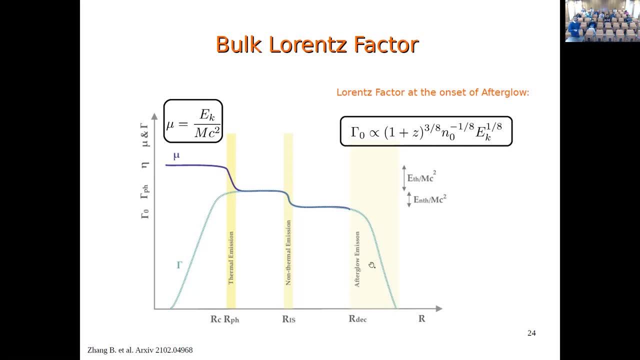 So this is basically the life and death scenario, How we can calculate gamma naught. So in the afterglow models, gamma naught depends at this time on the injected energy from the central engine surrounding medium density and rest of the source. 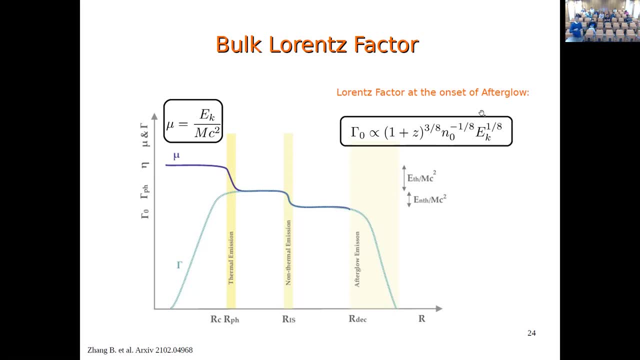 So a model parameter, or basically afterglow model with some certain values of these parameters, can constrain the Lorentz factor here. But the story again goes back here. The whole idea is to understand all these Lorentz factor everything. 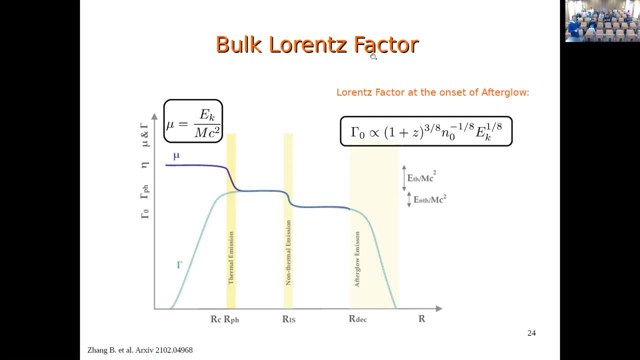 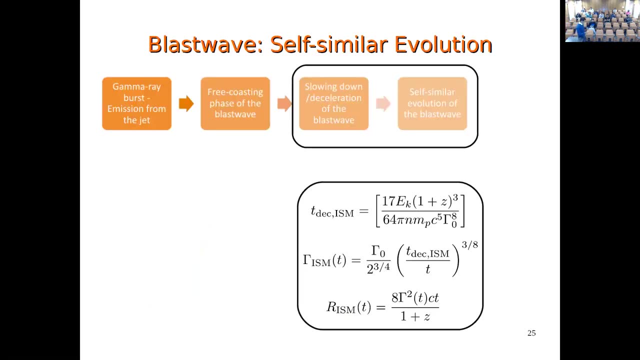 So then one has to combine the prompt emission- So that is something we discussed in the last talk. So how we do basically afterglow calculation. To do afterglow calculation we have to do self-similar evolution. So self-similar evolution is something kind of scaling. 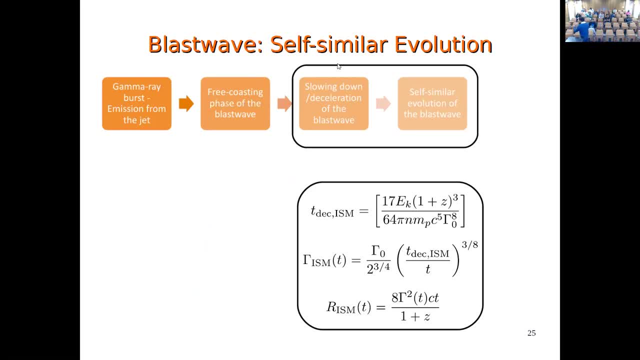 Like you have some. If you have some information about explosion at time t, you can scale it with a power law at t plus delta, d So the Lorentz factor of the afterglow can be written. It can be written in this scaling form. 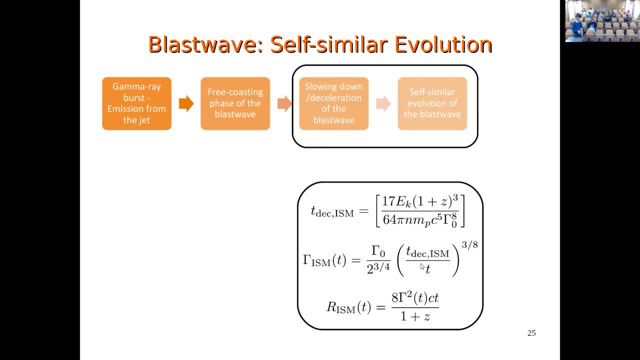 This is the onset when the afterglow starts. This is the time after that observed time, whatever time you want to see the afterglow, And this scaling can be further used to calculate the blast wave radius. This is the shock moving in the ion. 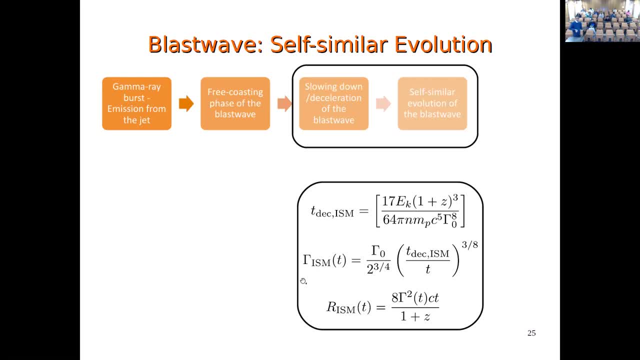 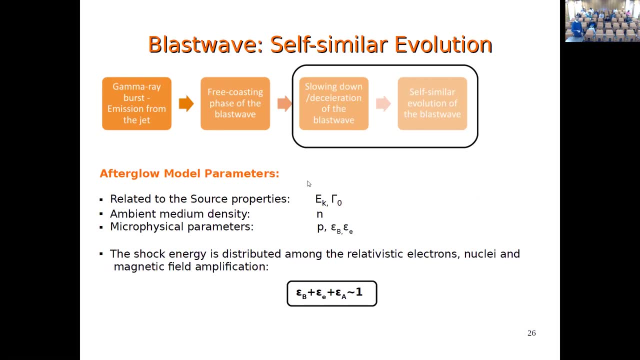 So you have some radius. The time the shock radius will change because it's expanding, And the part of the model parameters afterglow are these: These are related to the source source- energy- And definitely I would say that very late in time. 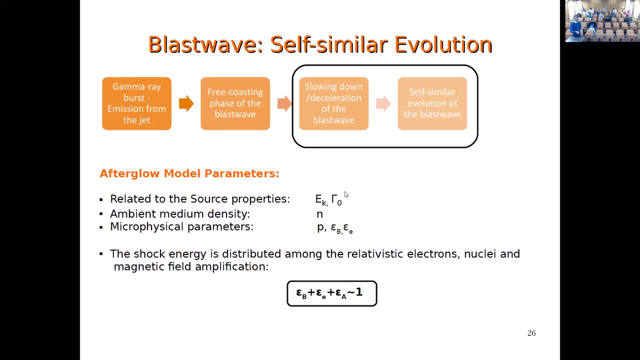 when afterglow, But it is useful if we want to lock it and try to figure out something about the prompt, which generally we want to do, Maybe not now. this is the ambient medium density and these are the shock parameters. so this is the spectral index. 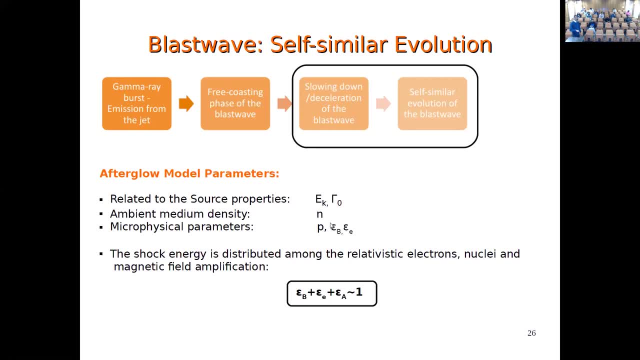 of electrons and these are the micro physical parameters. basically, you have shock and you have shock energy. it is assumed that the shock energy is distributed in the magnetic field amplification. so epsilon b is the fraction of soft energy going to magnetic field. epsilon e is going to electrons. 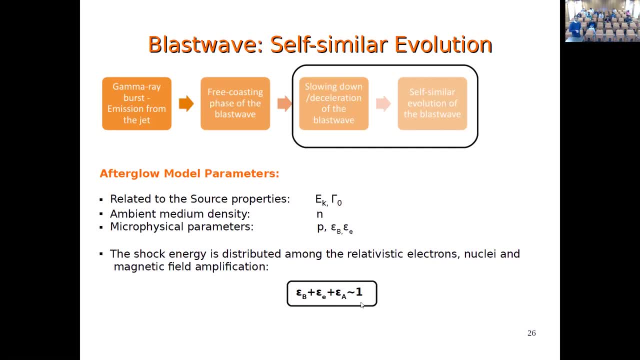 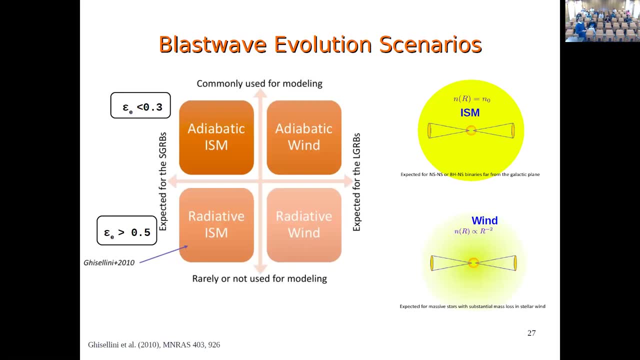 and if there are nuclei like proton, helium, iron, then the fraction going to and the total sum is assumed to be equal to one. and then about the blast wave, you can have scenarios. you can have scenarios like adiabatic and radiative, which you were asking in the last talk. so what happens? like 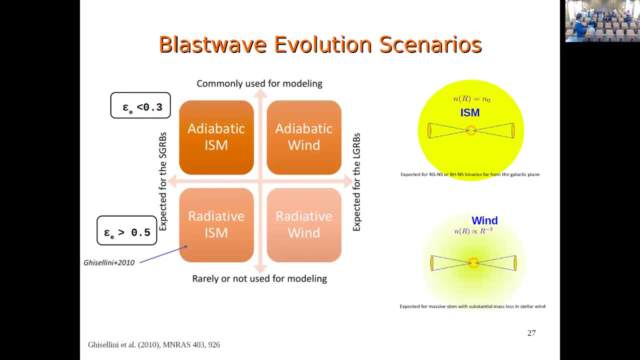 suppose you want to explain some flux f and you have this blast wave and then in the blast wave you have shock. and what would happen in the adiabatic case? you have the energy, just the particles are just getting cooled by the expansion of the medium. but in the radiative case you have 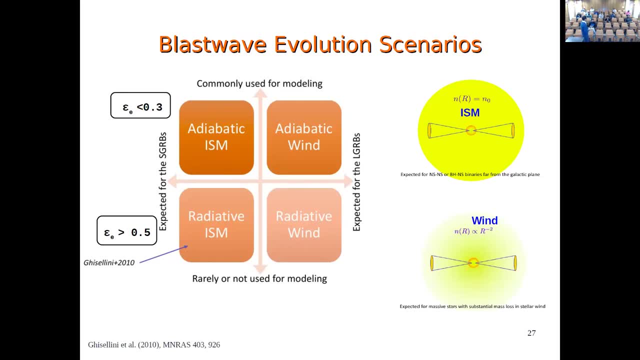 this expansion as well as you have energy exchange with the surrounding medium. so you want to explain the same amount of flux f and you have these two scenarios. so in the radiative case, definitely you have to inject more amount of energy to balance the cooling. okay, so that's why. 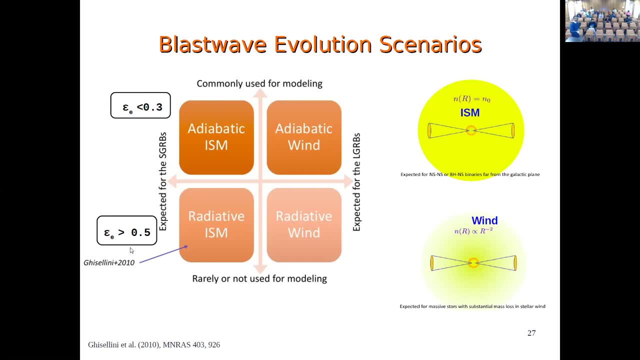 you have these two scenarios: adiabatic and radiative. however, if you see the community, there are very few papers with the radiative cases. okay, the most of the papers are either adiabatic, ism and wind. as i said, the ism will be mostly not necessary, but in an ideal, 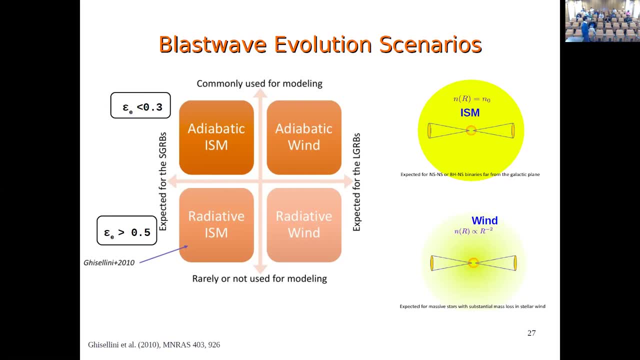 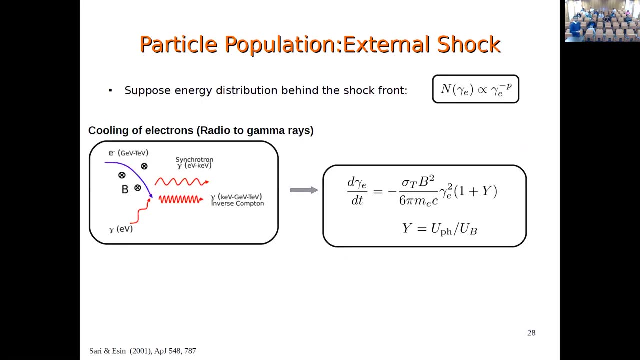 situation would be pretty trivial for the binary mergers and in the wind cases would be like the the collapsor kind of zero pitch. so this, this assumption is for throughout the evolution of blast wave, or this let's say, adiabatic ism assumption is for the prompt emission, or in 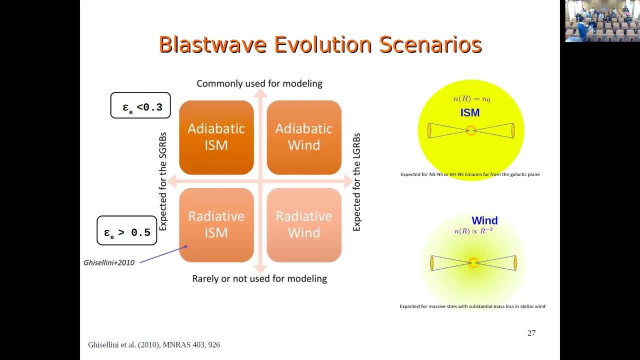 the beginning, but later you switch to something else. no, so this is the prompt emission, is called ism, which is the print emission, which is a completely different part from the afterglow. okay, so what happens? like you know, you have this energy, the internal shock. we don't care, so energy. 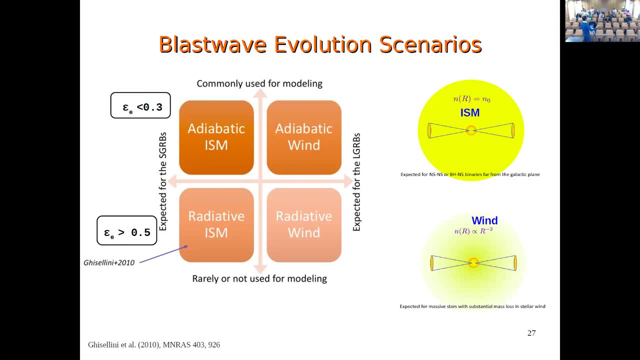 also exchange with the surrounding medium and then at some point you will have the like. you know, the plants may be for afterglow, okay, for the afterlife. yes, it can be for the prompt also, like one can name it. but here the blast wave which i am talking about is this afterglow. this is the 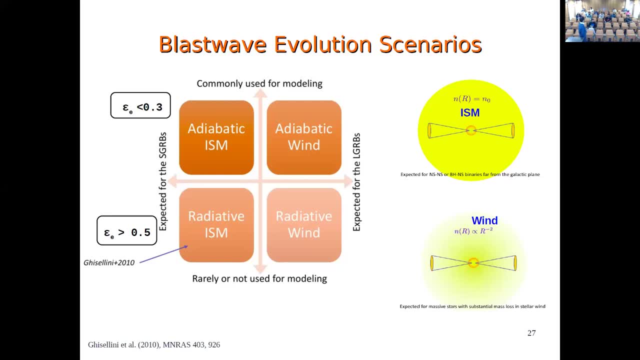 wind medium. here you are telling me that it is only for the medium is further. that's the ideal scenario. okay, then you start doing morning long grps also. the in the larger cases means whenever you travel the larger distance from the central uh portion of the grp, you can expect the ism, the. that's the interesting point. so there are like some. 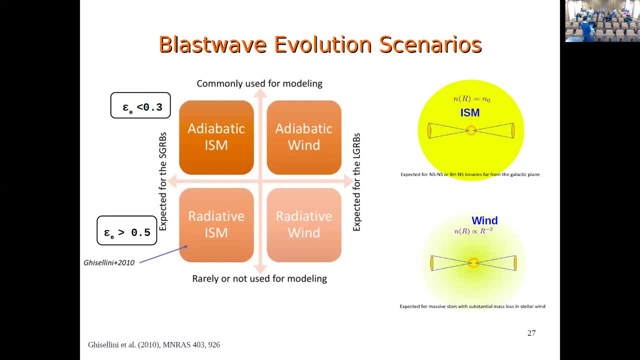 sources. people do model, so you have to figure out like you know when to start the upper globe, like tds lesson, rds lesson. and then you say, okay, you have the wind medium, but up to what extent the wind medium is, so you can do calculations, and then the motivation is phenomenological, like 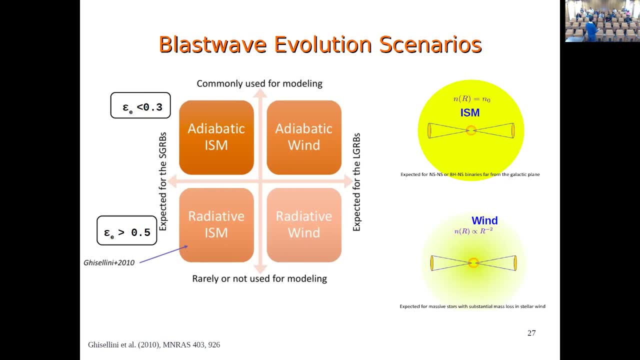 you have to see the observation and if observation can help us to figure out how extent is the wind medium, so that is, like you know, modeling part- definitely at some point it will go to the answer. but how can we? uh means, for that case means if you have two different, different mediums, because 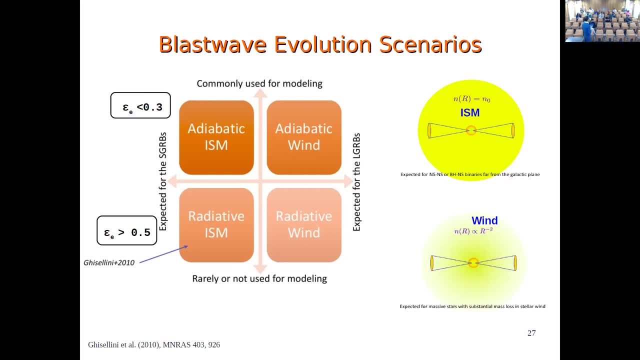 you can expect two different mediums, because whenever you are nearby one uh star, massive star, you can expect some wind medium, but whenever you go to the larger distance you expect some i, some medium. but how can you define this extent means? for different, different cases it will be. 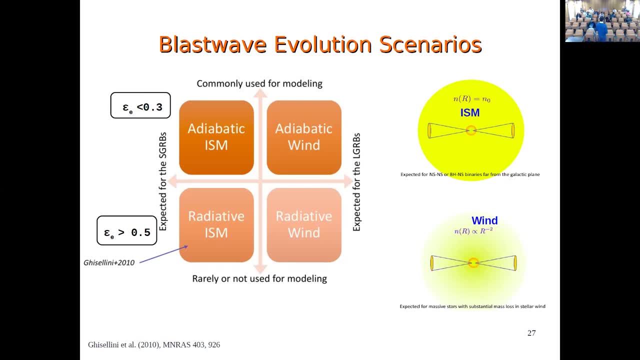 different because so, as i said, like it's completely motivated by the data. suppose you take a wind model and you start modeling your data. okay, you see that. okay, you put all the ingredients of the model, like jet break, you know, breaks of a cooling break, tm, all these things, and at some point you 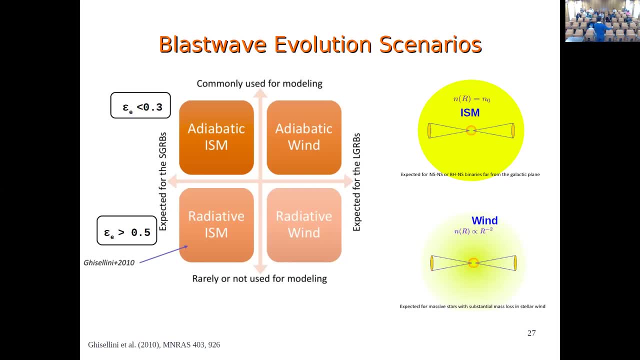 see, everything is explained, but the, the, the observation, they departure. okay, then, what you want to do? you think that, okay, let me put an ism and check, uh, uh, kind of. we put the density, like you know. then you have to update your model with this. yes, 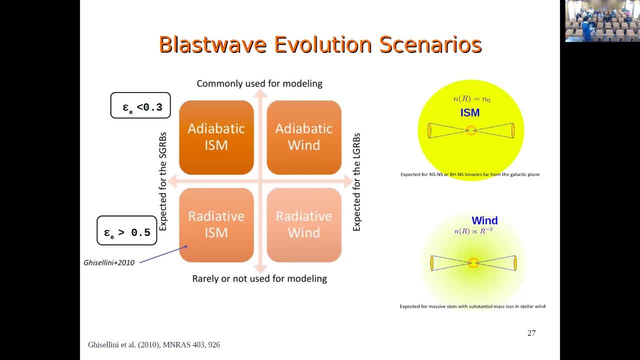 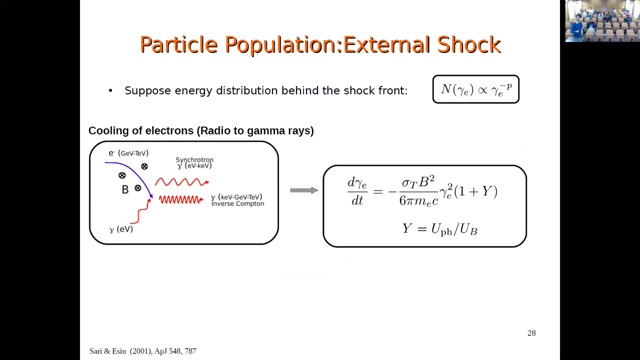 update your model. so. so there are papers, like some paper by freya where he did, i think, for this, 1901, 140 or maybe some other jr for 1929, yeah, so they have this green and then they go to the ice. so, yeah, so coming to the non-thermal particle population calculation, 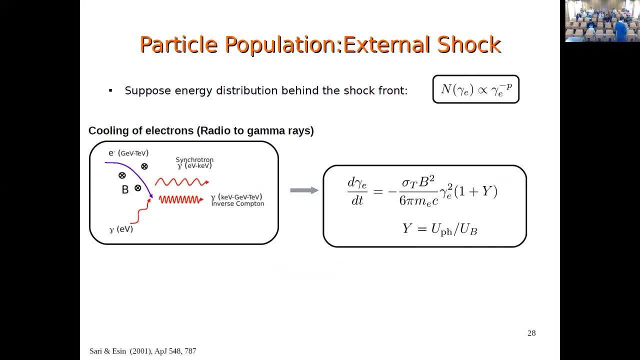 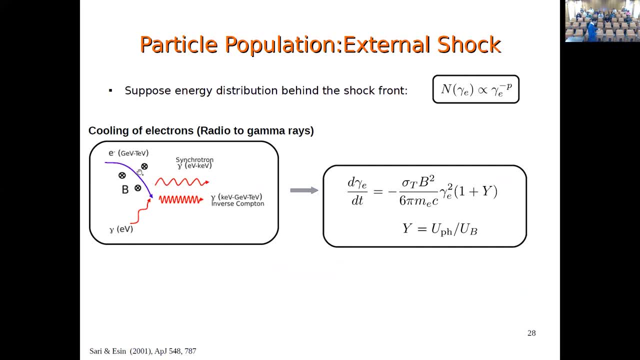 magnetic field. both are getting, like you know. electrons are getting accelerated, magnetic field is getting amplified. so what would happen is you will find uh synchrotron photons and then these synchrotron photons can be up scattered by the electrons of the medium. so you have 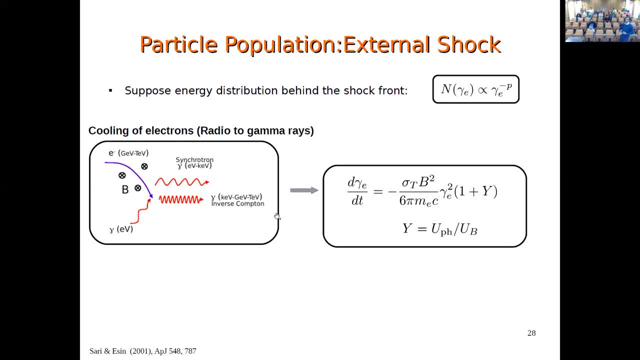 definitely a broad bandwidth spectrum which is useful, uh, for grb and, in particular, cases like the. the idea, or as well as the substance, is that this model is working, at least for the synchrotron self-contained in grb. so what we need to do is we need to solve this equation, which is the how much? 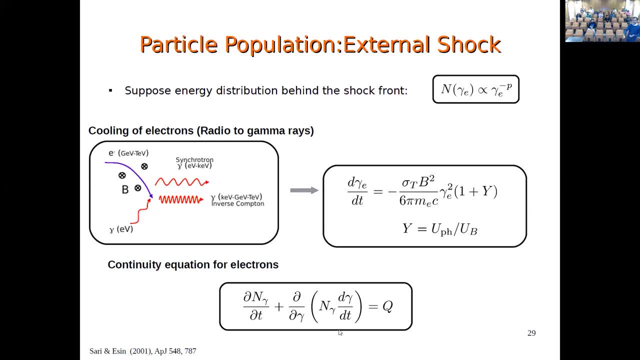 what would be the population of electrons in the shock region having the pool cooling stuff by magnetic field which is like magnetic b squared. the y is a parameter which is involved here, because suppose you have a two channel of cooling, synchrotron and inverse compton. 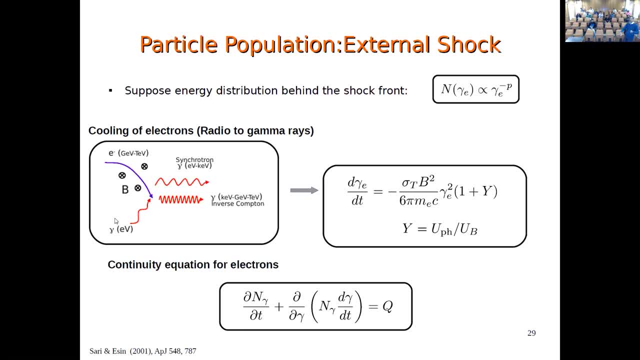 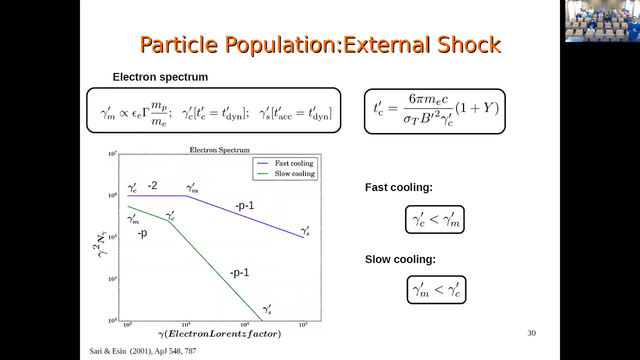 then the inverse compton is driven by the, the photon density. so y zero, you have only magnetic field cooling. y have some value, then the photon, target photon are also important. so we, we put these two coolings and then now then we find two scenarios. uh, we have two kind of populations of 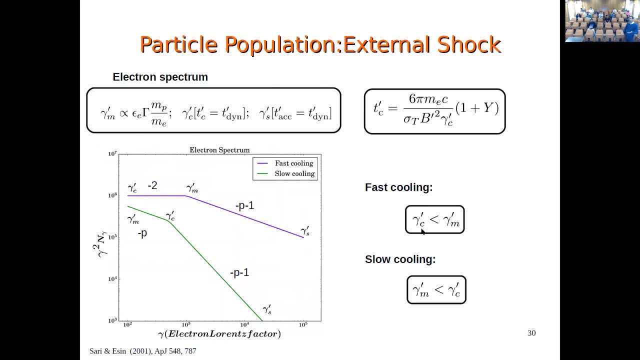 steady state population. one is the fast cooling, where the cooling orange factor is less than the minimum orange factor, and then you have slow cooling where it inverses and what would happens like physical picture of fast cooling is like you have a dynamic time, so dynamic time, like you go instant of time and you see the blast radius. so that will be live for. 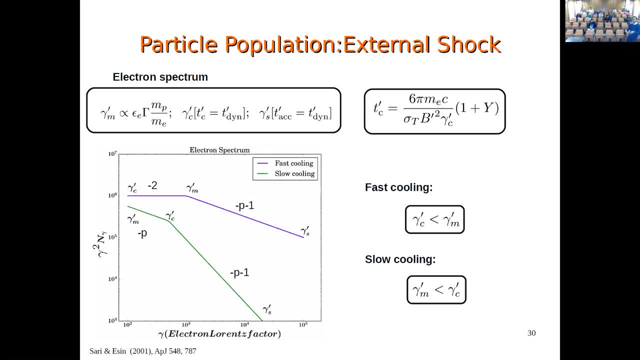 a given time and then in that particular time you have to check what is the cooling time and stuff. so you, in the fast cooling all the electrons are cooled, but in the slow cooling only this component will be cooled. so slow cooling is when we do the detail calculation, like the feedback effects. 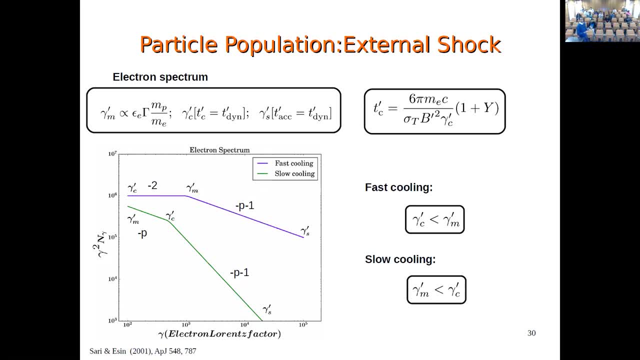 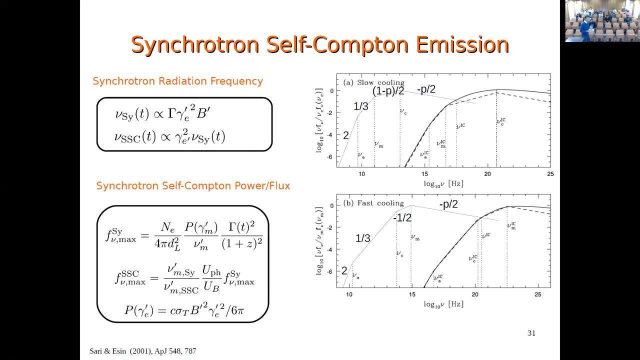 of thompson, scattering and everything is easier and we can do this. so the fault is that when we do the flow calculation and we talk about the flow, this is the conclusion from the plot and it will be easy to understand when we are calculating the flow, because we can. do that when we are doing the flow calculation, then we can do that. but in the slow cooling source you are talking about a very specific energy flow and that means we will have a very specific current that will be very parametric in relation to this slow cooling emission and most grv, generally the afterglow. can be explained by the slow cooling emission. now again to go to synchronous help and calculation, one has to. so we we know that we have an electron spectrum having these breaks, gamma and a gamma c, and as well as we know that the power radiated by electrons depends on gamma e square. so we can find any spectrum you. 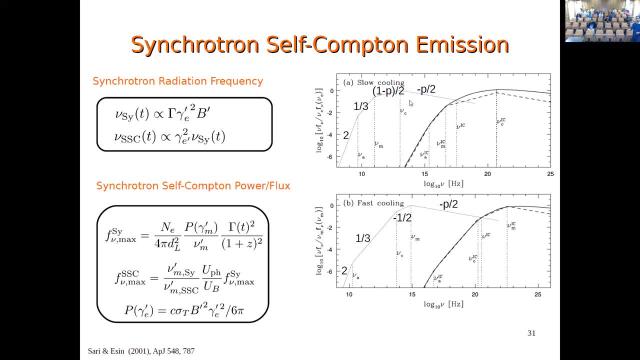 component. so this is the component synchrotron part and this is very analytical approximation and because it more or less matches with the numerical, other than that in numerical you won't see these breaks, but the flux-wise it is more or less okay approximation here. I 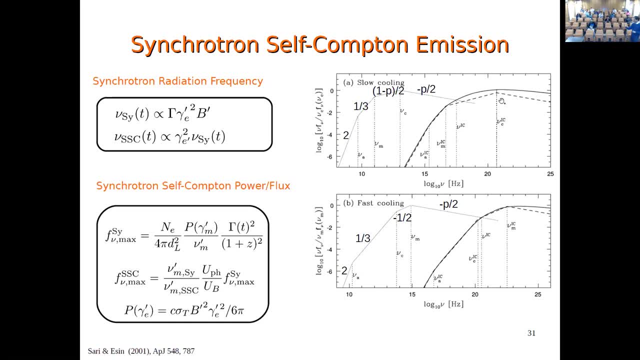 have shown two cases for this. this is the ssc part. one thing you can do that. okay, you have the synchrotron spectrum and analytical part. just do a mirror of scattering by gamma and square, which will give you this component dashed line with the similar kind of scatter. 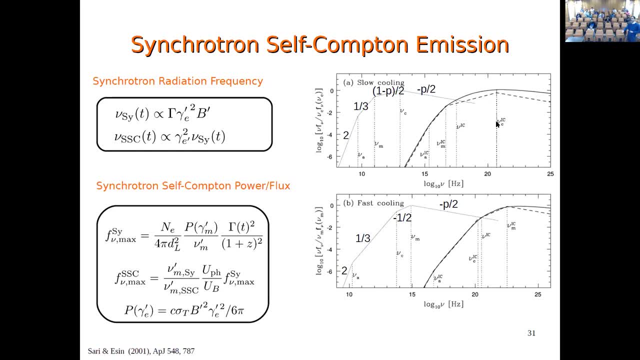 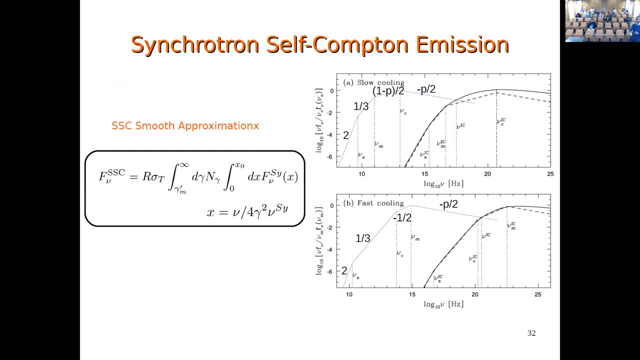 frequency here nu c. you have nu c, i c, which is gamma square. this part, gamma c square, nu c. so this is the analytical approximation one can do, the smooth approximation, which is more reliable, not reliable, which basically considers all the interaction between the photons, target photons and the electrons. so 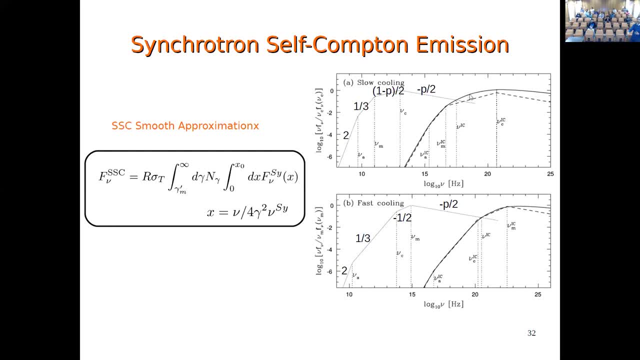 so one can basically use either this or that. but yeah, the smooth approximation is so the, at the lowest standards, the spectral slope of two. so what gives? is it the synchrotron component or something else? so this is the synchrotron self-absorption point. so self-absorption is uh high by two. 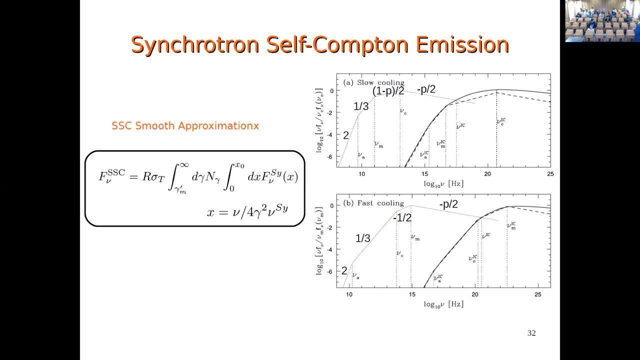 and it's 2.5. ah, okay, so because now i was confused, i am confused. now i am confused. no, no, that i agree. so now i am confused because, uh, i remember that people also talk about this thermal component in the grb right, that blackbody component. 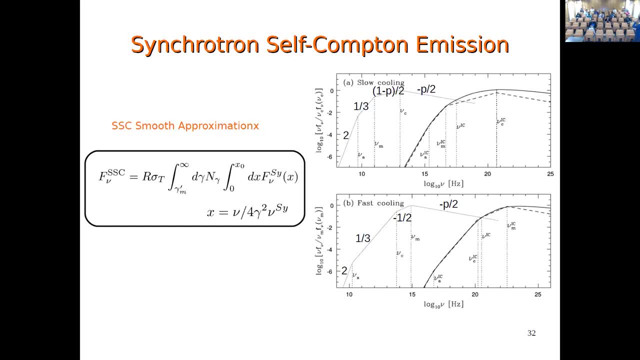 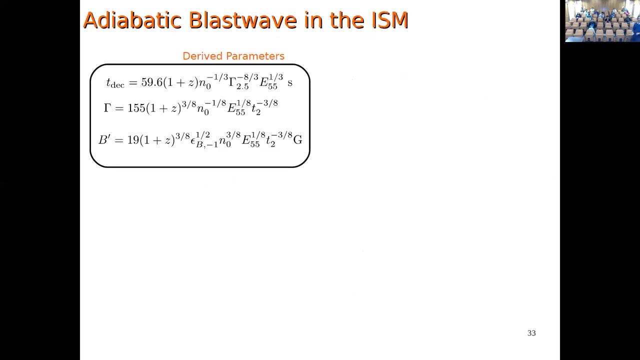 and that has a two power law. i mean that will be into two power of two that body. okay, so you don't see in the end. okay, so now to do the after glow calculation. we need to. definitely, this is the onset time. it depends on the parameter here, like the density law inspector, the injected energy, and we can. 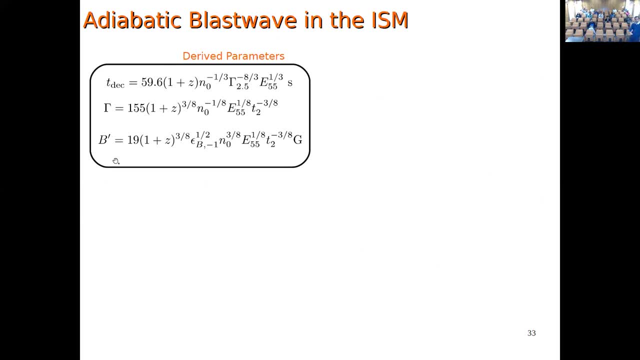 calculate all these parameters and once we have a slide, everything is moving like magnetic field, evolve with time and the law inspector relaxes that. we are doing the same thing. here we have a factor will also evolve with time. so we can calculate all these parameters and based on that, 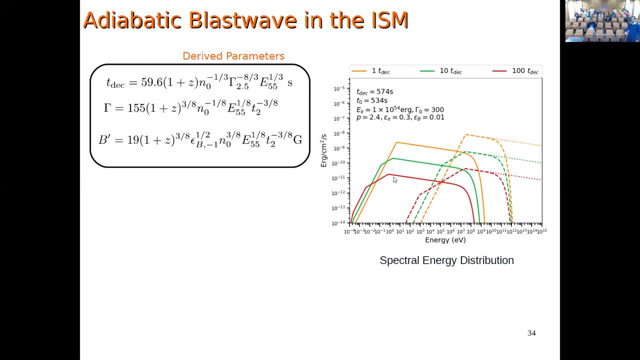 having the having some input parameters, we can have this synchrotron part and the ssc part. for just for simplicity, everything analytical here and the cutoff to the synchrotron comes from the maximum synchrotron energy. so we can, we can, based on the shock conditions, we can calculate the 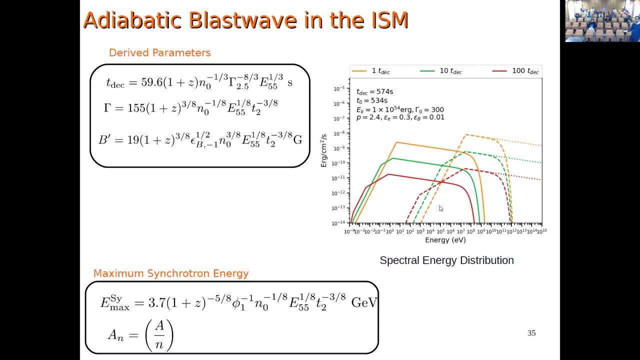 maximum energy of synchrotron photons. so this is the cutoff here, shown exponentially. here the cutoff. basically it can go forever, but from at least under the r20 electron volt. but all these high energy photon teb range, they are absorbed. so we have to put the reps dependent, or maybe source. 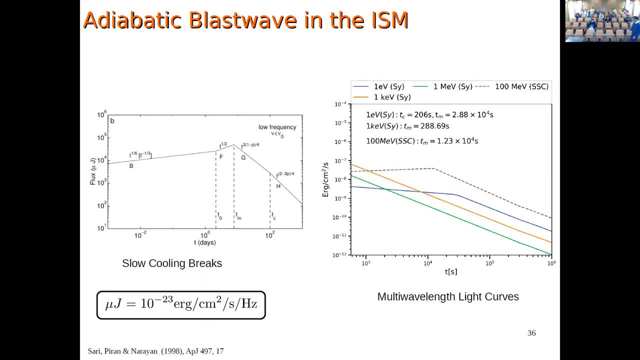 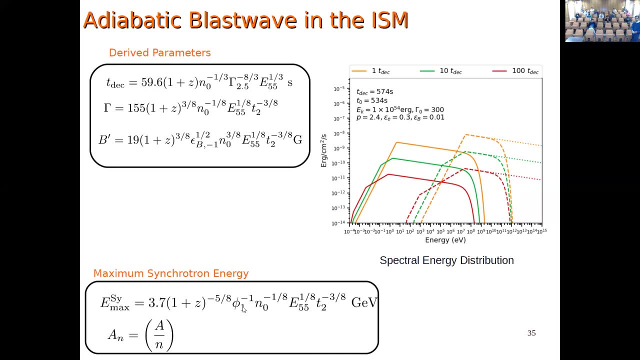 dependent cutoffs. uh, the maximum synchrotron energy should be also depending upon the loading factor. yeah, yes, yes, so this is the okay, so this is the. oh, you see, like more or less not, uh, not actually not depending here, but whenever you consider the energy. 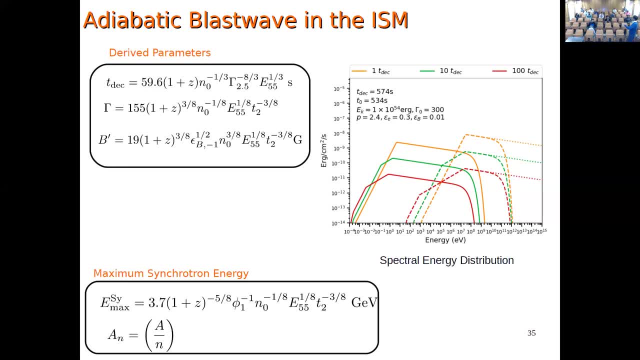 there is some. yeah, that's the boost. like you have e prime and then uh, the observer energy is common times e prime. that's the boost of energy from one frame to another frame. so when you do this calculation in the uh, in the short region, it looks like it was in terms of the different. 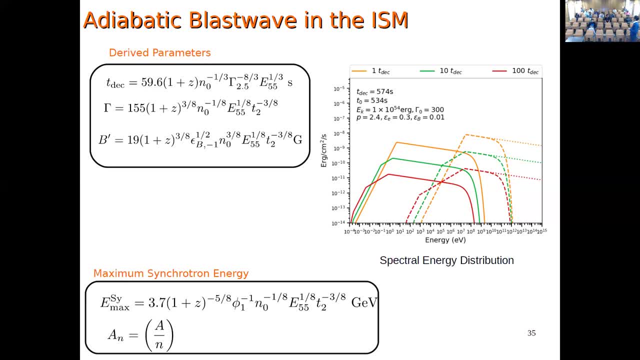 different grgs. you have different different loading factors. yes, okay, yes, that's the bulk orange factor. yeah, the workload, so the maximum synchrotron energy, as far as i equation, so it is somewhat depending upon the, uh, lower infected background factor. okay, so i don't. 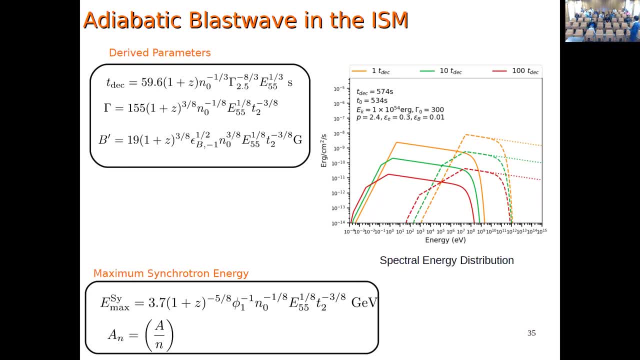 have the calculation now. but what you do? basically you calculate the saturation orange factor. yes, so you have this acceleration, the time of electrons. so it's a short property. uh, not sure how i connect it to the gamma belt law inspector. but what happens? like you have this acceleration time, 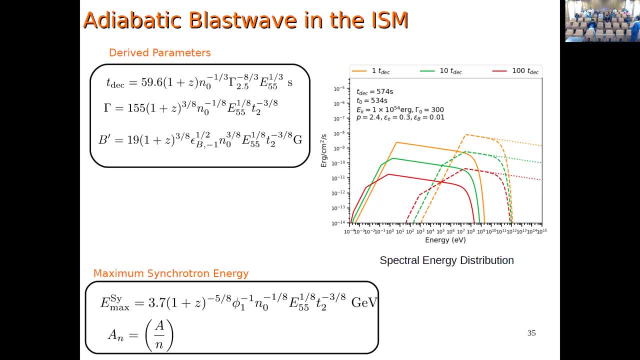 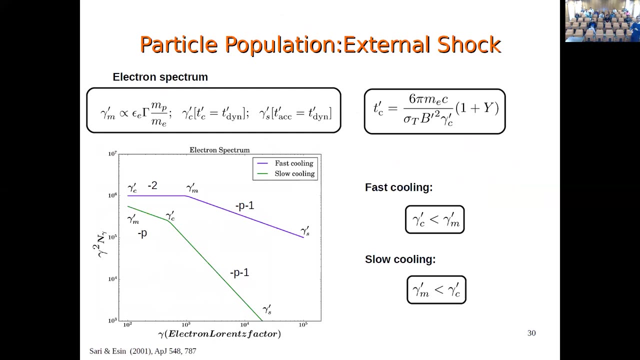 scale and you have uh, the uh, some pieces. this would be not cooling the acceleration time. you said: just let me turn. okay, i just missed the point. so yeah, so you can basically calculate the dynamic time. so dynamic time is, uh, the time i said. like you know, the blast will last will be, uh, be lying for you on for a given instead, so that we know. 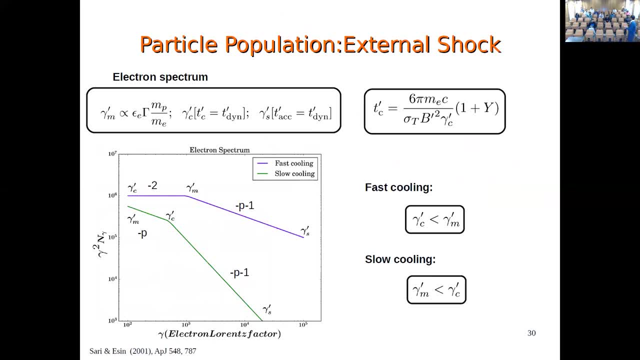 each dynamic time just r, gamma, rc by gamma, or just the observer time. okay, and the solution time is uh, i haven't uh defined here, but it depends on the shock problem if you want to see, is on the. so this one, that the maximum synchro front that you have written, this is the absorbed one- are in. 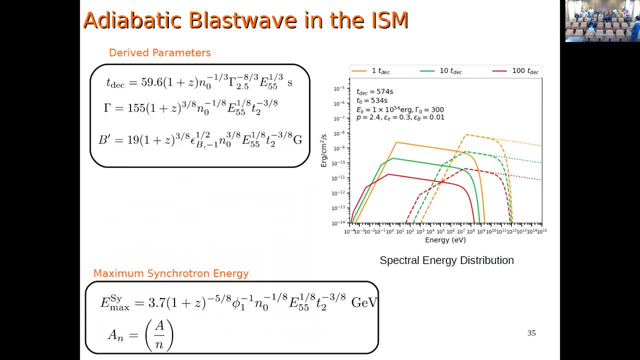 the frame of the soccer, something this is to show if you are not working on the curve. but let me write this thing, okay, so we can start with your data. so this is the max Han's Шаг. This is the observed one. Yeah, this is the observed one. 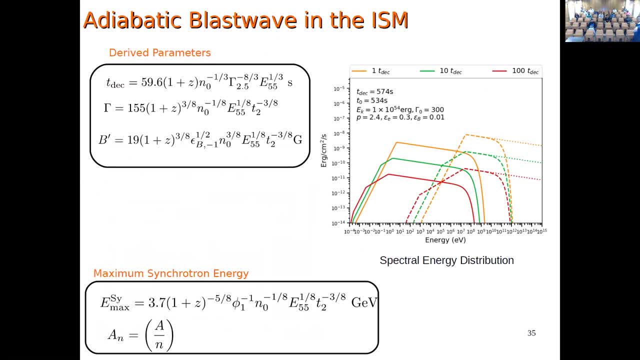 That's what this spectrum is. So what I was like here. what I'm showing is the observed spectrum, So observed cutoff and all the parameters for the maximum energy are defined here, And also by the time you are calculating this. 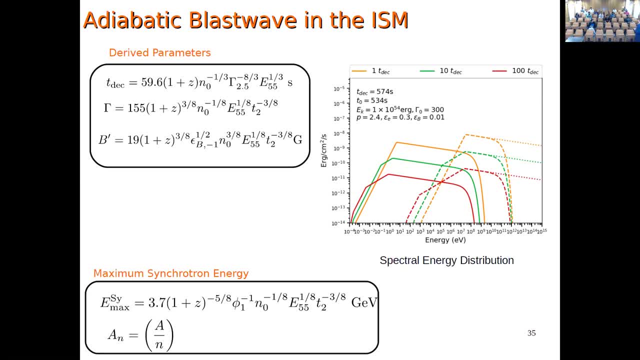 does one have already reduced coagulation? It depends. It depends on the time. Like these three curves, if you see, like the first one is at the desolation time, which is 574 seconds. So the first one, the orange color. 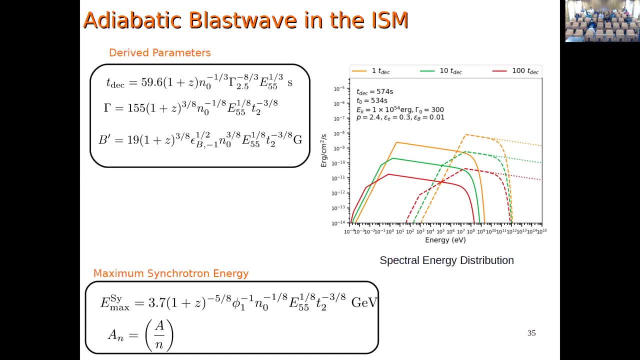 So you have the cutoff like around the gamma naught is like 300.. So I think for T desolation gamma will be around 100 maybe, And then if you go late in time it will be like 10 or once. 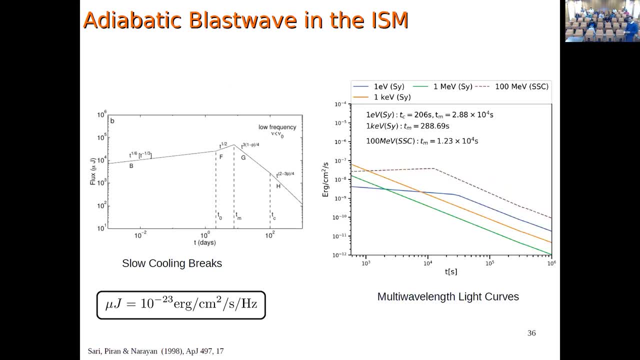 So yeah, So the first thing we can calculate, we can calculate is this, which is called spectral energy distribution. The second thing is we can calculate the light curves, How a particular frequency, like you see X-ray, or One minute. 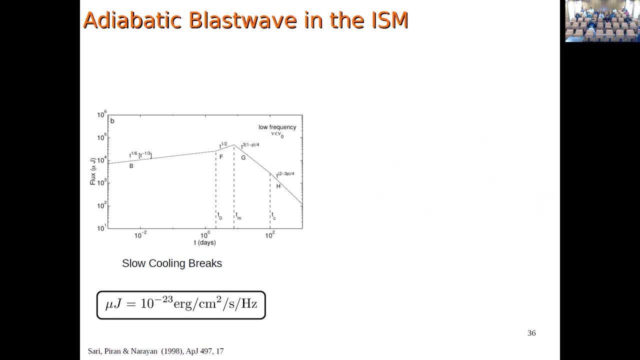 Okay, That was enough. This is Okay. But Okay, I have to do this really fast then. So the light curve: basically, you have a particular frequency and you have the light curve And you can see all the breaks. 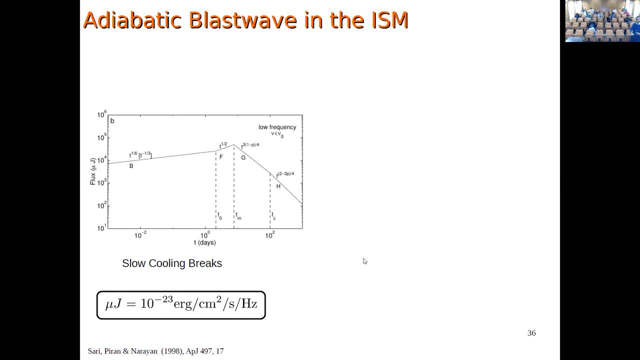 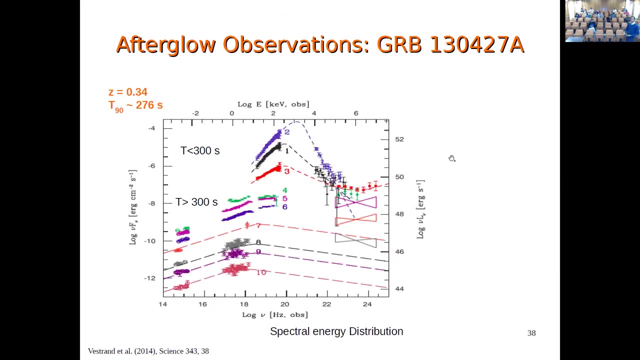 Okay, So you have the cooling frequencies, corresponding cooling breaks, And. But in the real picture you might see one break like, for example, 100 MeV. you just see the TM break. So you might not see the whole picture. but it depends on the input parameters of the model. 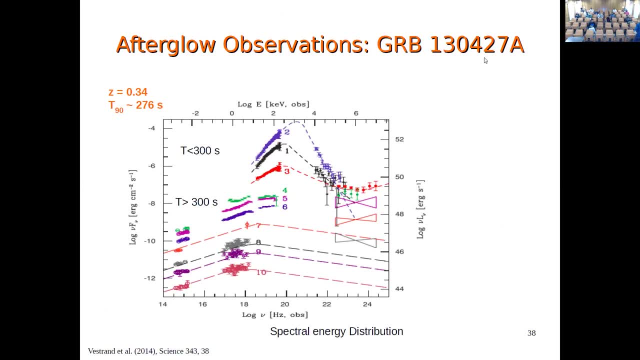 Here I have just shown the picture, like for this GRP At least. I want to finish this part because I could also ask these two GRPs. So this GRP, if you see, having T90, 276 seconds. So this part, we think that it's prompt emission. 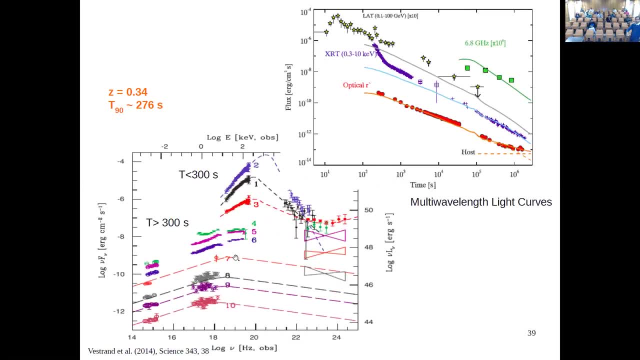 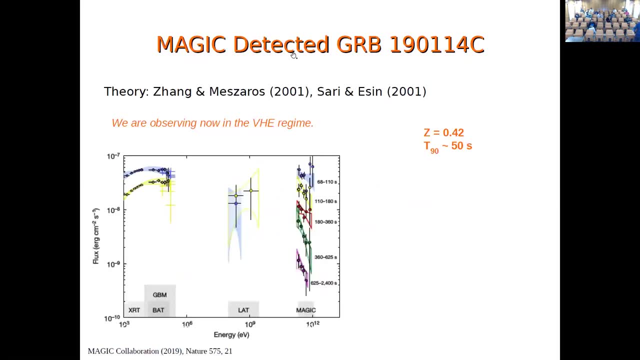 And here it saturates. the afterglow, The light curve are also shown here, which is like in this part, And only you have the prompt emission. I will compare them. just Let me put this: another GRP. This is the first GRP in the TEB component. 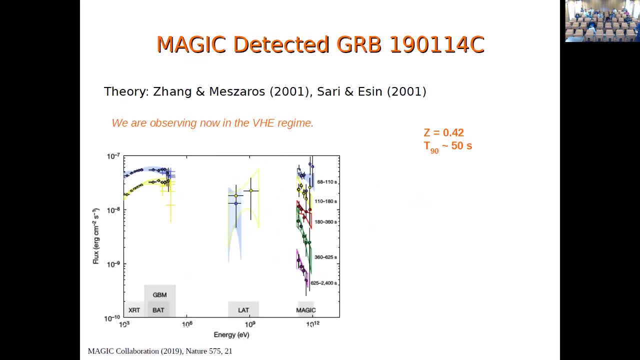 The TEB component appears at around 68 seconds And then, it was well observed, till 2500 seconds. Okay, And one calculates the maximum energy. what can come around 50 seconds? The gamma is around 100 to 500.. Again, depends on the input parameter, what gamma node you start with. 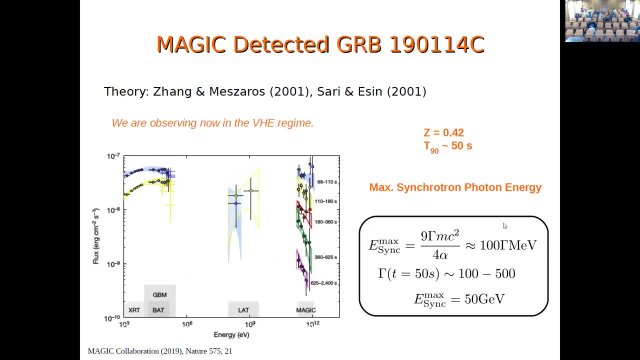 That's why I am telling that the maximum synchrotron energy, the 100 gamma MeV. So No, this is the boost, The boosted one, This is the boost. This is like you know. it's written in a different form. 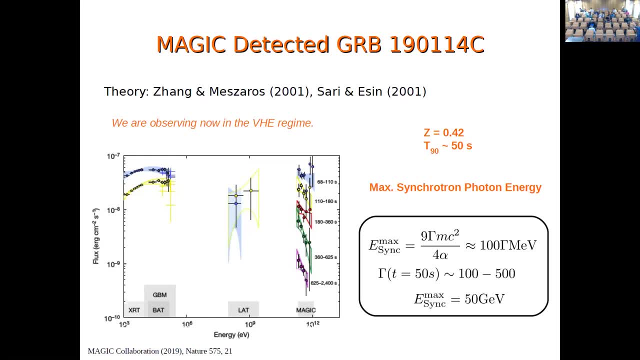 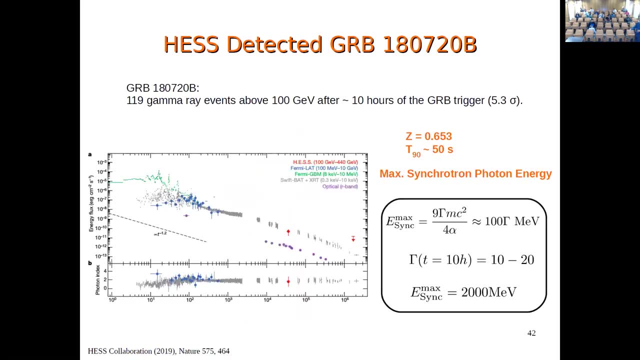 So this is Despite the- I am not sure, but it might be- co-moving plane to the observable field. Yeah, Kind of that. So So, maximum energy, you will find synchrotron very, very less. And then one needs something. 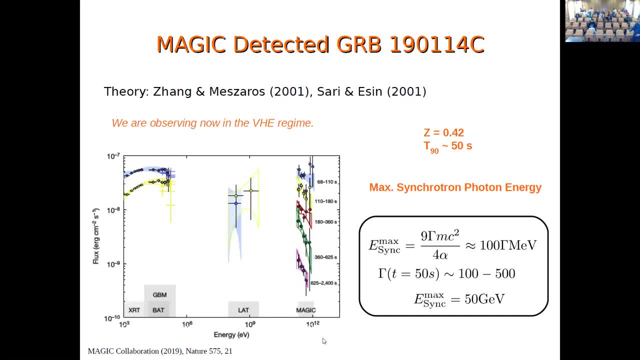 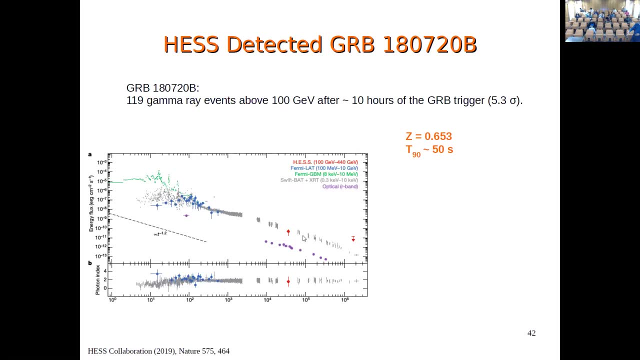 Here it is 50 GEB, But you see photons around sub-TEB or TEB photons, And it has detected this- another GRP in TEB 10 hours after the trigger here. So this was the second GRP Again. you need something different to explain all this. 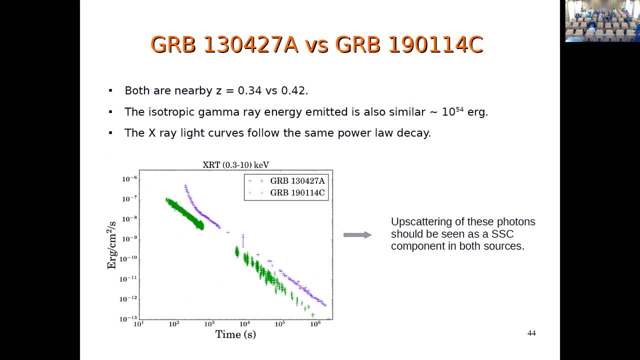 If you compare these two GRP light curve in XRT they looks very similar. I did not do the eject putting them on the same redshift kind of calculation, But more or less the X-ray light curve, they have the same features. 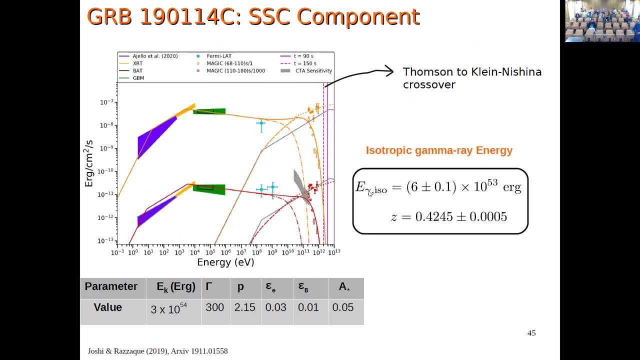 And when we model the SSC emission, at least for the first GRP, this one. So this is the synchrotron part here And here is the. So this is the EBL corrected photons And these are the EBL absorbed photons. 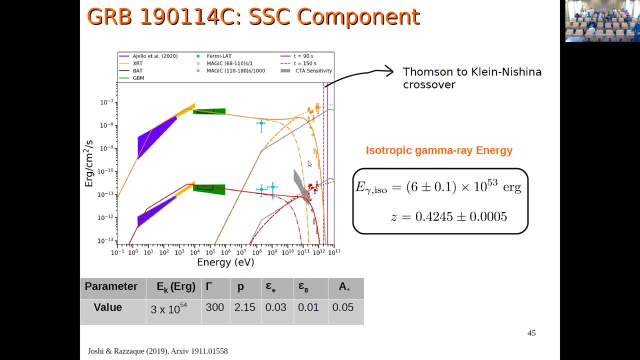 The model fits here And, as you realize, we correct it here, the EBL corrections. The second thing is when we do the feedback. So what can happen is like: In the system the electrons can cool either SSC, Thomson scattering or clan Isina. 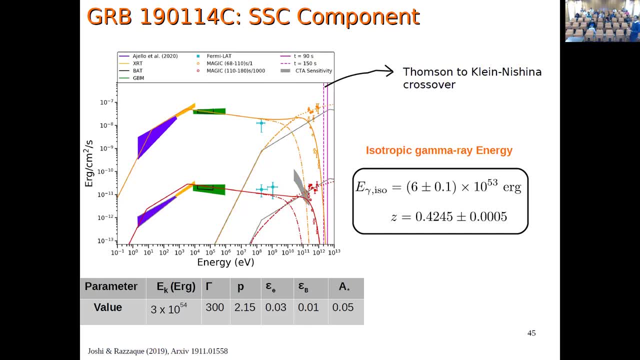 So clan Isina? the cooling is less effective because cooling depends on just gamma, But in Thomson it depends on gamma squared. So these effects are important, At least what we're finding here, that in this source the crossover to clan Isina comes somewhere after the magic data points. 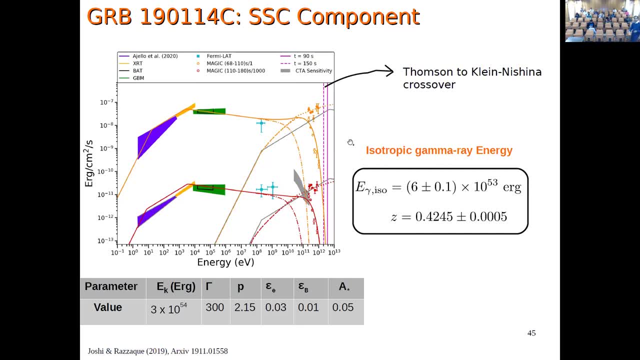 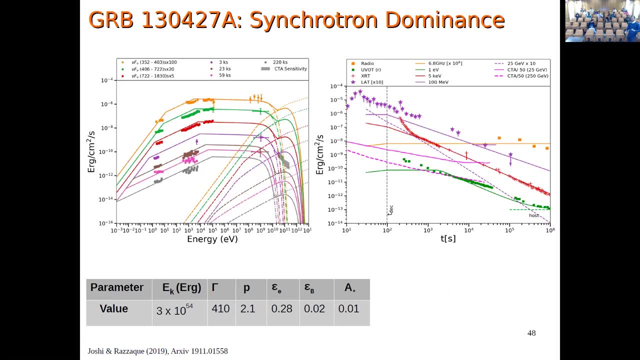 So we can explain the source with using the, The Thomson scattering. And yeah, I will not discuss in detail, But yeah, the same model can explain the light curves About this. GRP. GRP 13-0427A- all of the data can be explained by the synchrotron. 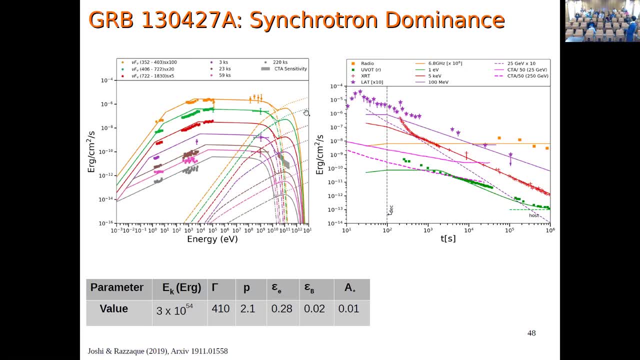 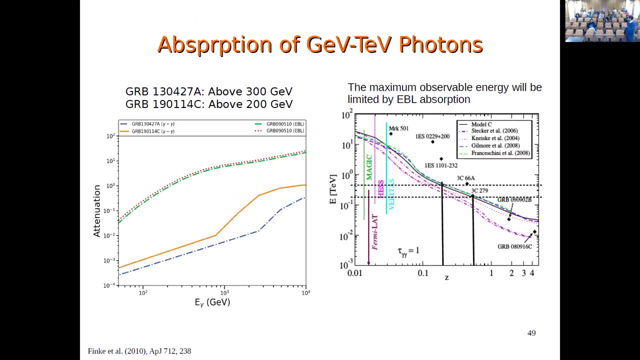 And we don't have any component here, even though both GRP looks very similar. So that is, I don't know why it was missed. So how much time do I have? Three, four minutes, Okay. So the second option about GBTV detection in GRP depends on this EBL attenuation plot. 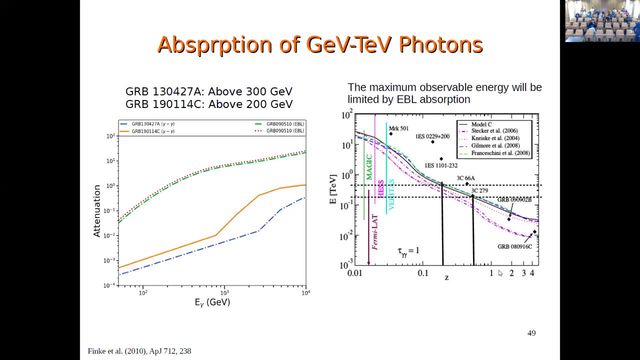 We know that as the redshift increases there is a limit. The maximum energy can come from a source. So it goes like if you want to see photons from a source above 100 GB, then the source has to be in redshift less than one. 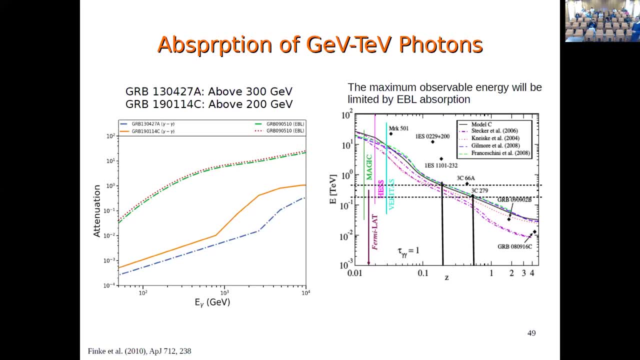 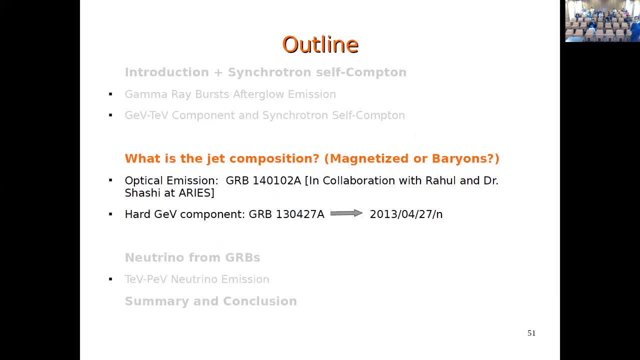 So I think the future of the CTL telescopes will discover how many all these sources exist within redshift. less than one. Okay, So I have. I can just give some hint about this reverse shock part which I did here with Raoul and Dr Sasi about the jet composition, if we can model the optical emission with the reverse shock or not. 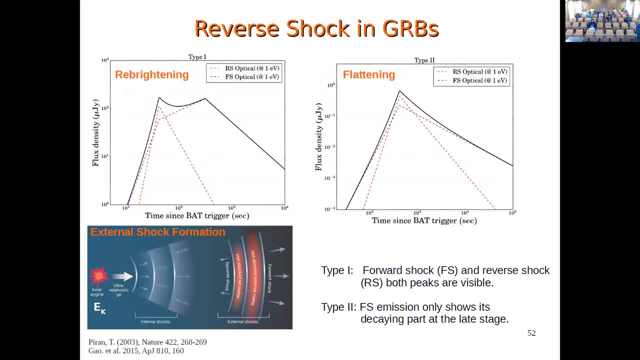 So we know about reverse shock, As I discussed like, once you have this shock formation, the forward shock is formed TDS lesion. The shock is also like deaccelerating, So there is an impact to the In the backward direction. 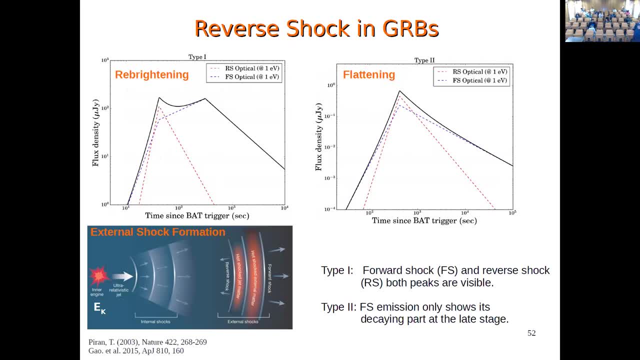 The shock, Reverse shock creates reverse shock, moves to the direction of the jet And the feature of it are two. You can see here like rebrightening occurs. This is the reverse shock, the first peak, and this is the forward shift. 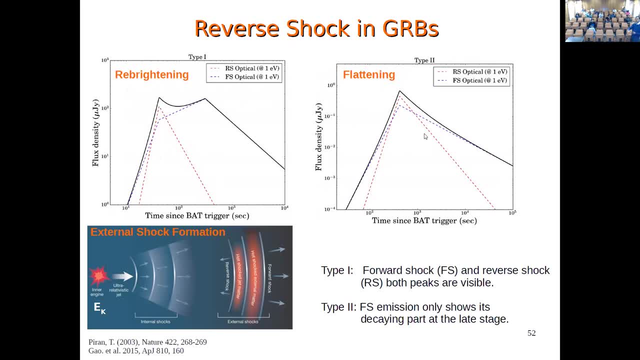 So if we see this kind of data, we can say, okay, this is rebrightening. Here you have the peak reverse shock and then no peak of afterglow, but the later time the forward shock is actually dominating. So we found this source. 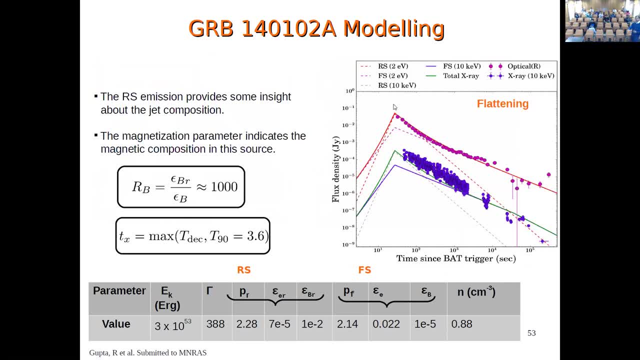 So we found this source where we can model this optical emission. only in time with the flattened And we see the later time, the flattening. It gives us the model parameters And in first it indicates the magnetization of the jet is around 1,000. 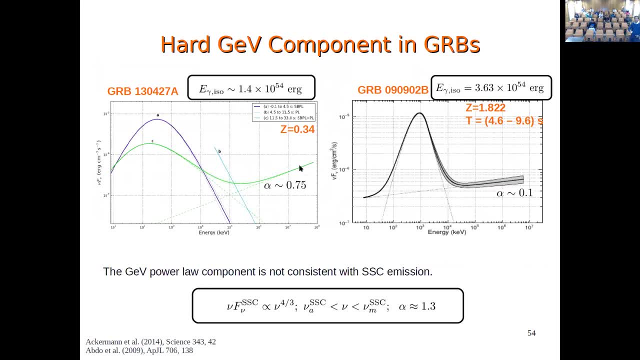 The second part I want to just Before I finish. I want to discuss here, like in some of the GRBs- at least in this 1304, 0909,, you see this component And if you try understanding the index, it doesn't match with the SSC. 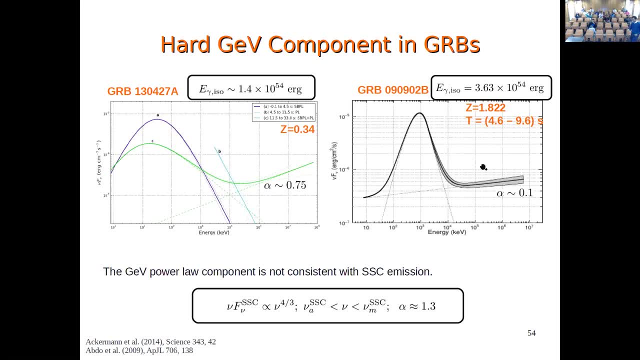 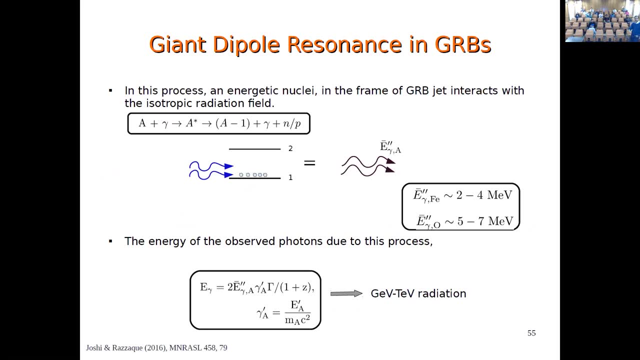 Then what can happen? Can we figure out some composition of the jet? We tried this model which is called the. Suppose the jet is loaded with the iron nuclei, You can have some interaction- iron- with the target photons available in the source. 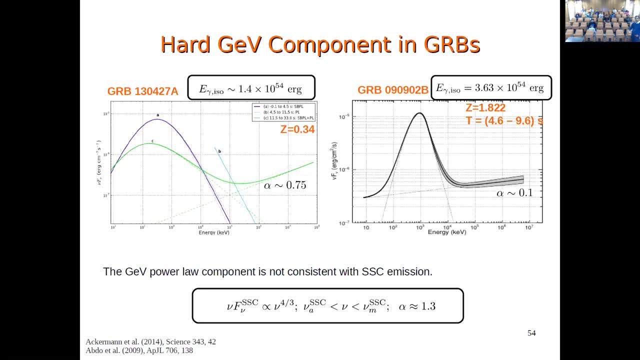 And here the whole calculation is not in the afterglow, This is only in time. So what I assume is: I assume there are iron nuclei and they interact with these target photons in the time Duration somewhere 4.5 and 11 seconds. 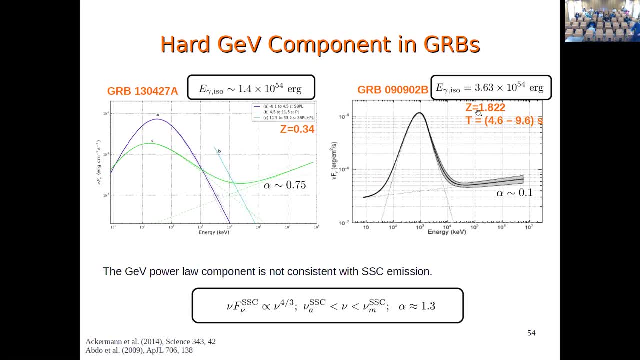 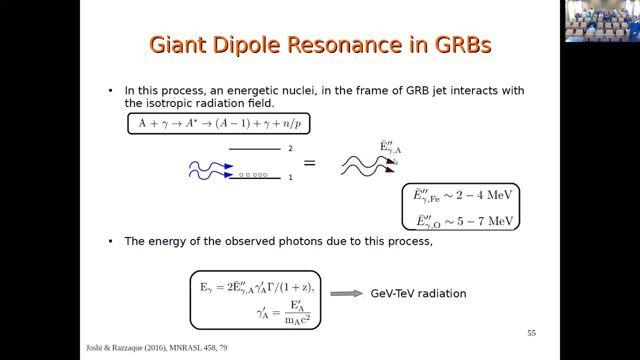 So this is more or less close to the prompt emission part And we So in these reactions we do get these gamma rays in the rest frame of the nucleus And then we convert them. What would be the energy on the other frame? 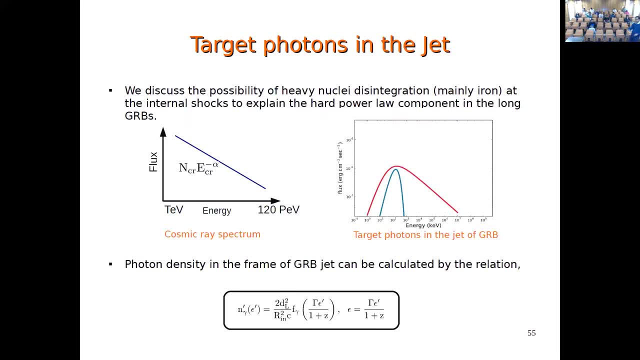 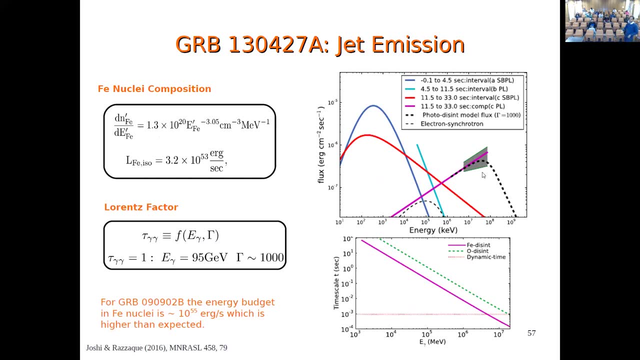 Doing all these calculations, you will, And this is just the interaction target: photon and nuclei. What you can find is the phenomenological model. again, we assume that there are iron nuclei- It is possible in some cases- And one can figure out what would be the maximum energy observed from a source. 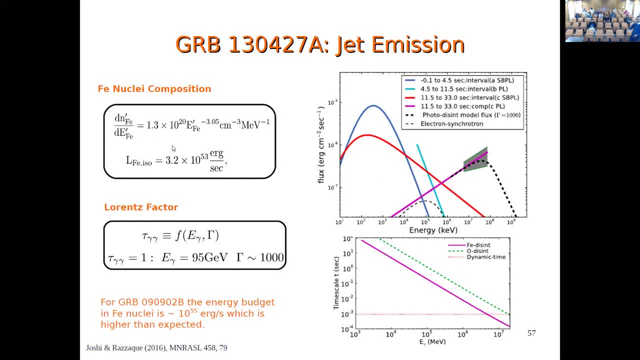 That can give us constant on the Lorentz factor And as well as give some idea that, okay, if this kind of components are This kind of target distribution seen in a particular GRB. At least we have one example here. This tail is very, very important to do the photodisintegration. 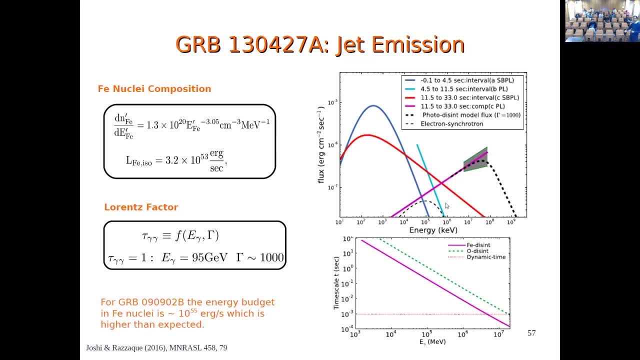 Because we have large energy of target photons And that can be used to do the GDR process. So the second GRB: we check we don't have these tail emissions And we found that the luminosity requirement to explain any of these power law components is really really high. 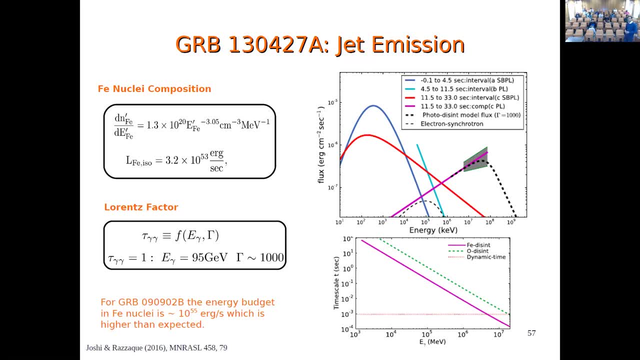 So it's not very, very, Very, very like. Okay, so only one source: The model works. Okay, I will stop here, Thanks. Okay, let's end the week And It's an interesting talk And now we can have some questions and such. 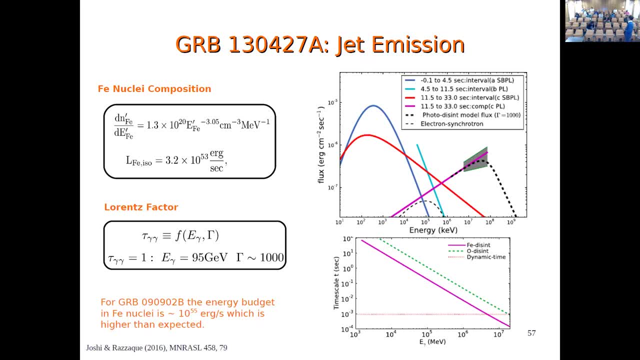 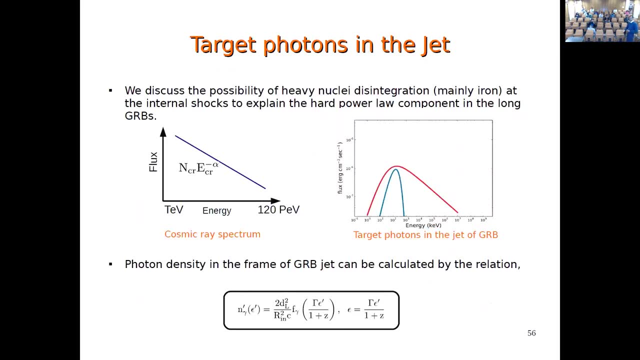 So I couldn't understand the What is the necessity of Adding this item? UTI here means I just missed these two. Okay, So what happens? like you know, You want to explain this component? Okay, In this GRB. 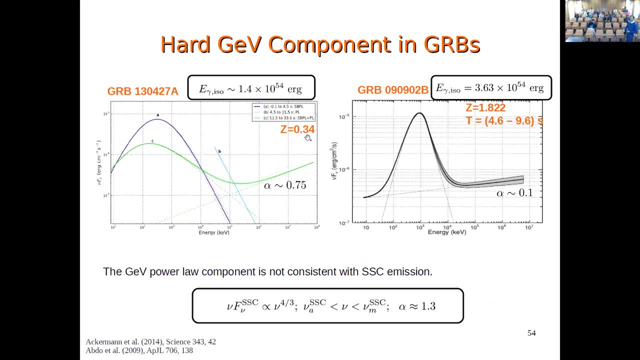 And it was found that the synchrotron model definitely could not explain it Because it again reaches the maximum limit. The other options is: The first option is inverse compact. The SSC People did that And what we found is like people. 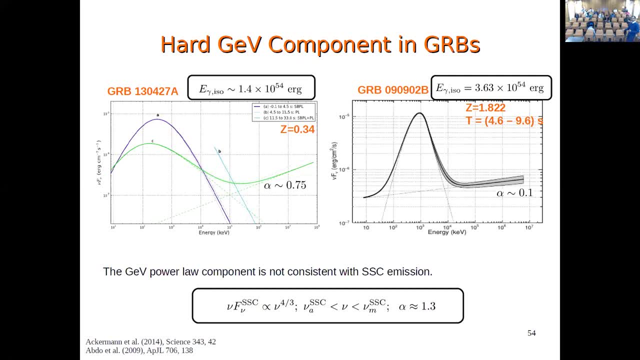 Okay, Already. That's why we checked the calculations And The index doesn't match with the index of any kind of. If SSC was there, then the index alpha should be around 1.3.. Okay, It was not. So in fact, there is something different going on. 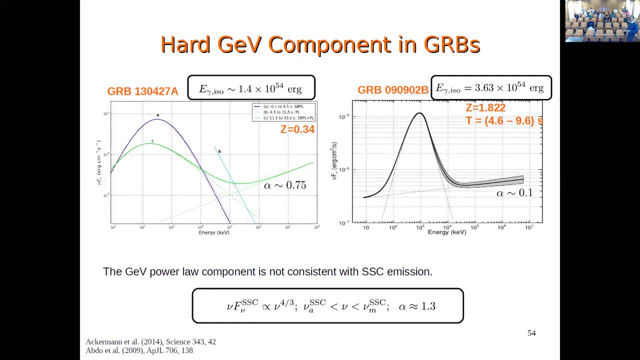 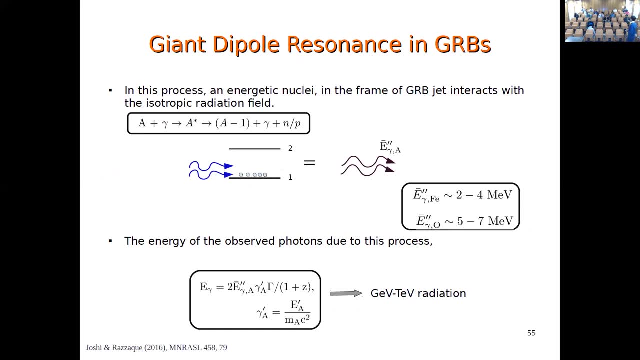 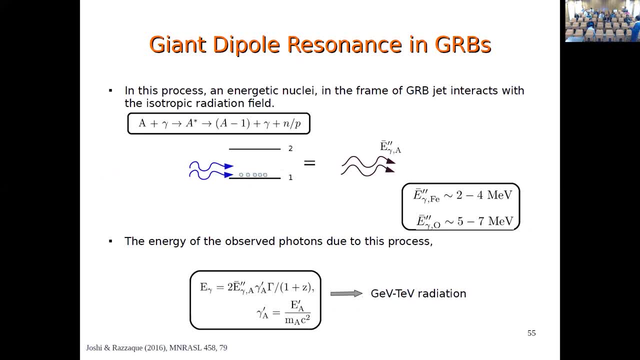 Because it is the most abundant source. Okay, So why iron and not others? Because it is the most abundant source. Okay, Because it is the most abundant source. Next two slides: Okay, So, yeah, Okay, Did you have. 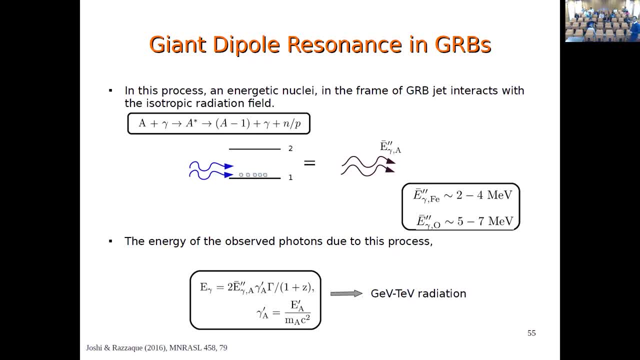 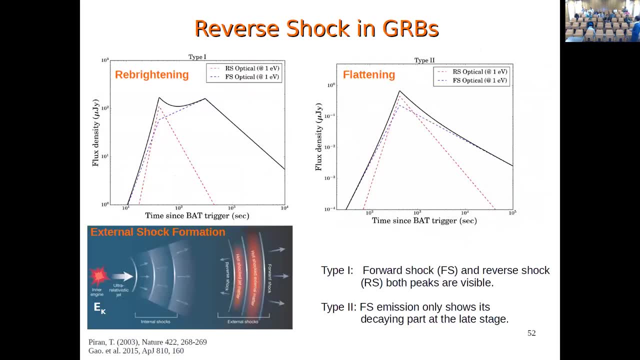 I have two questions regarding the reverse shock. one: Yes, So just go to the Yes. So here you have. So here you have Two things: One is re-brightning, Second is flattening. Yes, Okay. 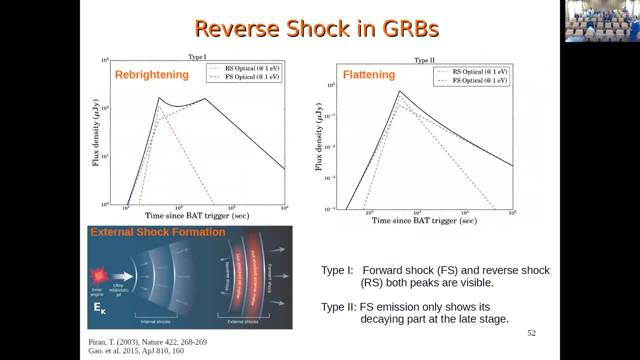 So flattening is the late time flattening, or it is how much time you want to flatten, Which is the. So here you have, You have to, You have to, You have to go, You have to go, You have to go. 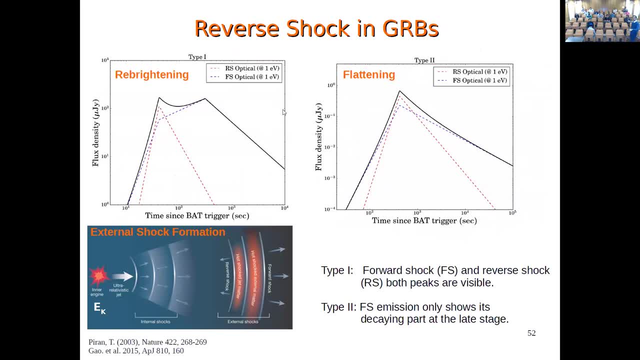 it is how much after how much time, which is 10 to the 4th second. so the contrast you see in these two cases you have the reverse shock peak and a forward. first you get the reverse shock emission. because of that you get some decay kind of thing. then after that the forward. 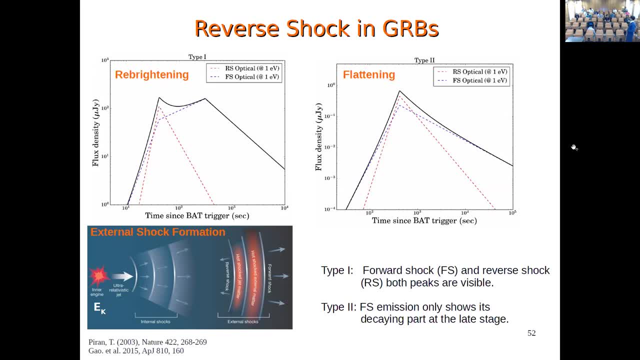 shock is dominant. yes, so that's the, and i i am studying somewhere that this late time flattening thing it is also coming because of the scintillation effect. okay, that's something i want to learn. so, whenever the grb emission coming near the, near our galaxy or near any galaxy there is, 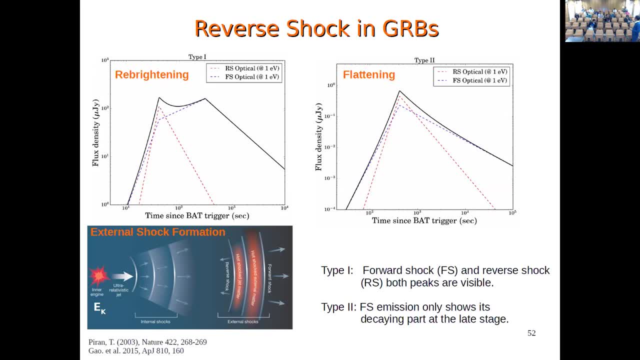 some scintillation effect and because of that the light curve is almost getting a plateau kind of thing, even in optical, yeah, even in the optical and in the radio. okay, very simple, and i'm aware, yeah, in radio it is dominated, but in that, yeah, but in optical also, not not very early. 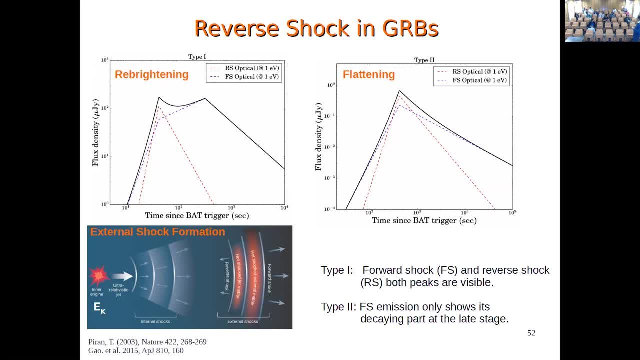 yeah, it is very hard. yeah, you know the exploration and radio rs is dominating up to very late time, so that's the possibility. optical it will be very early, very early. yes, so scintillation and optical, yeah, yeah, yeah, so i understand that. okay, okay, okay okay. 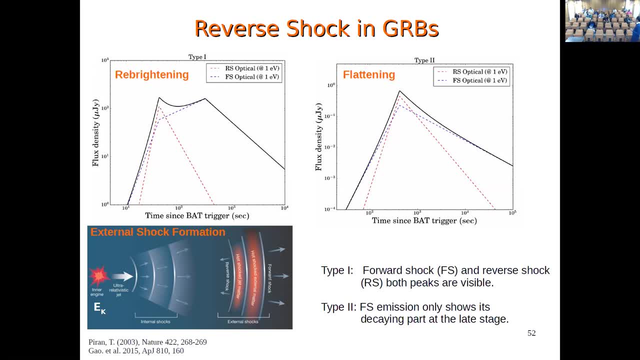 okay, okay, okay. so you pointed out some uh in one of the slides that was showing this uh, bottom left plot that external shock become effective in the blast wave. i mean later, later phase. why don't you see in the beginning external shock? because the flow is highly relativistic anyway you. 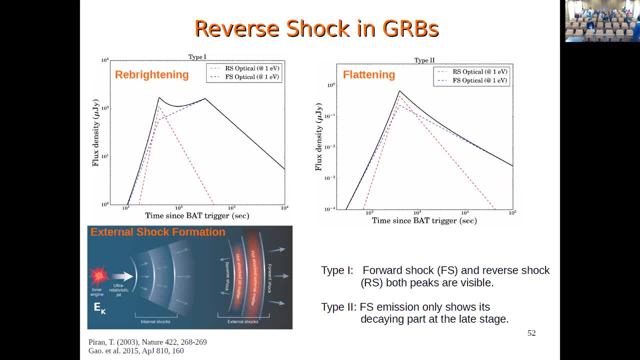 know? yeah, but it's a radiation fixture. yeah, you pointed out, everything depends on the dsd. oh, now that's it, and then ds lesson happens and the ds lesson. basically, you put the input parameter and the ds lesson time can become, like you know, one second, 10 to the power minus one second. there are cases. 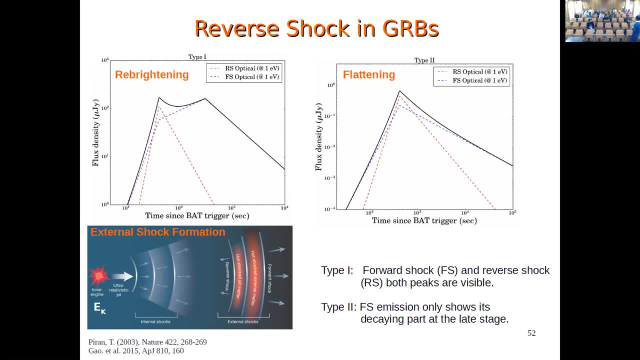 after you can start before prompt. okay, so in that case, how it happens, there are, like, like you know, papers about that, so it depends on the ds lesson time when it happens, so you can have only time, like you know, at least 13 over 27a. you have this complete model of rsn forward shock. you can. 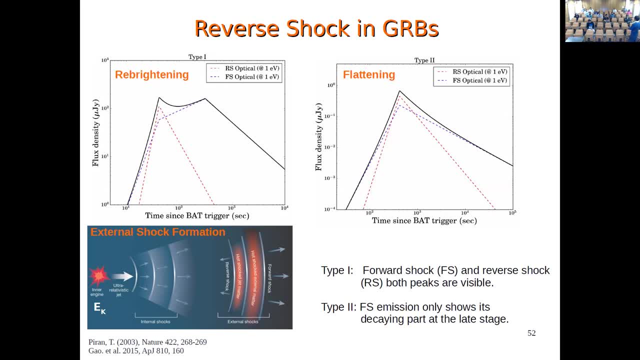 explain the instance from one second: first your shock and then the the product shock. so it depends on the ds lesson process is very quick. i mean the time taken from the originating case of the shock up to the external shock and we are just immune. it's a very short-lived process. yes, it's good. 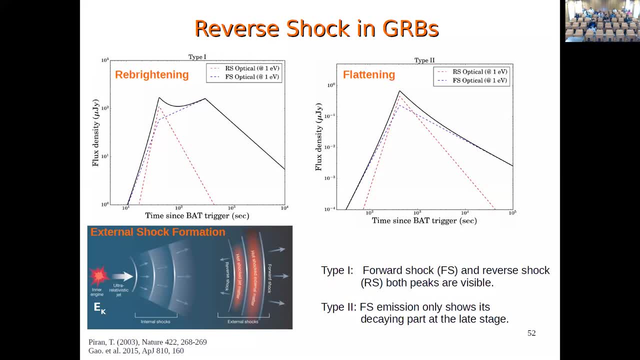 to write the time time. yeah, i was thinking like you know the plots. they show, like that, our synonyms. oh, you are saying the reversal time in the bottom. oh, yeah, definitely, yeah, so, yeah, definitely, this is around and you are 13 to the 14 centimeter radius. 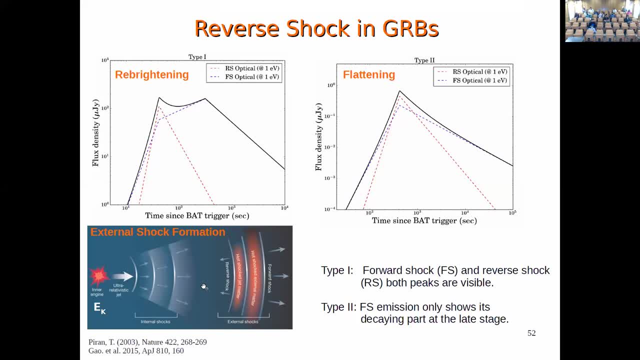 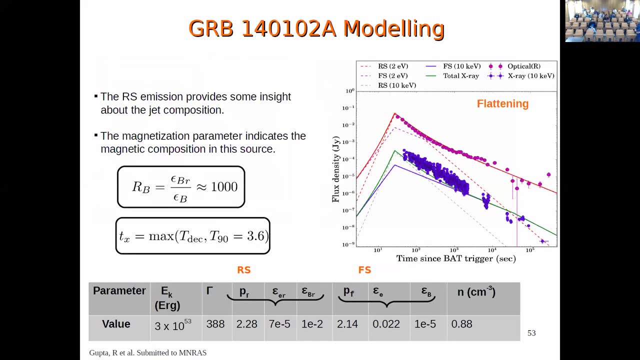 and this is then you are 16 to 17 centimeters. here you have considered the thick and thin cell. yeah, so this is important again, like pin and thick cell, like you know. so so how you define a thin cell is the maximum of ds lesson and t90- okay, that is the peak emission here. 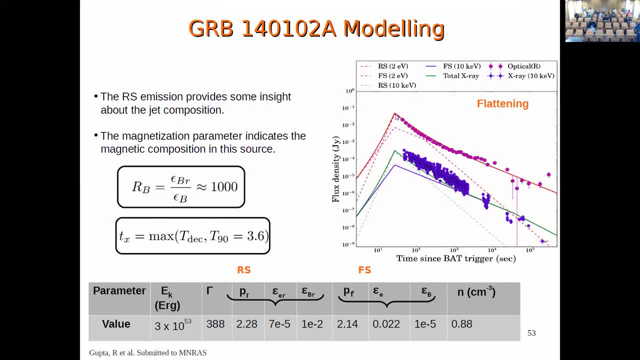 and when, at least you see the ds lesson time. so the tx is this and tx takes a value, something around 15 or something. so basically tds lesson is greater than t90 and this is called thin cell. consider a case: thick cell. okay, what would happen? so it will reverse, basically. 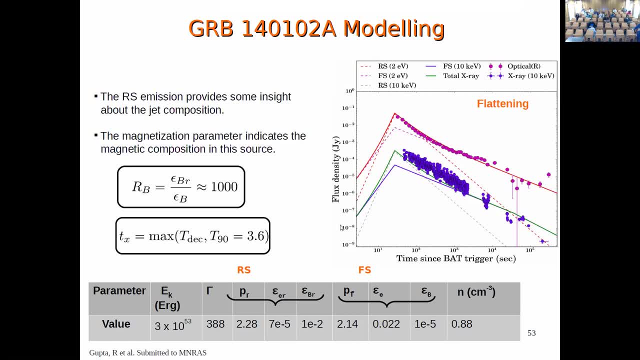 so then tx will become 3.6. so the emission has to be somewhere here. can we detect something like that? one second, two seconds of your shock signatures? so like suppose there is a pixel case. so pixel case, the tx will become 3.6. so then, 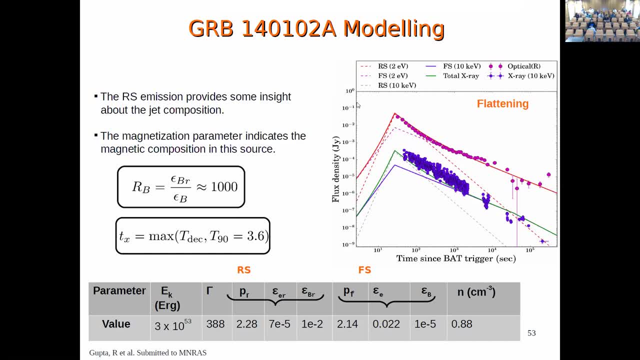 the peak will sit, like if there is a thick cell, then we should see emission only in time, something like that. so maybe asking for getting 3.6 from the value of 3.65 in the case of thick cell, whenever the shock crosses the cell, yeah, it becomes the relativistic. 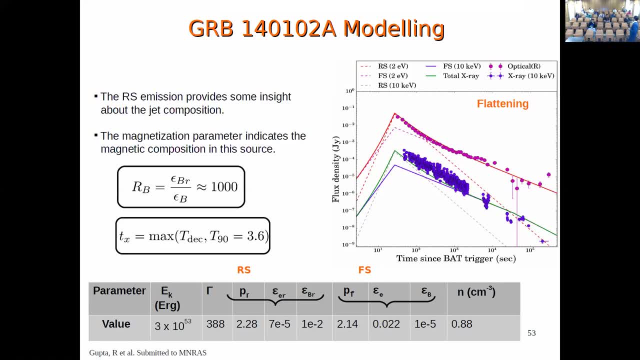 so this is why you can get some early time emission for the thick cell, but for the thin cell you can expect some newtonian kind of means. this is not related. is later? yes, correct, yeah, yeah, so this is one of the basic set of equations that you start with when you see your data, like the initial equation.